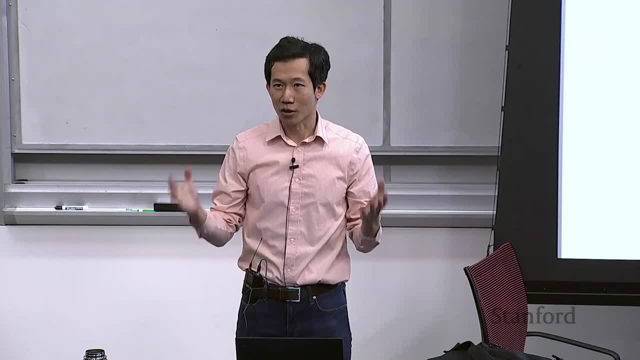 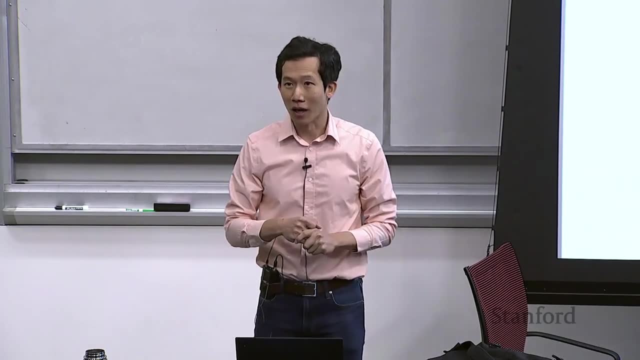 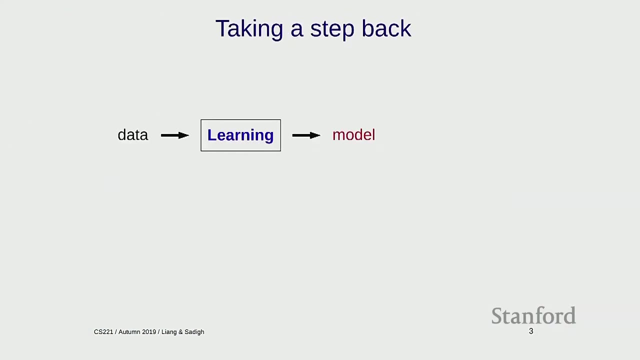 on next Monday's lecture how you can do logical inference to arrive at answers much faster than you might have otherwise. So we've arrived at the end of the uh, the class um, and I want to just reflect a little bit on what we've learned. 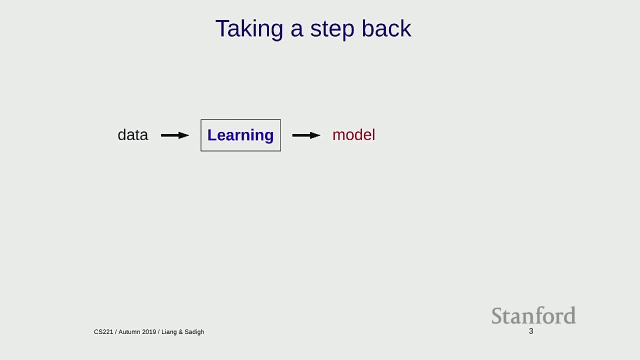 and maybe this will be also a good review for the exam. Um, so in this class we've bolst- bolsted everything on the modeling inference learning paradigm, And the picture you should have in your head is this, Abstractly, we take some data. 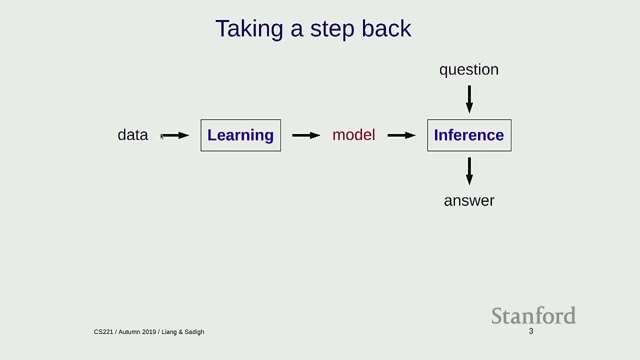 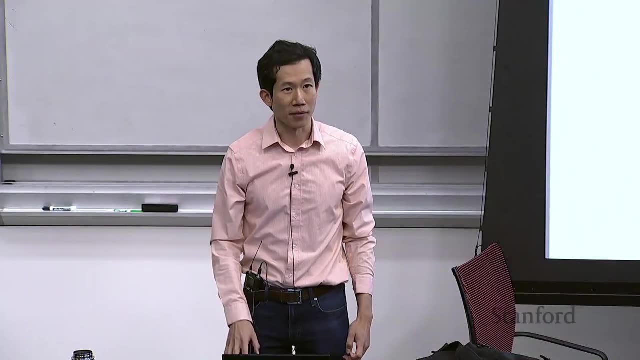 we perform some learning on it and we produce a model And using that model, we can produce- perform inference, which looks like taking in a question and returning an answer. So what does this look like for all the different types of instantiations we've looked at? 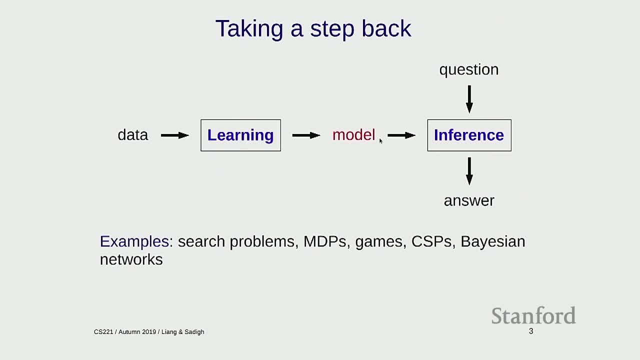 So for search problems, the model is: a- is a search problem and the inference asks the question: what is the minimum cost path Um in MDPs and games? we ask the question. what is the maximum value policy In CSPs? we ask the question. 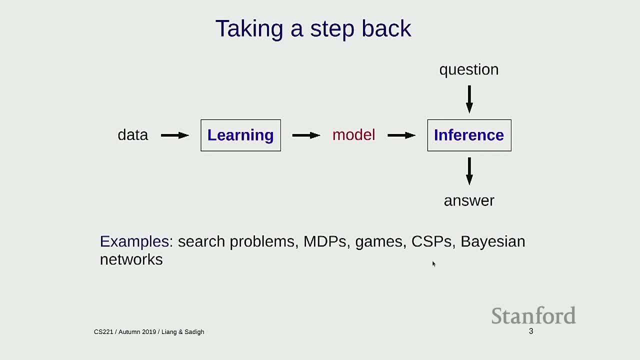 what is the maximum weight, ass- assignment? And in Bayesian networks we can answer probabilistic inference queries of the form: what is the probability of some query variables condition on some evidence variables? And for each of these case we looked at the modeling. 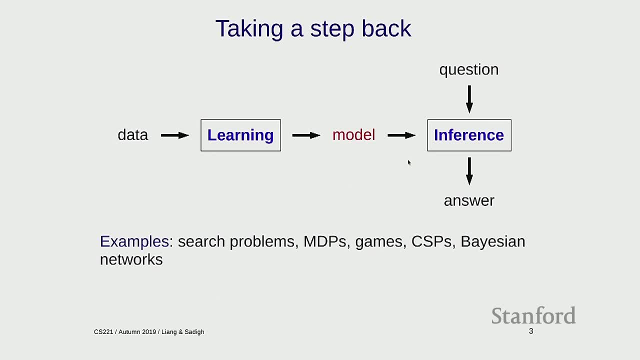 we looked at the- the inference algorithms, and then we looked at different types of uh learning procedures going backwards, maximum likelihood Uh. we looked at uh various reinforcement learning algorithms. we looked at structured perceptron and so on. 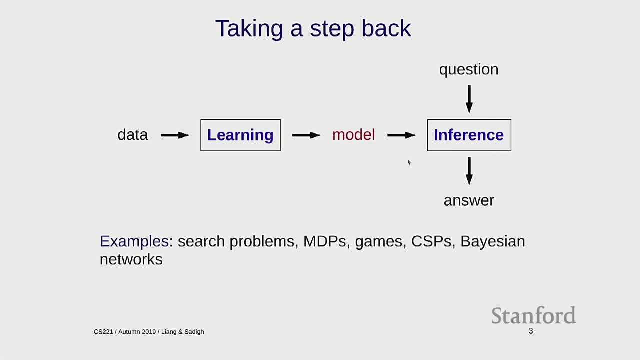 And hopefully this- this kind of sums up, um, the kind of the worldview that CS31 is trying to impart is that there are these different, you know, components, um, and depending on what kind of modeling you choose, you have different types of algorithms. 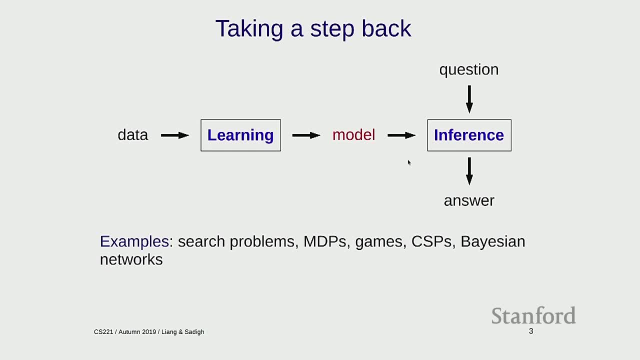 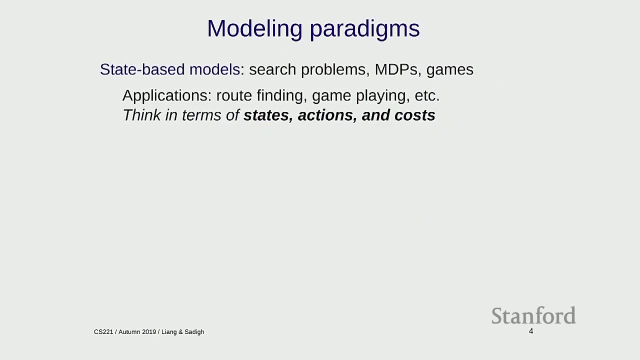 um and learning algorithms, inference algorithms and learning algorithms that emerge. Okay. So we looked at several modeling paradigms um, roughly broken into three categories. The first is state-based models, search problems, MDPs and games. 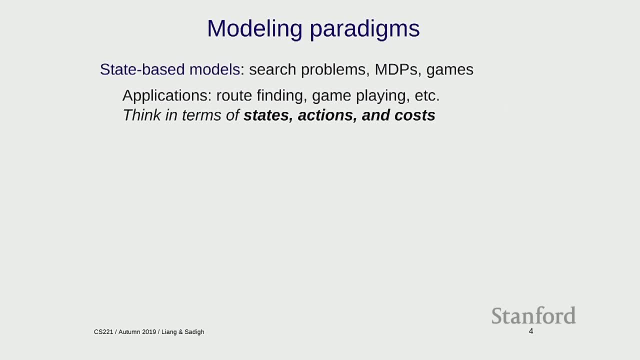 And here um the-, the way you think about modeling is in terms of states and as nodes in a graph and actions that take you between different states, um which incur either a cost or give you some sort of reward, And your goal is just to find paths, or 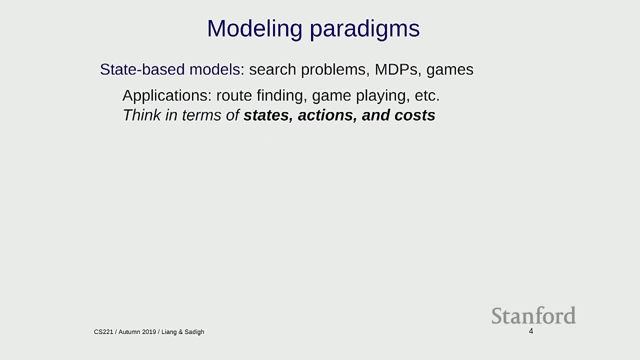 uh contingent paths or policies, um, in these graphs. Then we shifted gears to talk about variable-based models, where instead we think about variables, um, and factors that constrain, or um these variables to uh take on certain types of values. 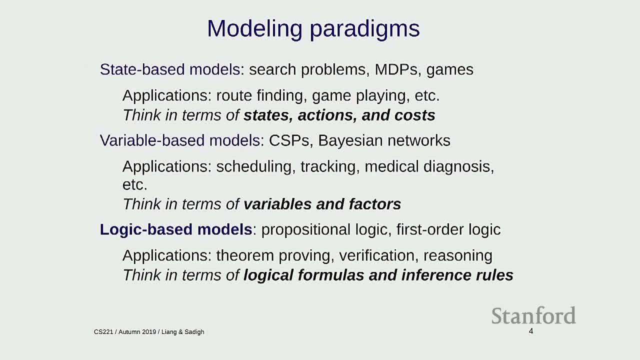 Um. so in today's lecture, I'm gonna talk about logical-based models. So we're gonna look at propositional logic and first-order logic, which are two different types of logical languages, or uh, models. And um, we're gonna instead think about logical formulas and inference rules. 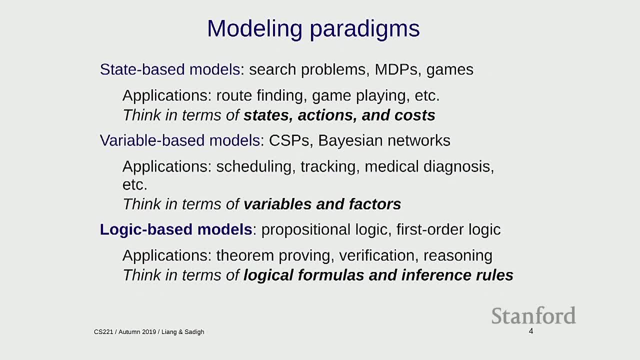 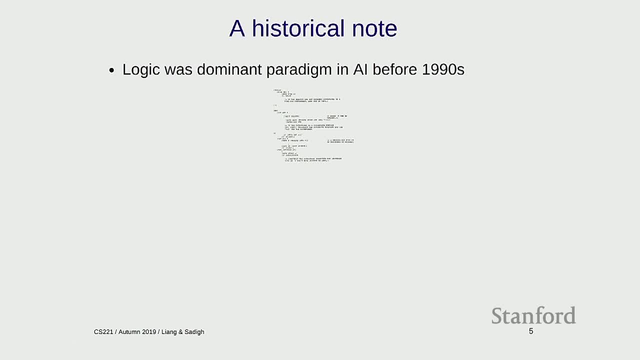 which is going to be another way of kind of thinking about, uh, modeling the world. Historically, logic was actually the dominant paradigm in AI um before the 1990s, So it might be hard to kind of believe now. 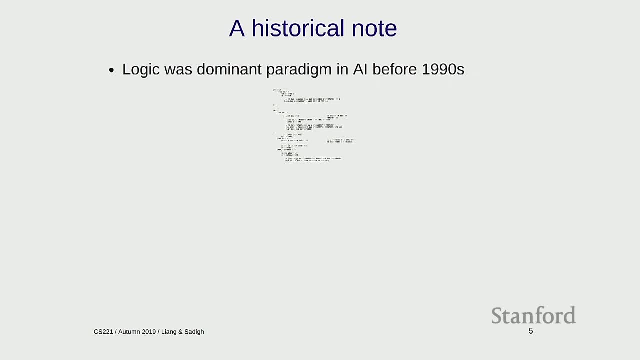 but just imagine the amount of excitement that is going into deep learning today. This equal amount, uh, of excitement was going into logical-based methods in- in AI, in uh um in the 80s, and before that too, Um, but there was kind of two problems with logic. 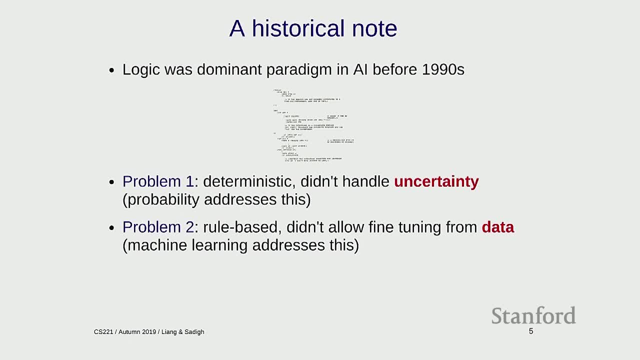 One is that um logic was deterministic, so it didn't handle uncertainty very well, And that's why probabilistic inference and other methods were developed to address this. And it was also rule-based, which allow- didn't allow- you to naturally ingest a large amount of data to 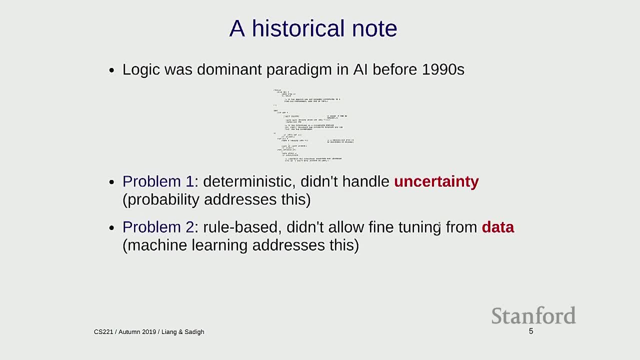 you know, uh, guide behavior And the emergence of machine learning has addressed this, Um, but one strength that kind of has been left on the table is the expressiveness, And I kind of emphasize, uh, that logic, as you will see, 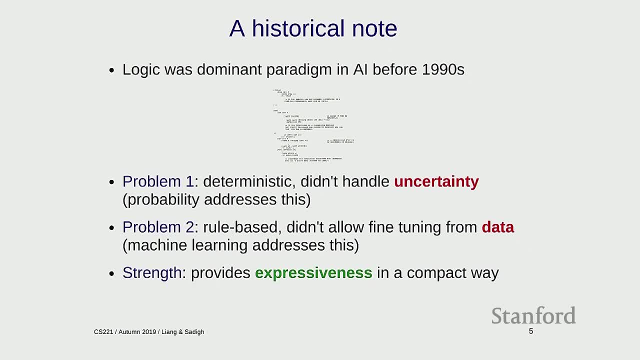 gives you, um the ability to express very complicated things in a very, you know, succinct way. And that is kind of the main point of uh logic which I really want everyone to um kind of appreciate, And hopefully this will become clear through examples. 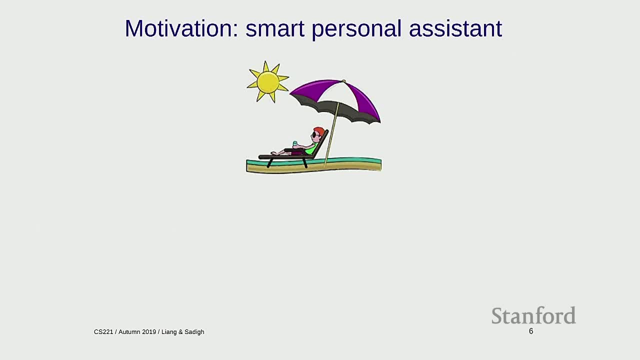 Um, as I motivate on the first day of class, the reason, uh, one- one good way to think about why we might want, uh, logic is: imagine you want to lie on a beach, um, and you want your assistant to be able to do things for you. 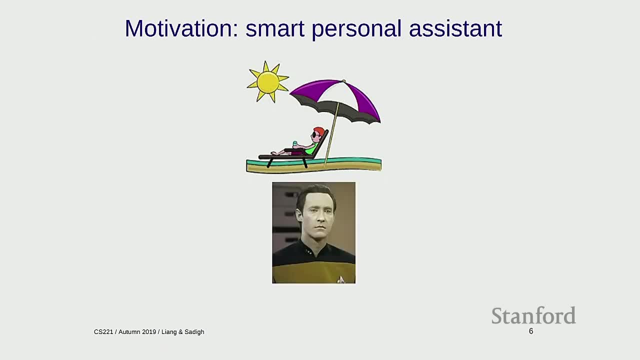 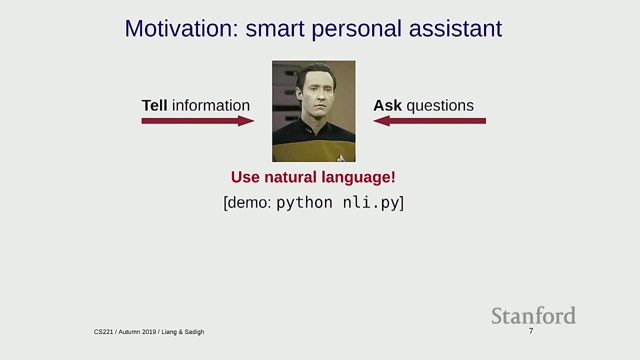 But, um, hopefully it's more like um data from Star Trek rather than Siri. Um you want to take an assistant. you want to be able to at least tell information and ask your questions and have um these questions actually be answered in response to reflect the information that you've uh told him. 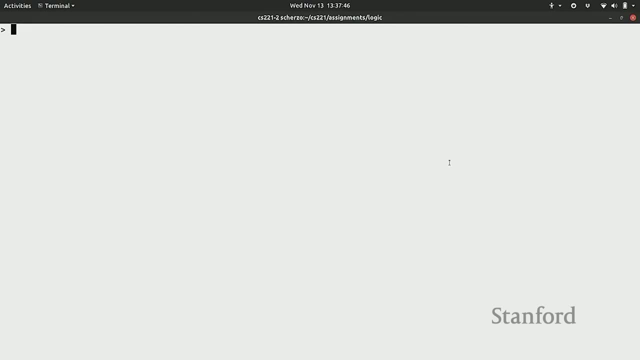 Um. so just kind of a brief refresher. On the first day of class I showed you this demo where you can talk to the system, um, um, and say things and ask questions. So a small example is, um, let's say, all students like, uh, CS 221. 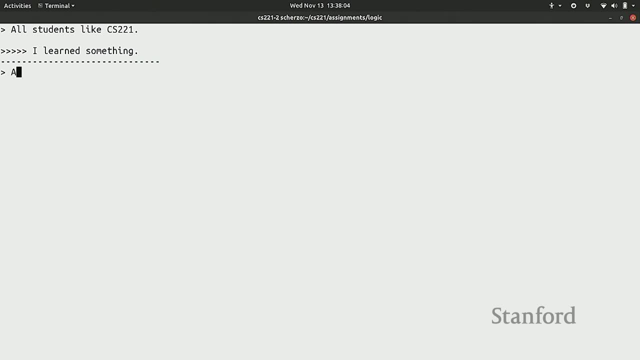 It's great, It teaches important things. Um and uh, Alice does not like CS 221.. And then you can ask: um you know, is Alice a student? And the answer should be no, because it can kind of reason about this. 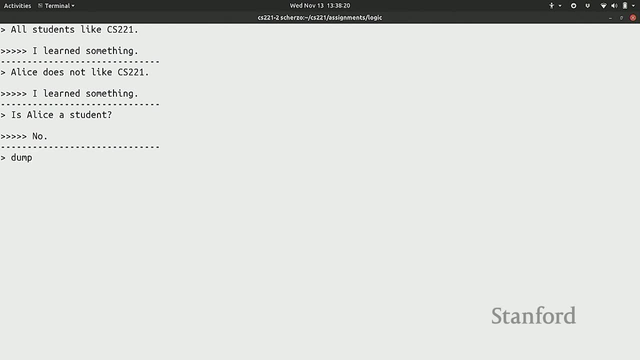 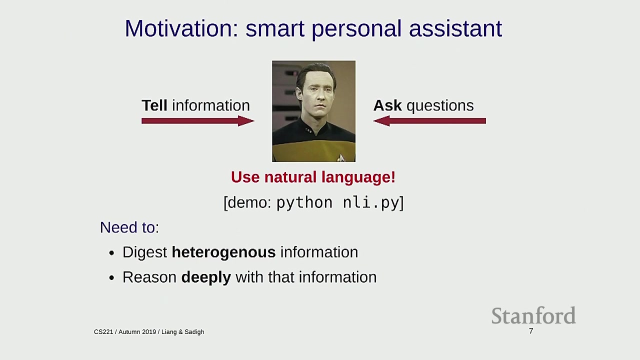 Um, and just to dive under the hood a little bit: um, inside it has some sort of knowledge base that contains the information that, um, it has. We'll come back to this in a second. Okay, Um, so this- this assistant needs to be able to digest. 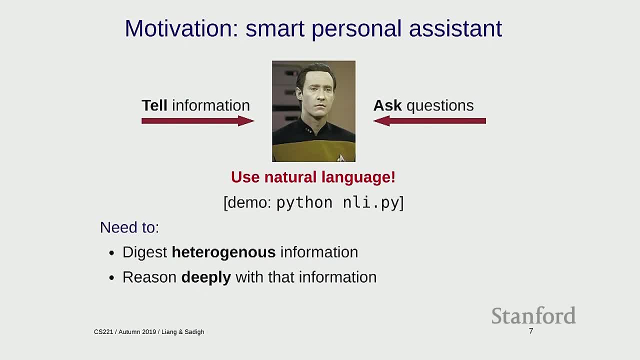 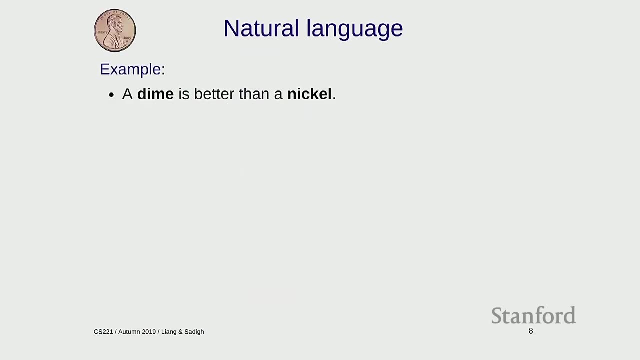 heterogeneous information in the form of natural language. you know uh utterances, and it has to reason deeply with that information. So it can't just do. you know superficial pattern matching. So I've kind of suggested natural language as an interface to this. 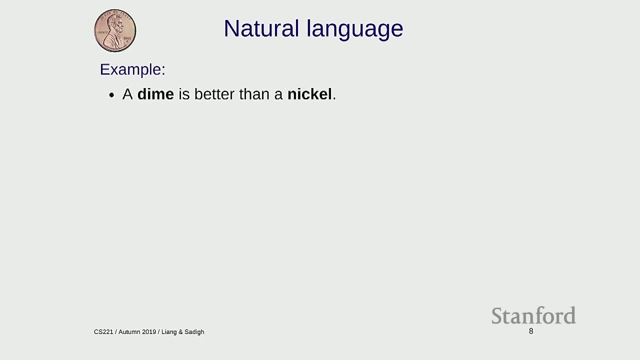 Um, and natural language is very powerful because, um, I can stand up here and use natural language to give a lecture and hopefully you guys can understand at least some of it. Um and-. but you know, let's- let's go with natural language for now. 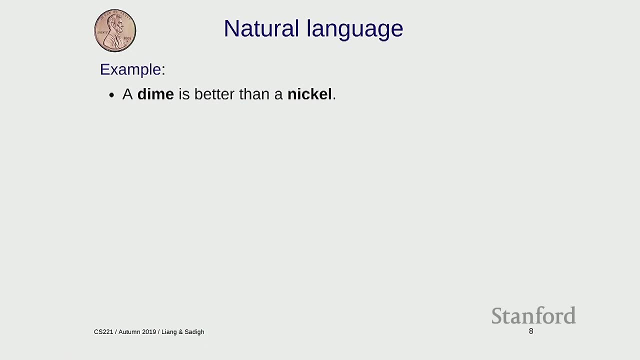 So here- here's an example of how you can draw inferences using natural language. Okay, So a dime is better than a nickel. Um, a nickel is better than a penny. So therefore, a dime is better than a penny. Okay, So this seems like pretty sound reasoning. 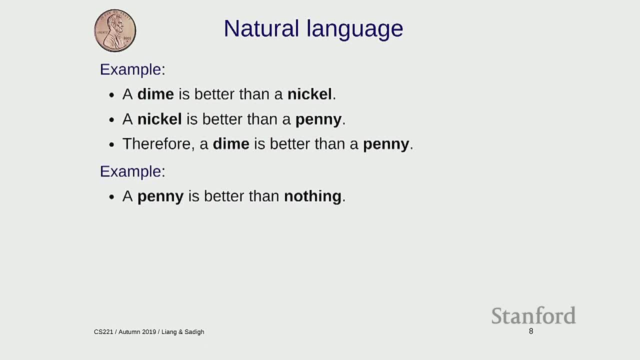 Um, so what about this example? A penny is better than nothing. Um, nothing is better than world peace. Um, therefore, a penny is better than world peace, right, Okay? So something clearly went uh wrong here, and this is because 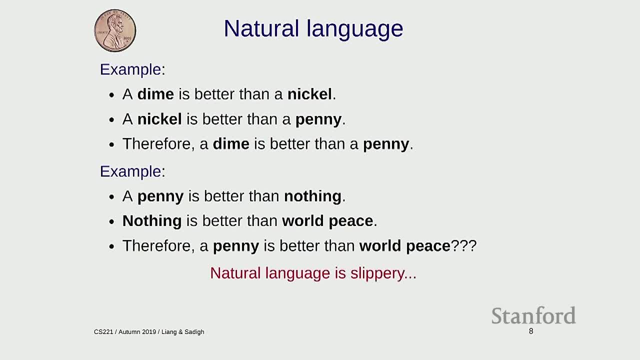 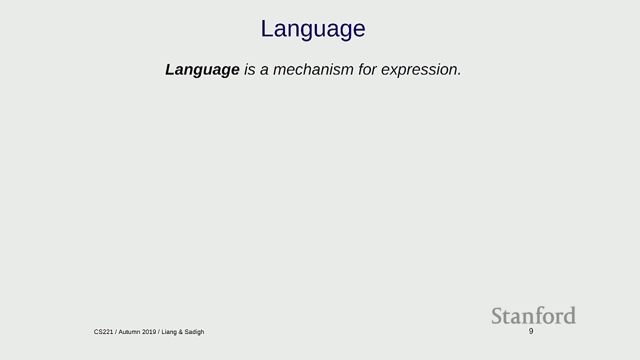 language is- natural language is kind of slippery, It's not very precise, which makes it very easy to kind of make these, um, these mistakes, Um. but if we step back and think about what is the role of natural language, it's really language itself is an ex- mechanism for expression. 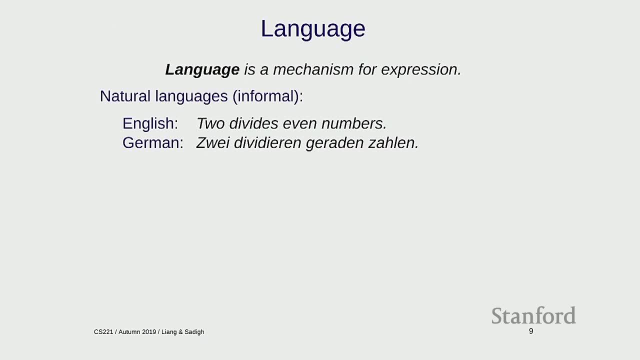 So there are many types of languages. There's natural languages, um. there's programming languages, which all of you are, you know, familiar with um. but we're gonna talk about a different type of language, called logical languages, Um, like programming languages, 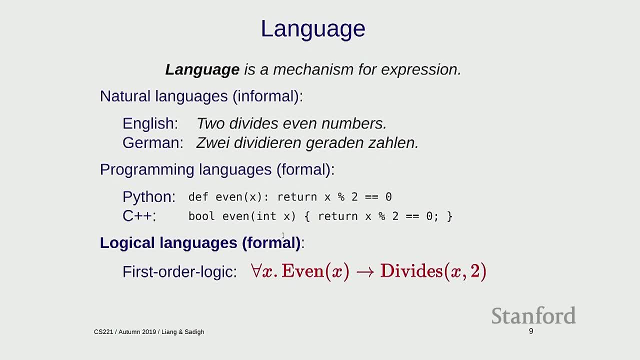 they're gonna be formal, So we're gonna be absolutely clear what we mean by when we have a statement in a logical language- Um, but- and like natural language, it's going to be um, declarative, Um, and this is- might be a little bit harder to appreciate right now. 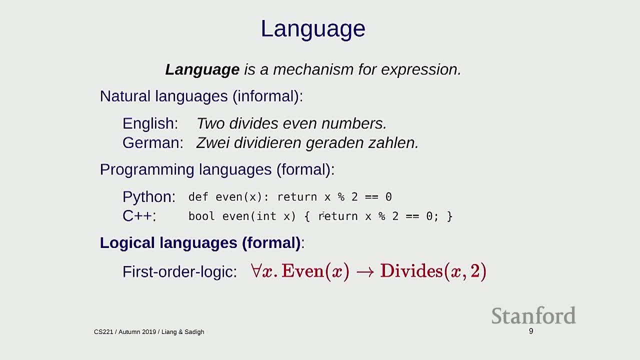 but it means that, uh, there's kind of a more of a um one-to-one isomorphism between um languages, One-to-one isomorphism between logical languages and natural languages, as it compared to um programming languages and natural language. 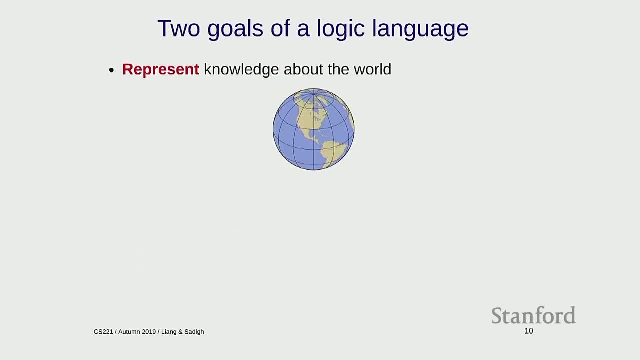 Okay, Um, so in a logical language, we want to have two uh properties. First, the logical language should be uh rich enough to represent knowledge about the world, Um, and secondly, it's not sufficient just to represent the knowledge, because, 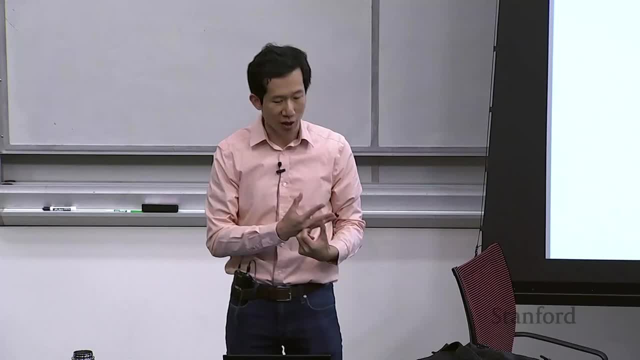 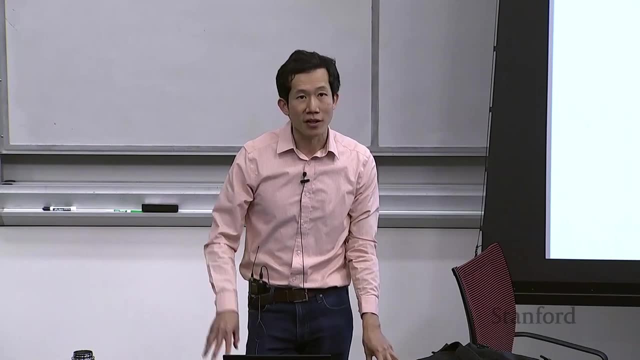 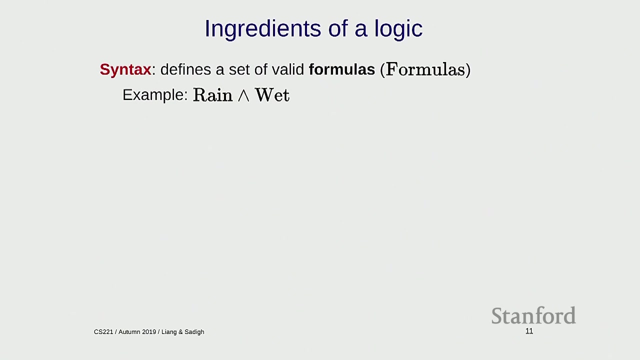 you know, a hard drive can represent the knowledge, but you have to be able to use that knowledge in a- in a way to reason with it. Um, a logic contains three uh ingredients, um which I'll um go through it in a- in subsequent slides. 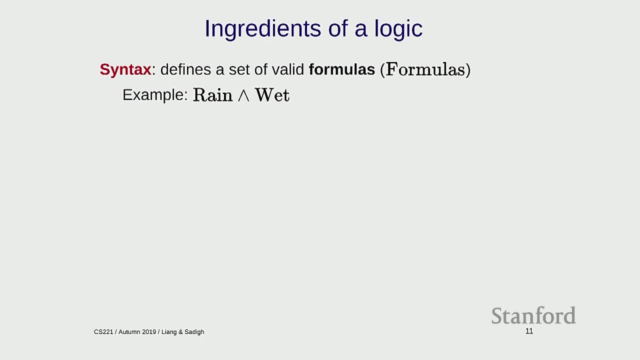 There's a syntax which defines um what kind of expressions are valid or grammatical in this language. Um there's semantics, which is for each um expression or formula, what does it mean? And mean means- is actually mean something very precise. 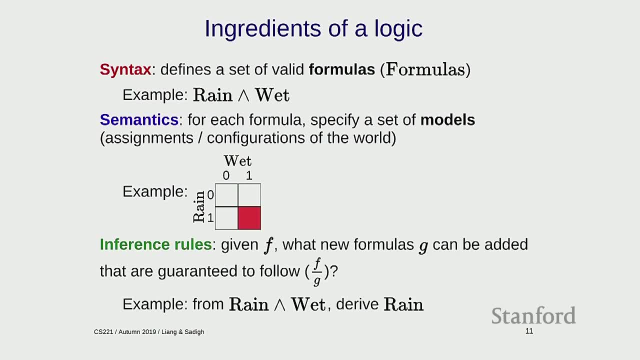 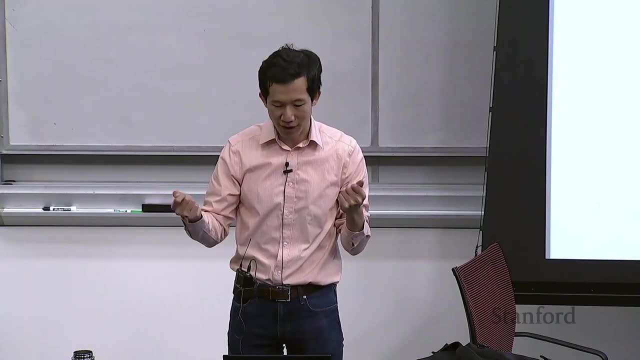 which I'll you know come back to. And then inference rules allow you to take various formulas and do kind of operations on them, Just like in the beginning we- when we have the algebra problem. you can add equations, you can move things to different sides. 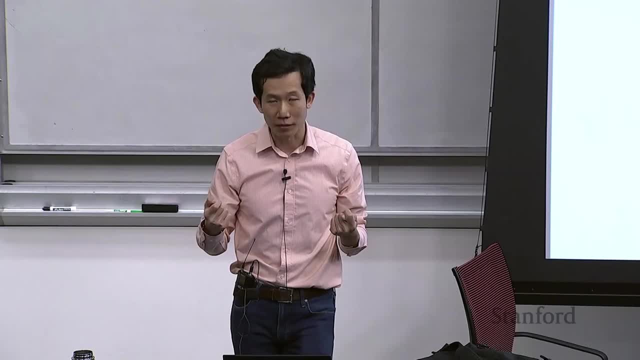 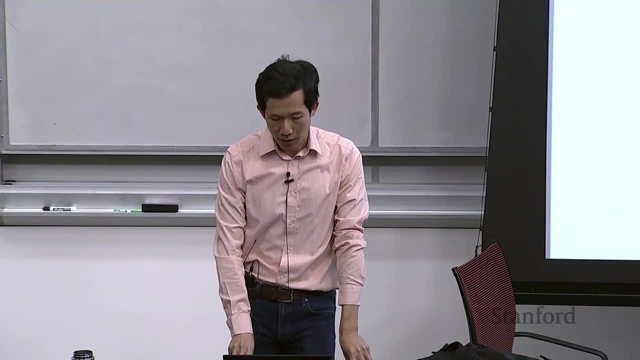 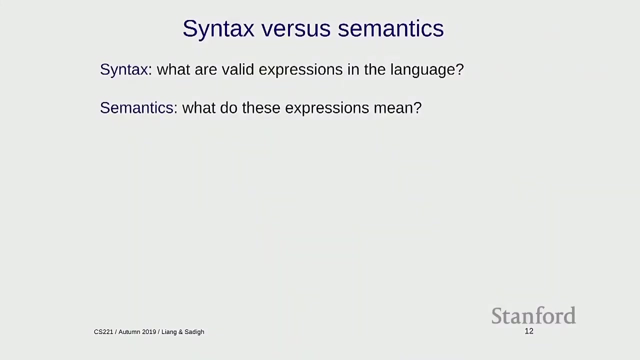 You can perform these rules, which are syntactic manipulations, on these formulas or expressions that preserve some sort of semantics. Okay, So just to talk about syntax versus semantics a little bit, because I think this might be a slightly subtle point which hopefully will be clear with this example. 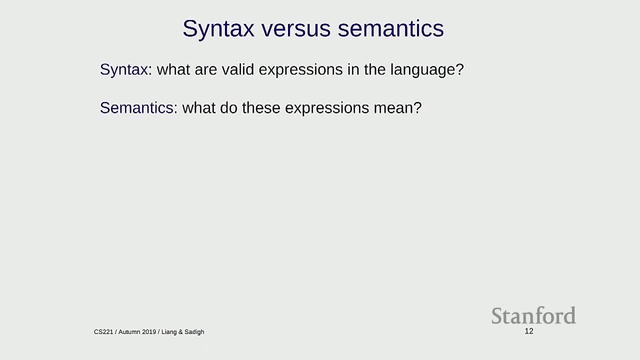 So syntax refers to what are the valid expressions in this language, And semantics is about what these expressions mean. So here's an example of two expressions which have different syntax: 2 plus 3 is not the same thing as 3 plus 2,. 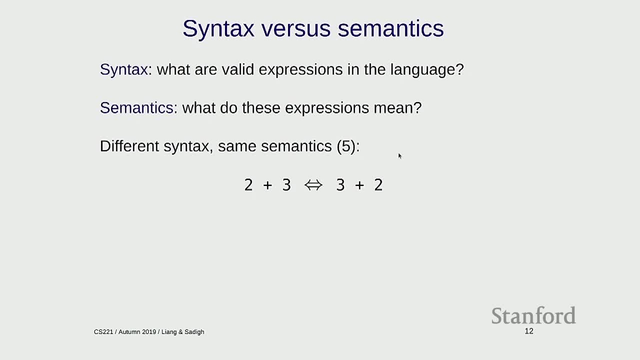 but they have the same semantics. Both of them mean the number you know, 5.. Here's a case where we have two expressions with the same syntax- 3 divided by 2, but they have different semantics, be- depending on which language you're in. 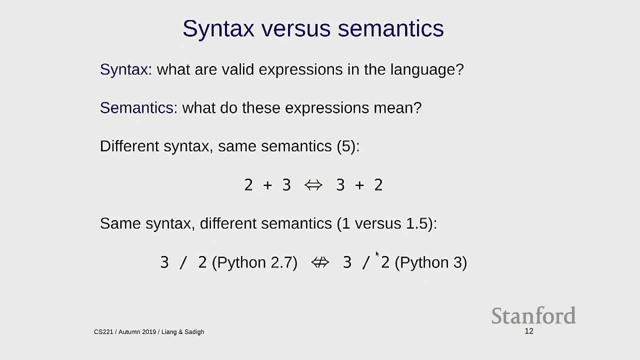 Okay, So in order to define a language precisely, you not only have to specify the syntax, but also the um, the semantics, because just by looking at the syntax, you don't actually know what its meaning is, unless I tell you. 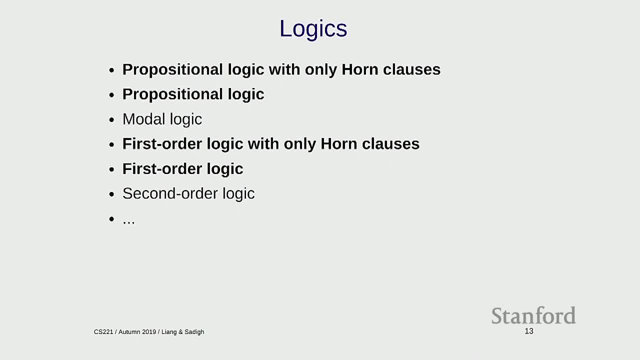 Um, there's a bunch of different logics. Um, the ones highlighted in bold are the ones I'm gonna actually talk about in this class. So today's lecture is going to be um on propositional logic. Um and then uh. 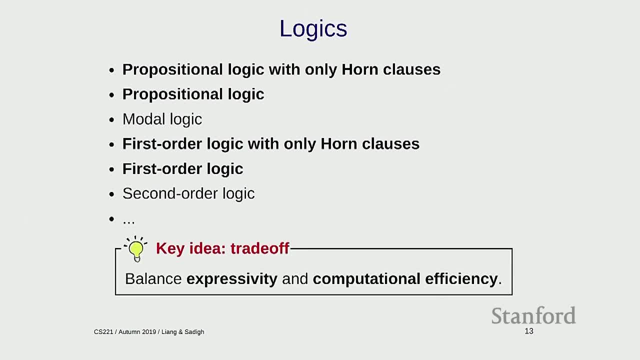 in the next lecture I'm gonna look at first order logic. Um, as with most models in general, there's going to be a trade-off between the expressivity and the computational efficiency. So as I go down this list to first order logic and beyond, 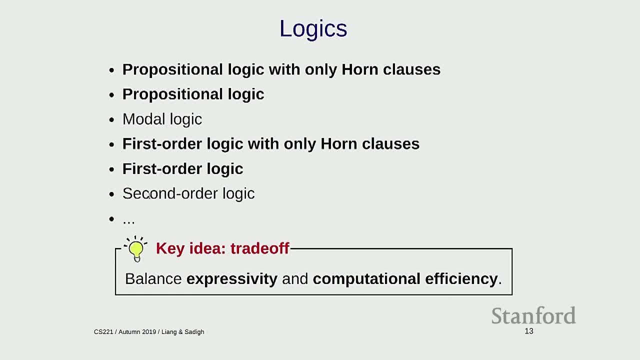 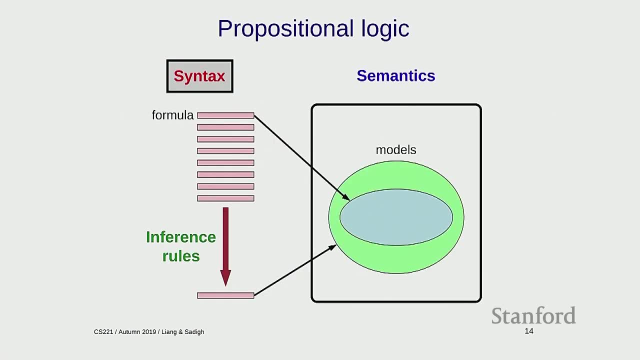 um, I'm going to be able to express more and more things using the language, but it's going to be harder to do, uh, computation in that language. Okay, So this is the- the kind of a key diagram, um, to have in your head while I go through. 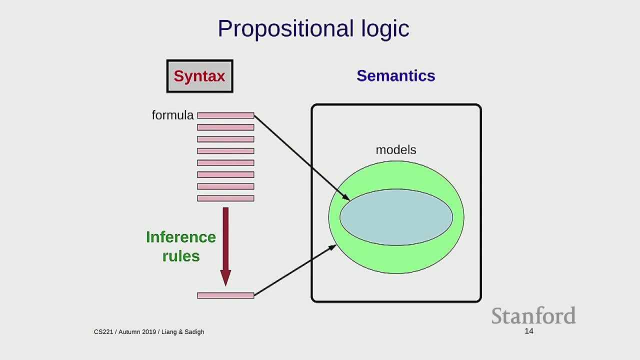 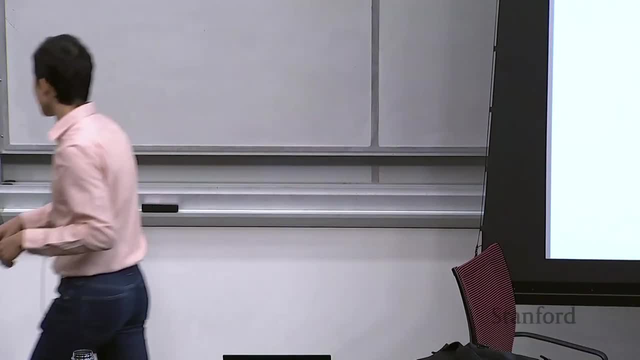 syntax, semantics and inference rules. So for every- I'm gonna do this for propositional logic and then in uh Monday's lecture I'm gonna do it for uh first order logic. Um, so, just to get this on the board. 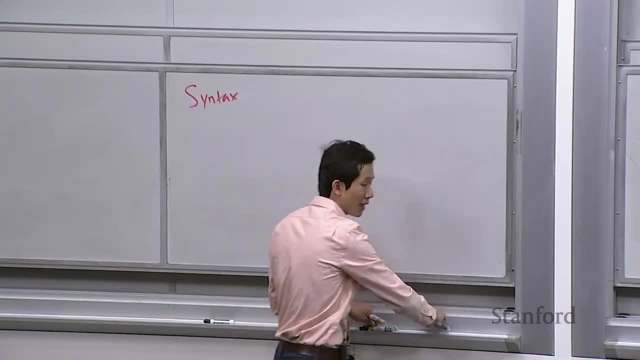 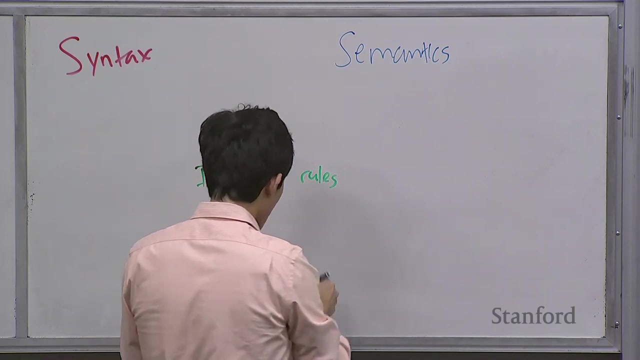 um, we have syntax, we have um semantics, and then we have inference rules. Um, let's just write it there. Um so? so this lecture is going to have a lot of definitions and concepts. um, in the- just to give you a warning. 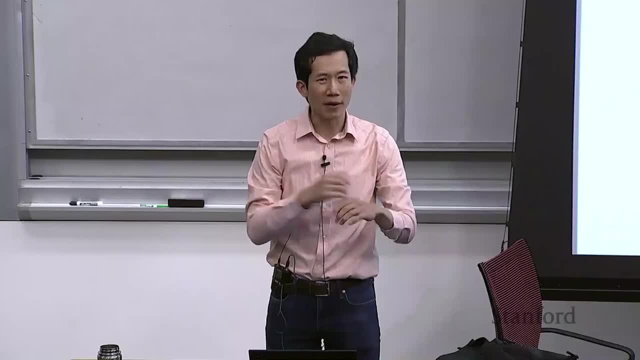 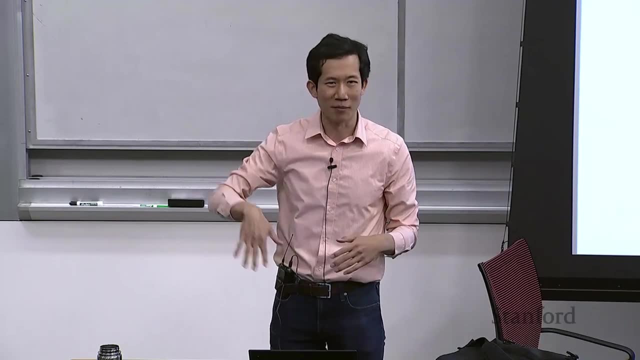 There's a lot of kind of ideas here, Um, they're all very kind of uh, um simple by themselves and they kind of piece together. but there's just gonna kind of be a barrage of uh terms and I'll try to write them on the board so that you can kind of remember them. 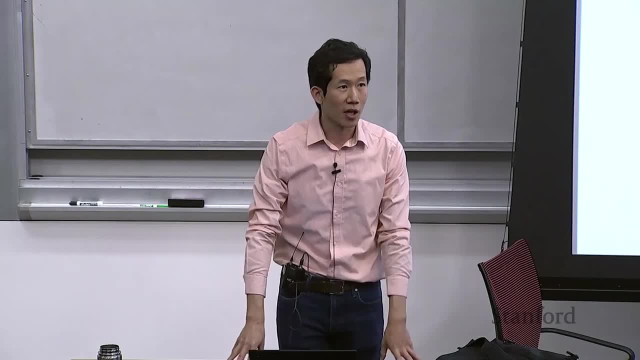 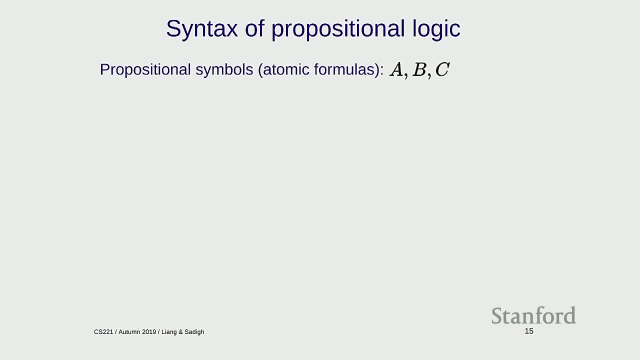 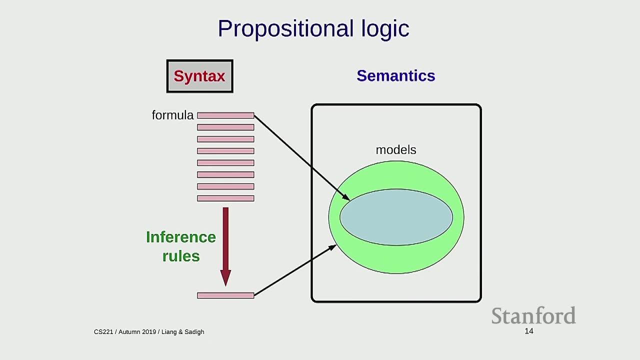 I need to specify um. I need to specify um. I need to specify um. I need to specify what are the formulas Um, um. so one maybe other comment about logic is that um. some of you have probably taken. 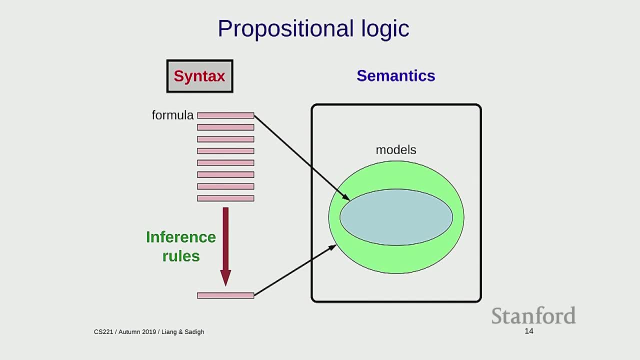 um CS103 or an equivalent class, where you've been exposed to propositional logic. Um, what I'm gonna do here is kind of a much more methodological, uh, and kind of rigorous treatment of it. Um, the- I want to distinguish the difference between: 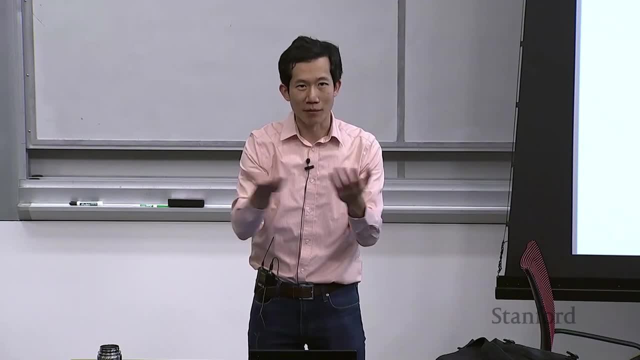 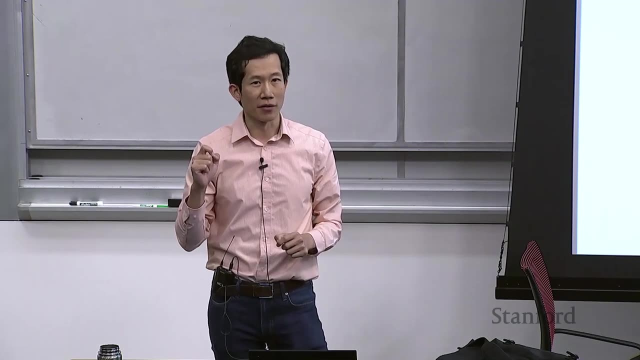 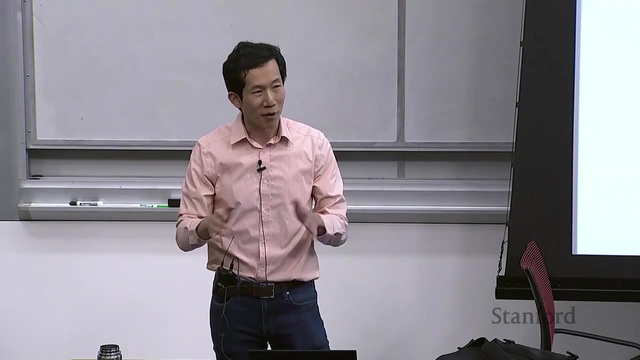 uh, being able to do logic yourself, Like if I gave you some uh logical expression, you can manipulate it. That's different than, um, talking about a general set of algorithms that can operate on logic itself, right? So remember, in AI. 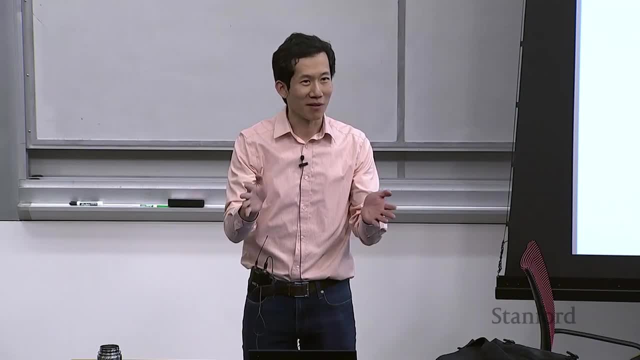 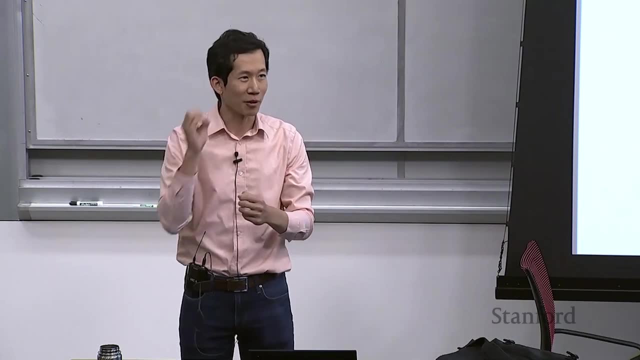 we're not interested in you guys doing logic, because that's just I, that's intelligence, Um. but we're interested in developing general principles or general algorithms that can actually do the work. uh, for you, okay, Just like in, uh, in the Bayesian networks. 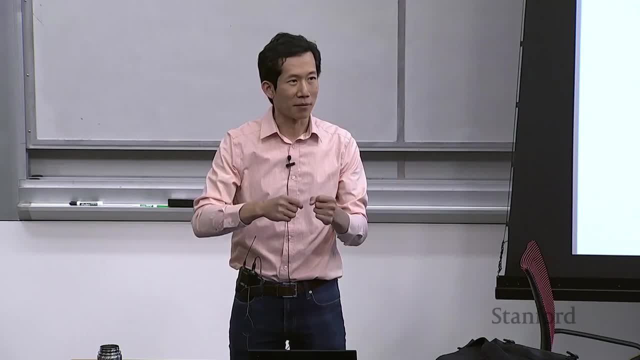 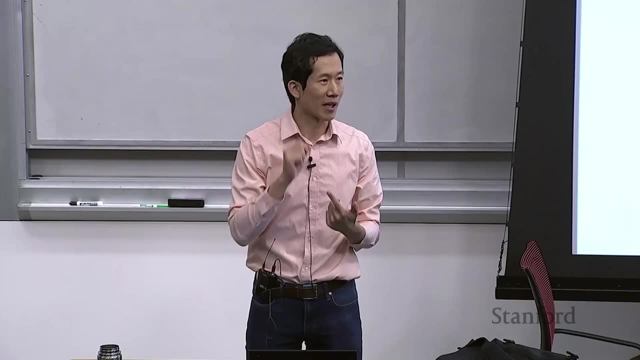 it's very fine- well that you can- you guys can uh manipulate and condi- uh calculate conditional and marginal probabilities yourself. But the whole point is we devise algorithms like Gibbs, sampling and variable elimination that can work on any um Bayesian network. 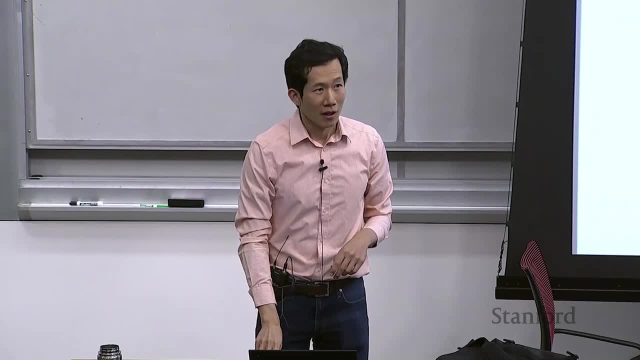 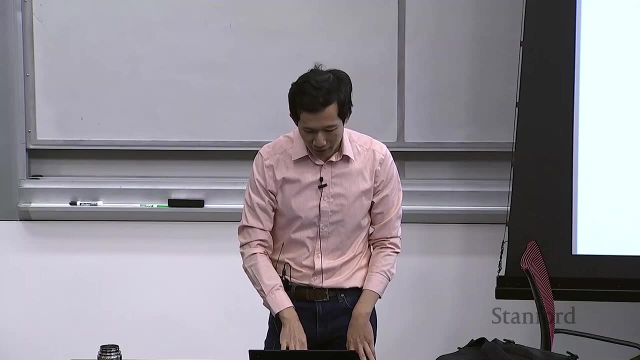 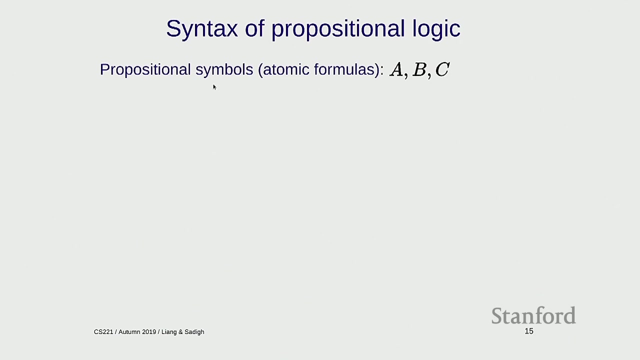 Just wanna get that out there, Okay. So let's uh begin. Um, this is gonna be building from the ground up. So, first of all, there are- in propositional logic, there are a set of propositional symbols. 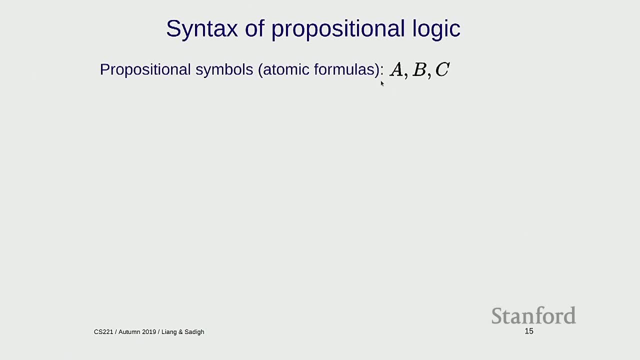 These are typically gonna be uppercase letters or even um, words, Um, and these are the atomic formulas: Um. these are formulas that can't be any smaller. There's going to be logical connectives such as uh, not and or, um implication and bidirectional implication. 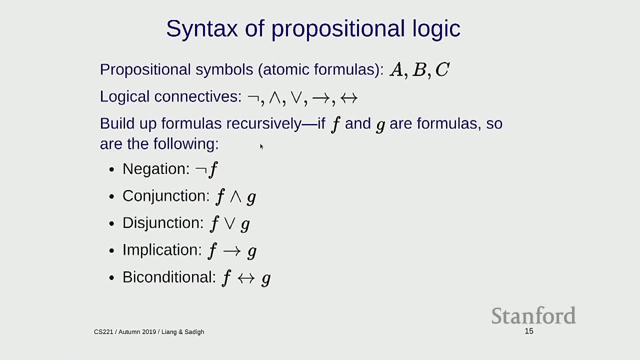 And then the set of formulas are built up recursively. So if f and g are formulas, then I can- these are also formulas. I can have not f. I can have f and g, f or g. f implies g and f. um. bidirectional implication: g or equivalent to g. 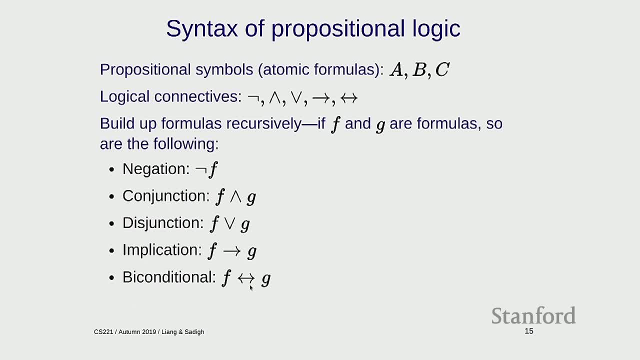 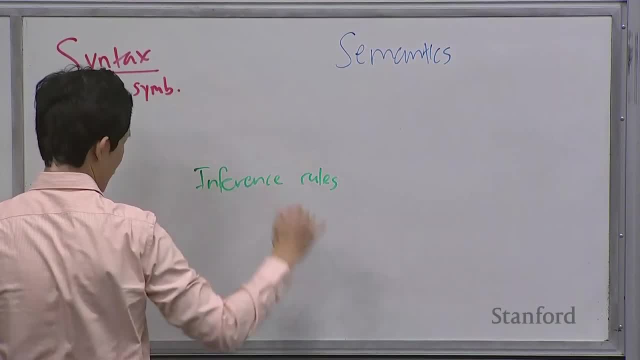 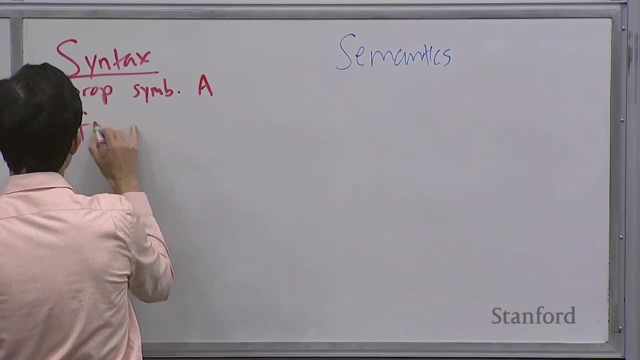 Okay, So the key, um, you know, ideas here are. we have um propositional symbols. Um, I'm gonna move, move this down, since I'm gonna run out of space. Um, so this- these are things like a. 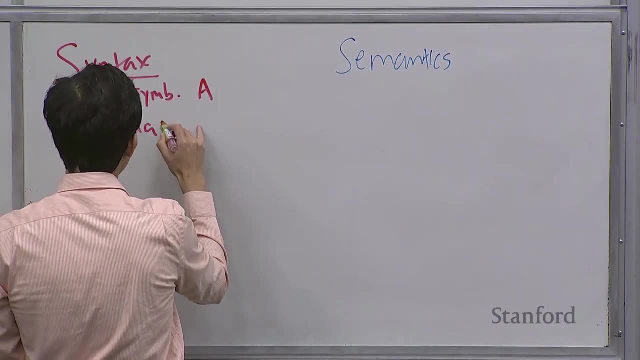 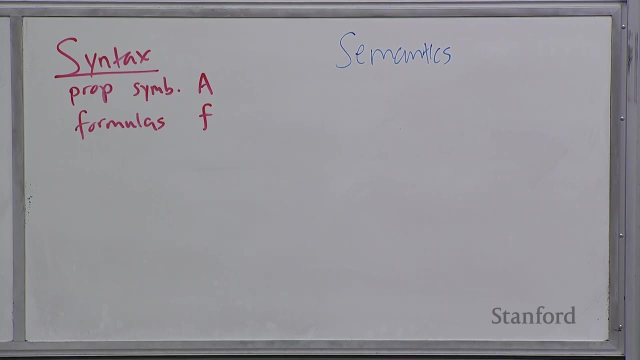 there's- that gives rise to formulas in general: um, which is gonna be denoted um, f, Um, and so here are some examples. So a is a formula, okay, It's- in particular, it's an atomic formula. 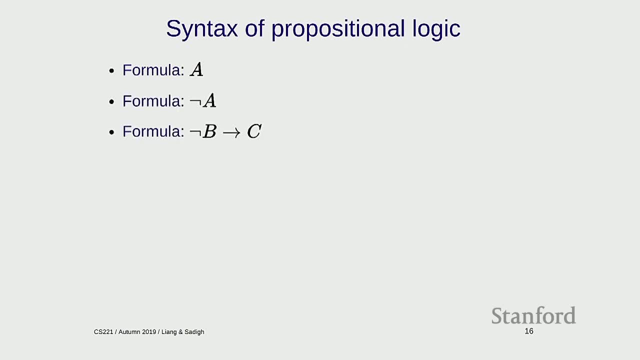 which is a propositional symbol. Not a is a formula. not b implies c is a formula. This is a formula. um, this is a formula. Double negation is fine. This is not a formula because there's no connective between a and not b. 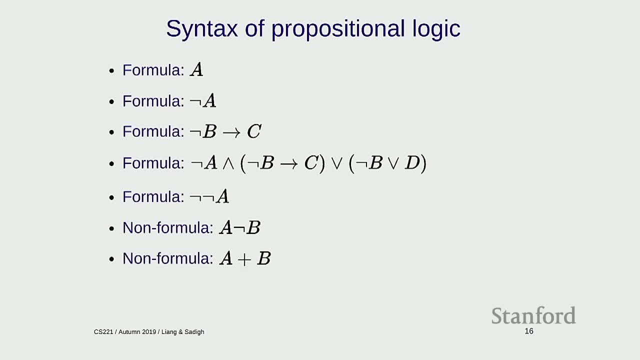 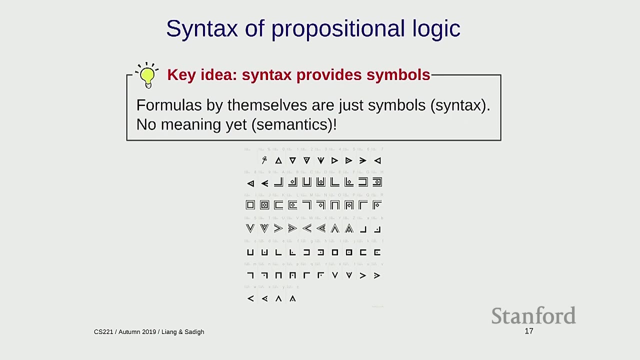 Um, this is also not a formula, because, um, what the heck is? plus Um, it's not a connective, So- so I think in- in thinking about logic, you really have to divorce yourself from the common sense that you all come with in interpreting these symbols, right? 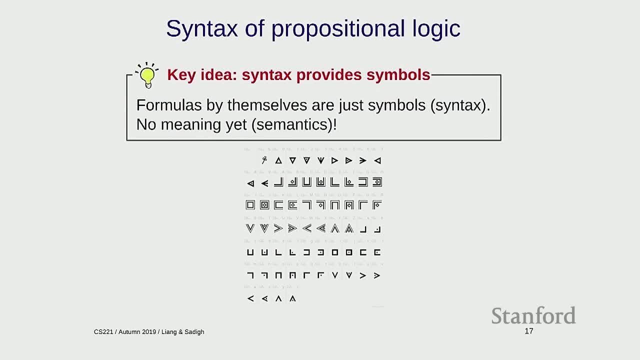 Not is just a symbol or is just a symbol, And they don't have any semantics In-. in fact, I can go and define some semantics which would be completely different from what you imagine. It would be a valid, logical um system. 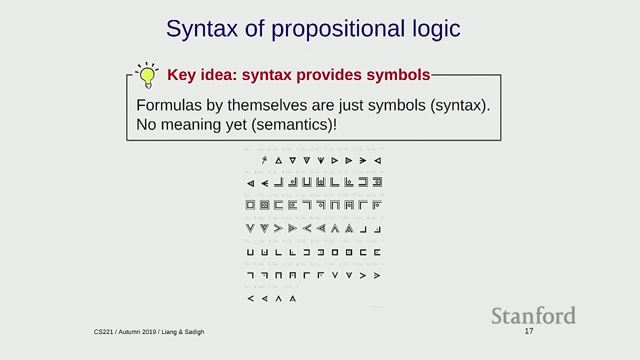 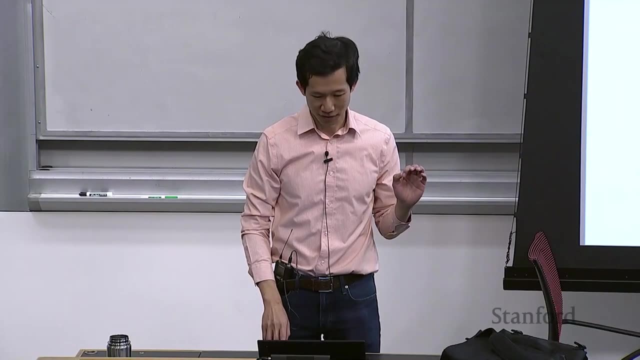 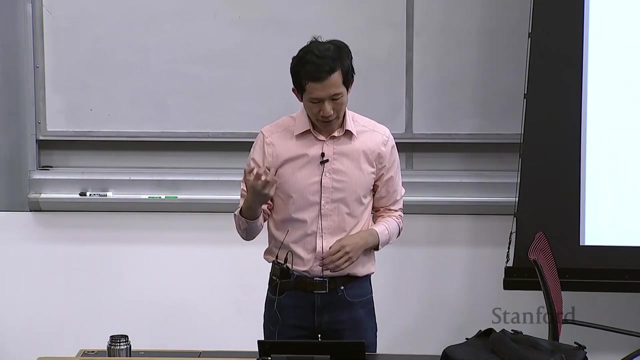 These are just symbols. Now, all I'm here defining is what symbols are valid and what symbols are not valid. slash grammatical. Okay, Any questions about the syntax of propositional logic. So the syntax gives you the set of formulas or, basically, statements you can make. 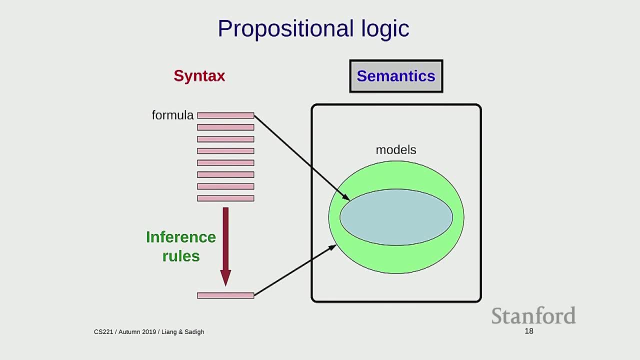 So you can think about as- as this is our language. If we could only speak in propositional logic, I could say a or not, b, or b or um. a implies c, and that's all. I would be able to say Um, and of course now I have to tell you what do. 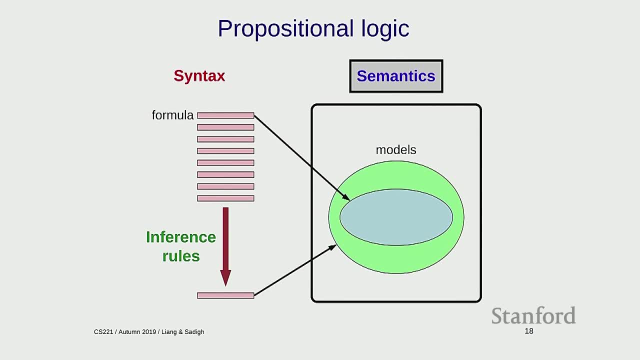 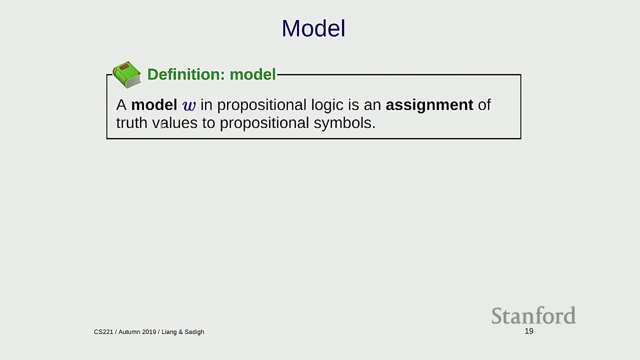 these things mean: okay, And this is the realm of semantics. So, semantics, there's gonna be a number of definitions. So first is a model. So this is really unfortunate and confusing terminology, but this is standard in the logical literature, so I'm just gonna use it. 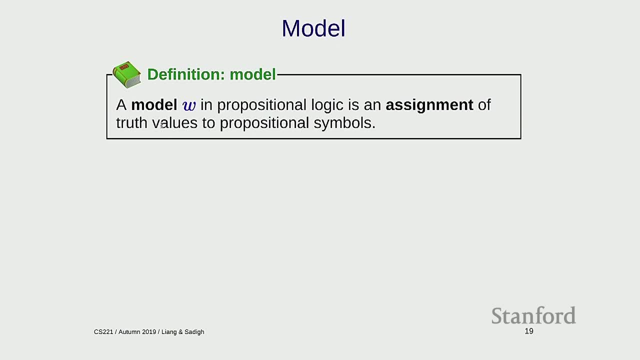 So a model which is different from our general notion of a model, um, for example, um hidden Markov model, for example- is a model here in propositional logic just refers to an assignment of um truth values to propositional symbols. okay, 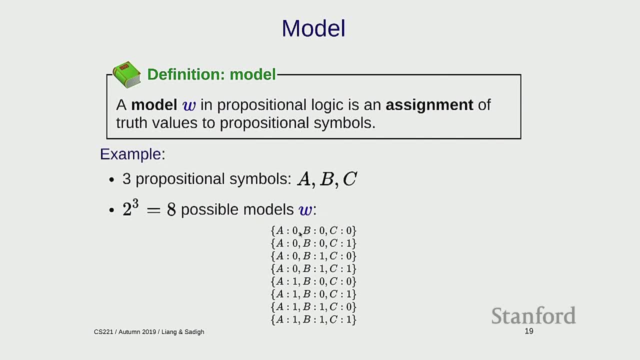 So if you have three propositional symbols, then there are eight possible models: Um a is uh 1, b is 0, c is 0,, for example. So these are just complete assignments that we saw from factor graphs. 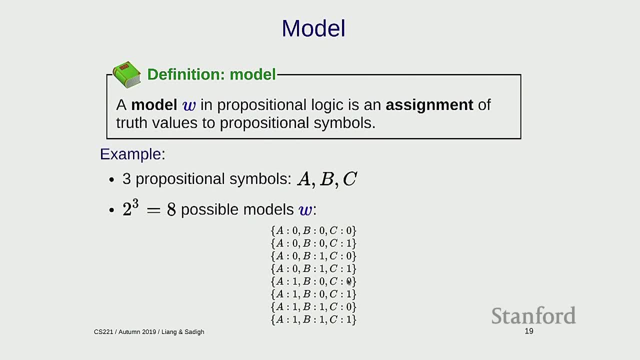 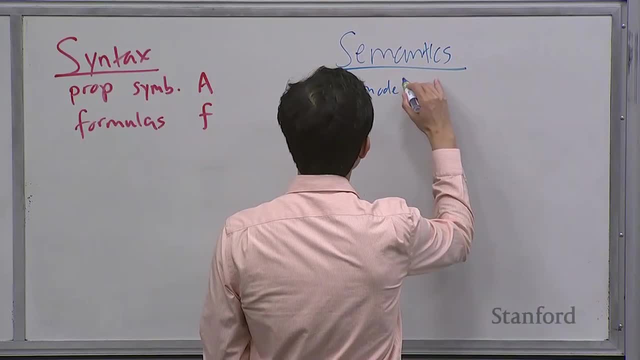 but now um in this new kind of language. okay, So that's the first concept, And in first-order logic, models are gonna be more complicated. um, but for now, think about them as complete assignments, And I'm using w because sometimes you also call them um. 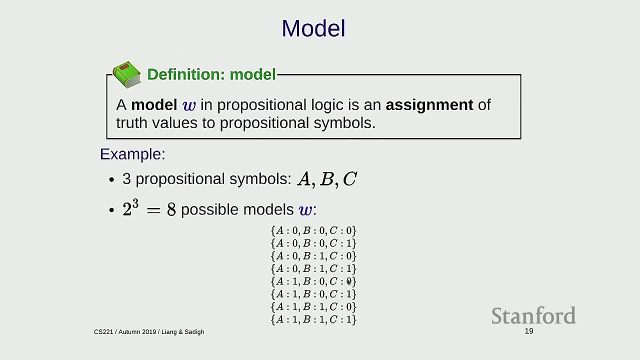 worlds. um, because a complete assignment slash, a model is supposed to represent the state of the world at any one particular point in time. Yeah, Can it only be either like true or false, 0 or 1? Is that like the domain, I guess? 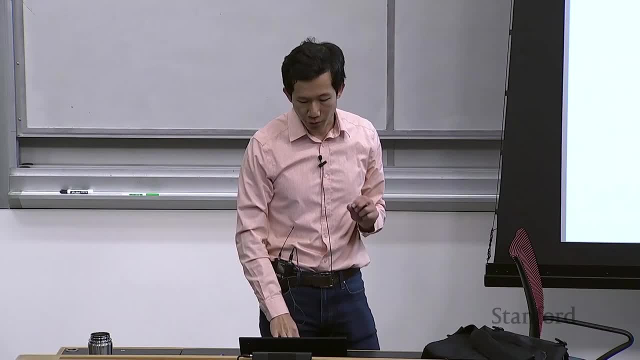 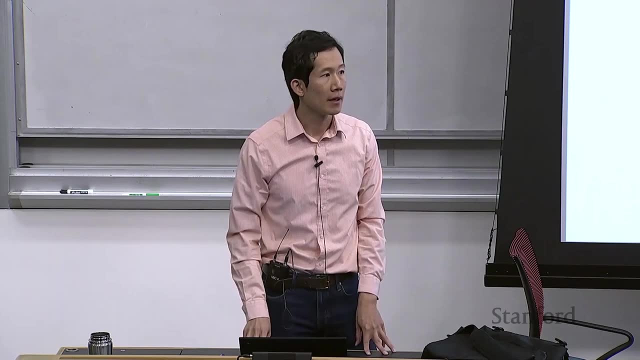 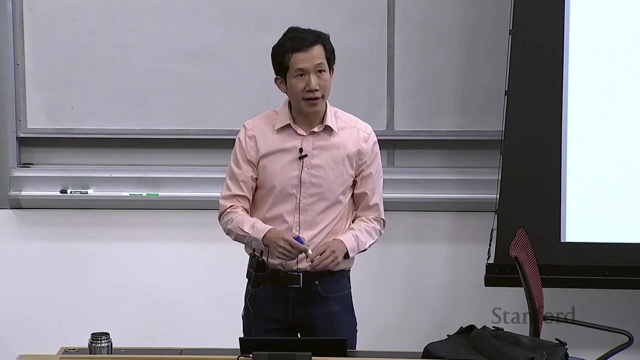 Yeah. So the question is: can each propositional symbol either be true or false? And in logic as I'm presenting it, yes, Only. true or false, Or 0 or 1.. Okay, So these are models. Um, and next is a key thing that actually defines the semantics. 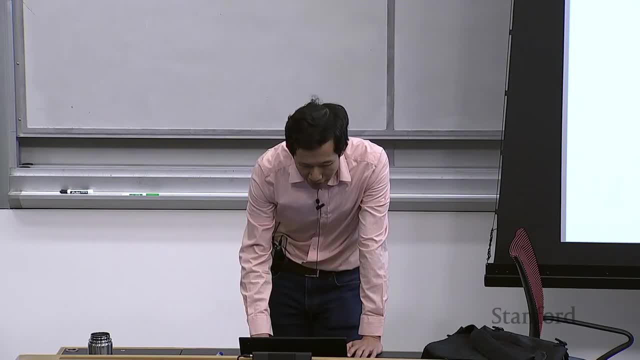 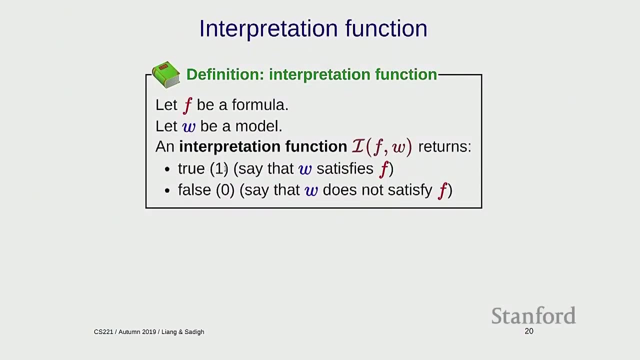 which is the interpretation function. So the interpretation function um takes a formula and a model and returns true if that formula is uh, is true in this model and false um, you know otherwise. Okay, So I can def- make the interpretation function whatever I want. 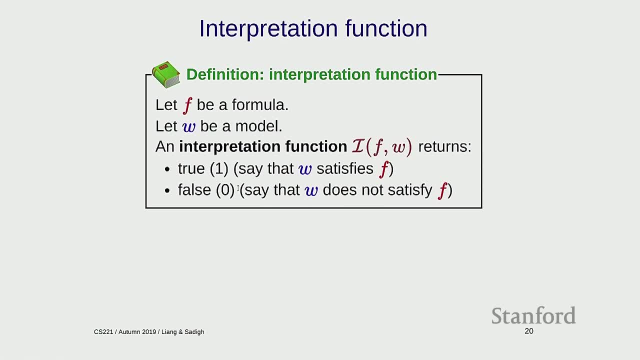 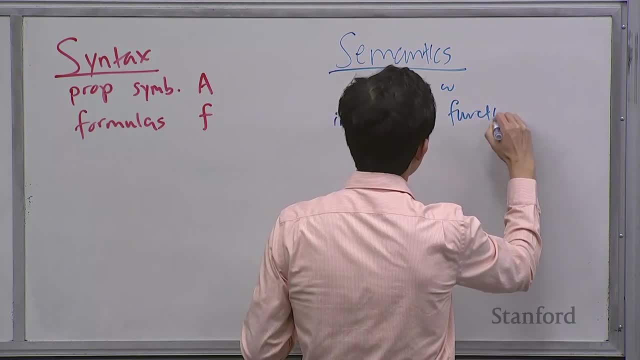 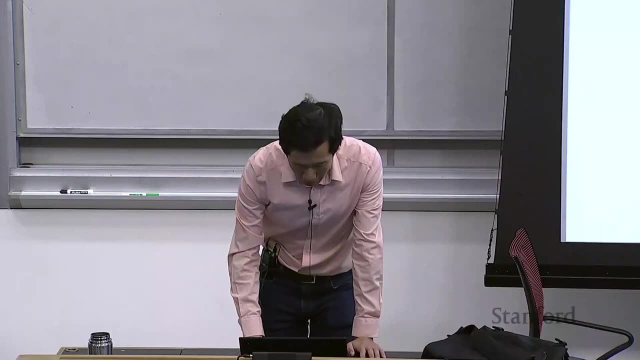 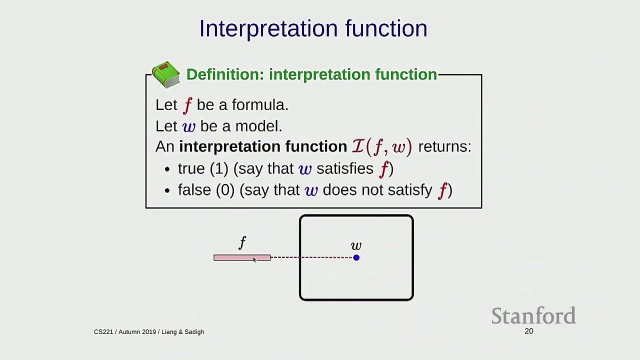 um, and that just gives me the semantics. So when I talk about what are the semantics, it's the interpretation function, Function i, um, f of w. So the way to think about this is: um. I'm gonna represent formulas as these: uh, horizontal bars. 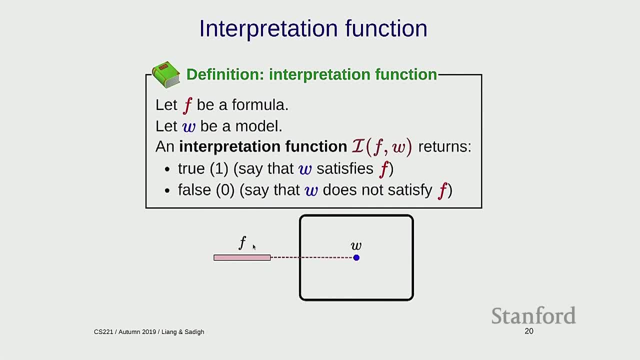 Okay, So this is- think about this as a- a thing you say It sits outside the uh reality in some- in some sense. And then this box I'm gonna draw on the space of all possible models. So think about this as a space of situations. 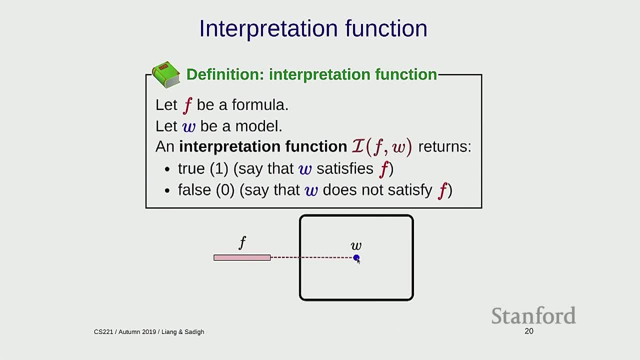 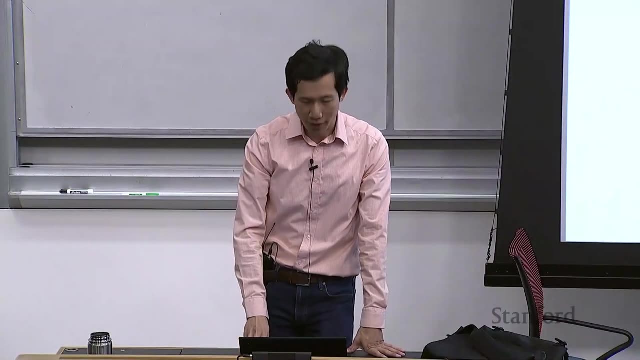 uh, that we could be in the world. And a point here corresponds to a particular model. So an interpretation function takes one- a formula, takes um a model and says: is this statement true if the world looked like this? Okay, So just to ground this out. 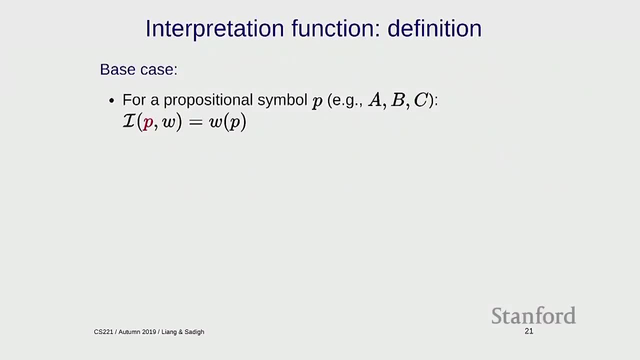 um, a little bit more. um, I'm gonna define this for propositional logic again recursively: Um. so for propositional symbols, um p, I'm just gonna interpret that propositional symbol as a lookup in, uh, the- the model right. 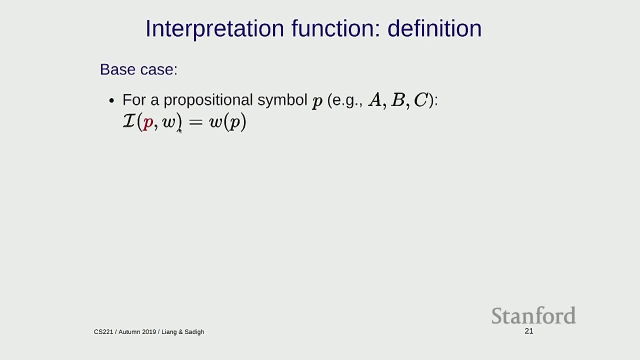 So if I'm asking, hey, is A true, will I go to my uh model and I see: well, does it say A is true or false? Okay, That's a base case. So, recursively, I can define the interpretation of any formula in terms of its sub-formulas. 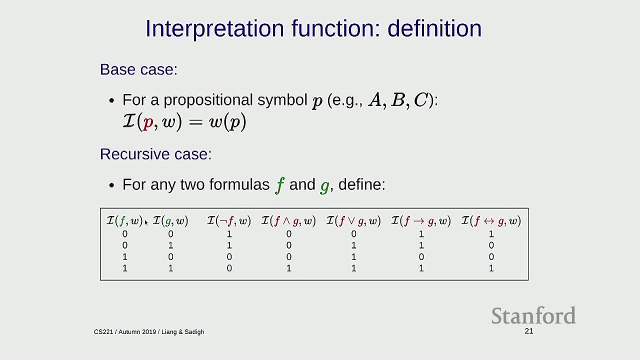 And the way I do this is suppose I have two formulas, F and G, and they're interpreted in some way. Okay, And now I take a formula, let's say F and G. Okay, So what is the interpretation of F and G? um in W. 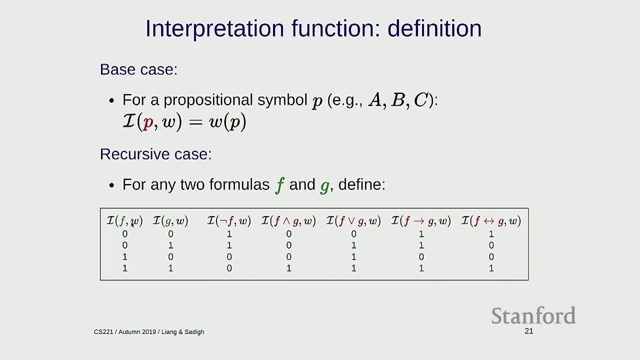 Well, it's given by this truth table. So if F is 0 and G is uh interpreted to be 0, then F and G is also interpreted to be 0.. And um 0, 1 maps to 0,. 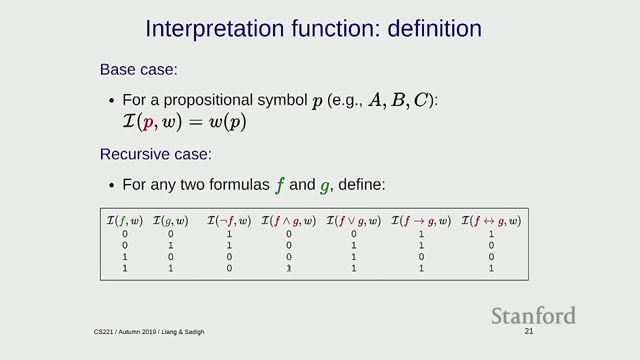 1, 0 maps to 0, and 1, 1 maps to 1.. So you can verify that this is kind of um, your intuitive notion of what AND should be Right. Um or is um? 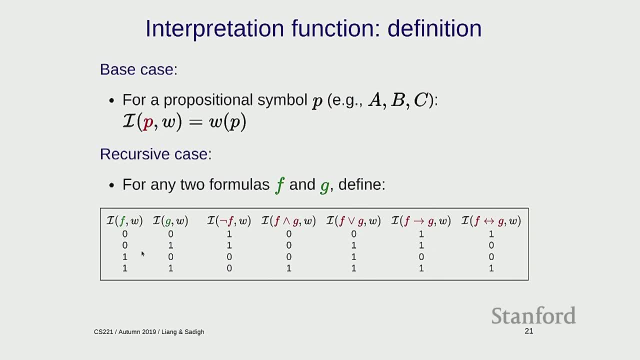 1 if um at least 1 of F and G are 1? Um implication is 1. if F is 0 or G is uh, is is 1.. Um bi-directional implication just means that if F and G evaluate to the same thing. 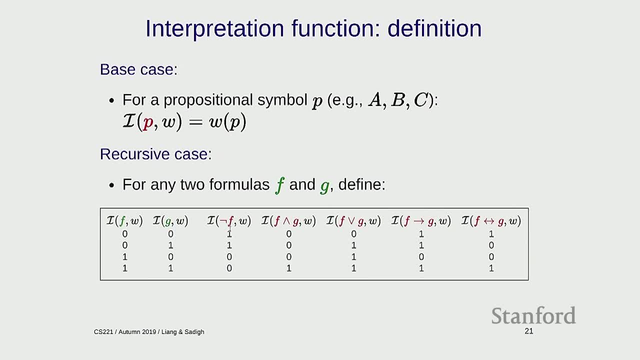 um, not F is you know clearly. just you know, negate Negation of whatever the interpretation of F is Okay. So this slide gives you the full semantics of propositional logic. There's nothing more to propositional logic. 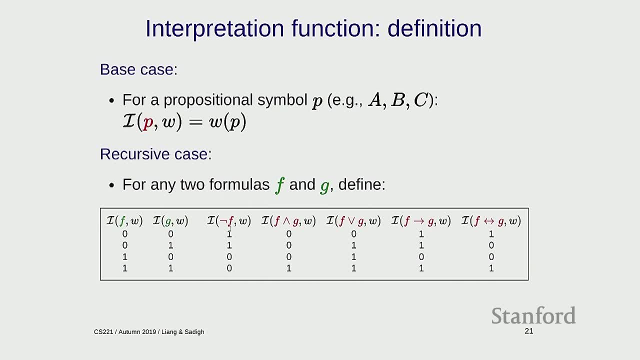 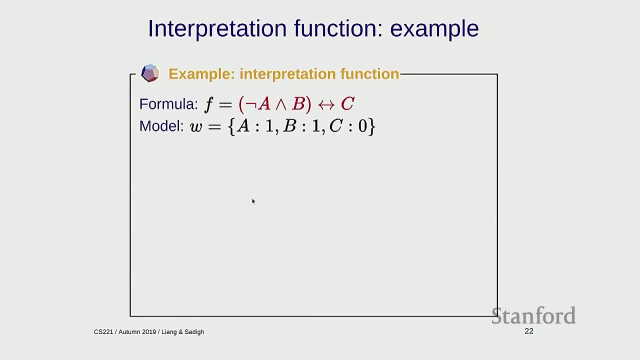 at least the definition of what it is, um. aside from this Um, let me go through an example and then I'll maybe take questions. So so let's look at this formula: not A and B. bi-directional implication C. 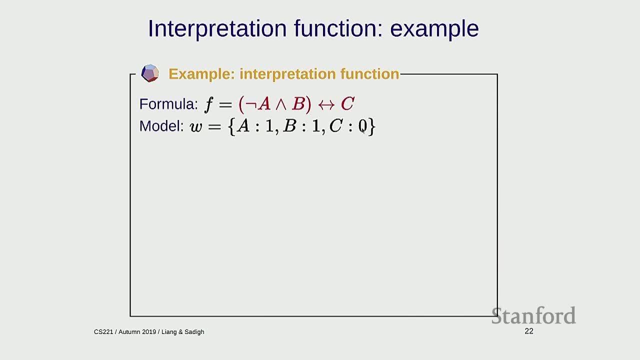 Um, and this model, A is 1,, B is 1,, C is 0.. Um, how do I interpret this formula against this model? Well, I look at the, the tree um, which breaks down the formula. 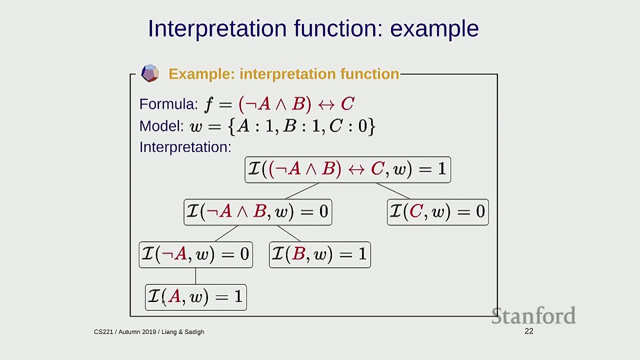 So if I look at the leaves, um, let's start bottom up. So the interpretation of A against W is just 1, because for propositional symbols I just look up what A is and A is 1 here. Um, the interpretation of not A is 0, because 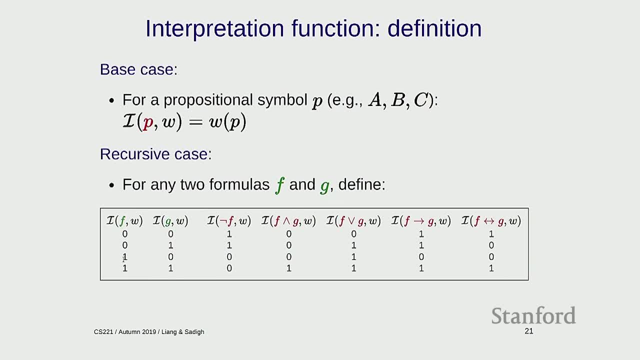 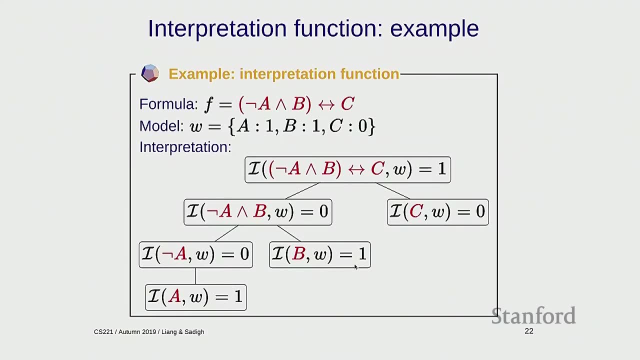 if I look back at this table, if this evaluates to 1, then this evaluates to 0 and just looking um based on the table, Um B is 1, just by table lookup, And then um, not A, and B is 0,. 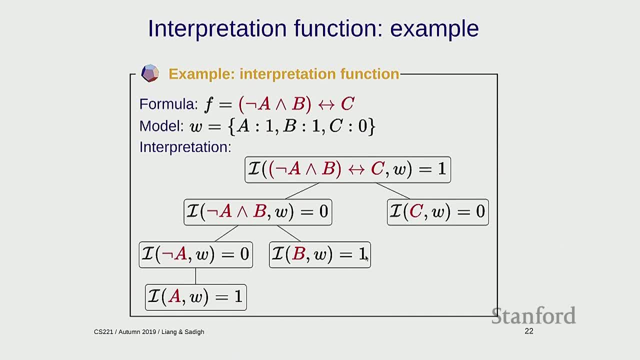 because I just take these two values and I and them together, Um C is 0 by table lookup and then by directional implication, um is interpreted as as uh 1 here because 0 is equal to 0.. 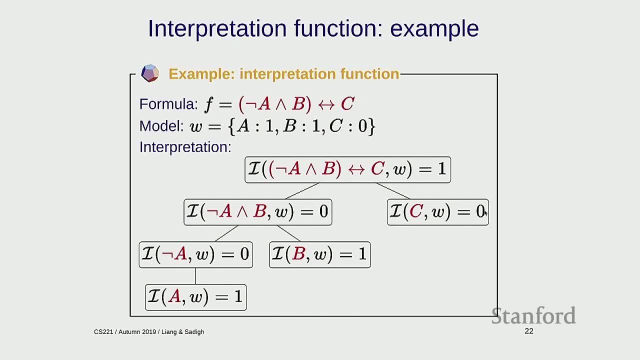 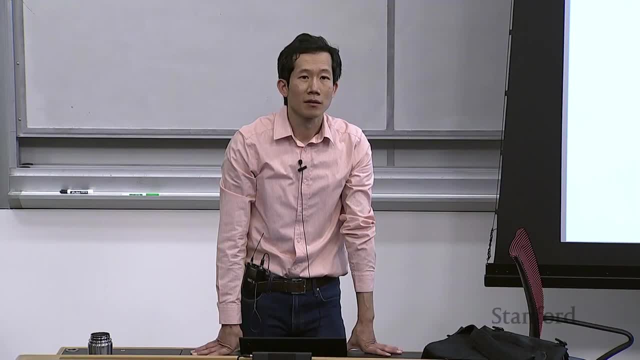 Yeah Yeah, question Interpretation function is user-defined in this case. right, Like you're not like learning how to interpret the proposition of logic, just like if you did the proposition of logic, then like you have two tables in the field, basically. 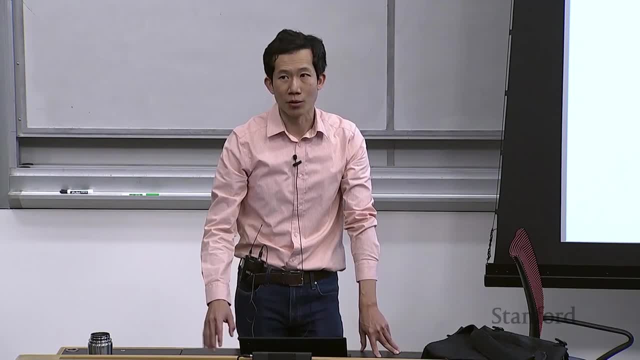 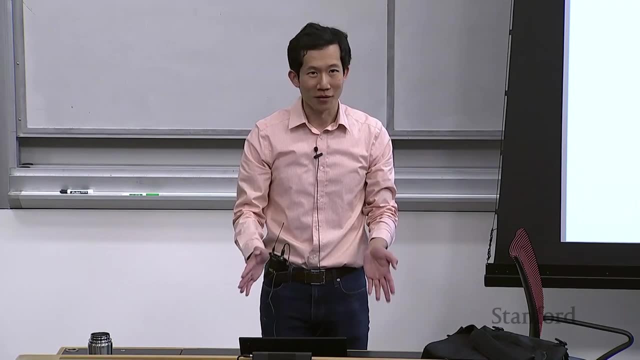 Yeah. So the question is: uh, is the interpretation function just, uh, user-defined? It is just written down: um, this is it. There's no learning, it's just: these are- this is what you get. Um, it's not user-defined in the sense that not everyone's. 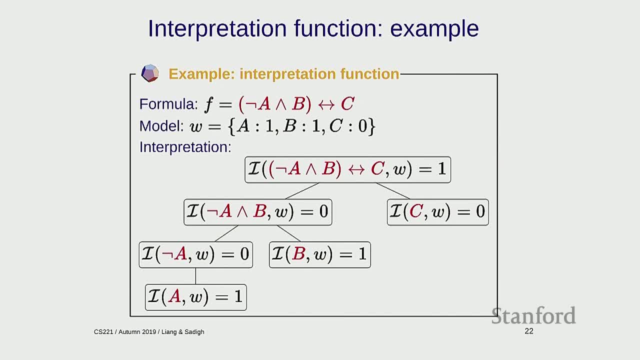 gonna go define their own. you know, truth tables, Um. some logicians came up with this and that's what it is. Um, but you could define your own logics and it's kind of a fun thing you could try doing. 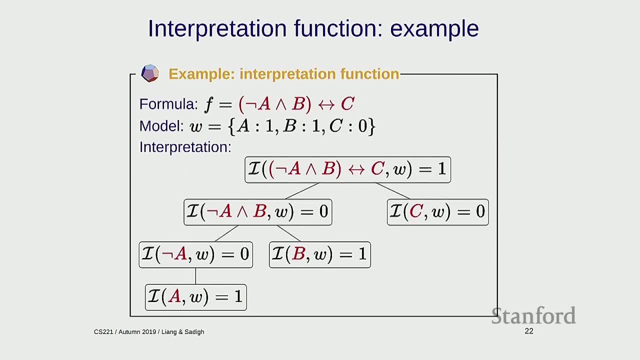 Okay, Any other questions about interpretation functions and models. So now we're kind of connecting syntax and semantics, right? So an interpretation function binds what are formulas which are in syntax land to um, a notion of models which are, uh, in semantics. 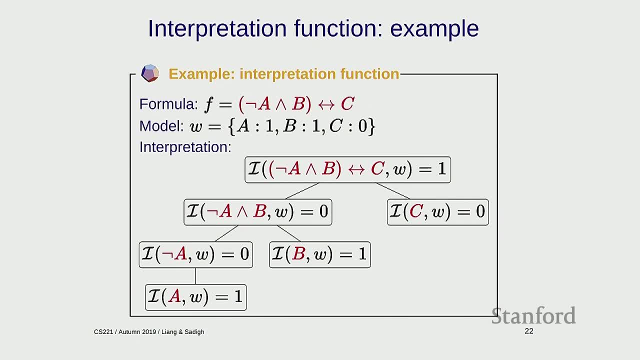 So a lot of logic is very- um, it might seem a little bit pedantic, but it's just because we're trying to be very rigorous in a way that doesn't need to appeal to your common sense intuitions about what these formulas mean. 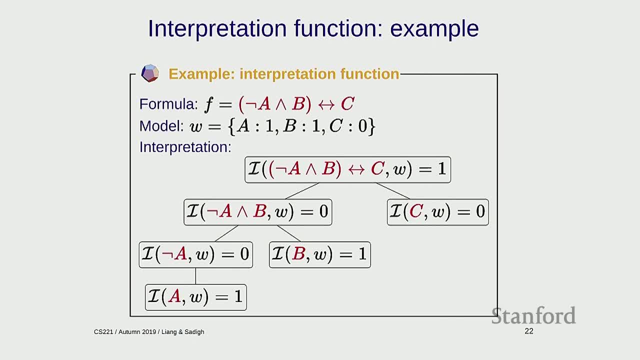 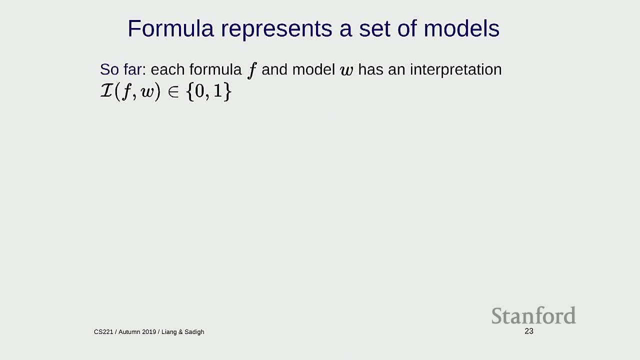 Okay, Any questions? All right, So so, while we have the interpretation function and it defines everything, it's really going to be useful to think about formulas in a slightly, uh, different way. So we're gonna think about the f- a formula. 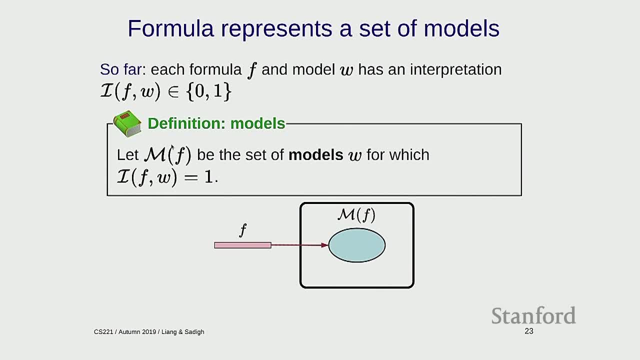 um as representing, um, the set of all models, right, Okay, Okay, Okay, Okay, Okay. So we're going to think about a set of models for which interpretation is you know, true? Okay So, M of f. 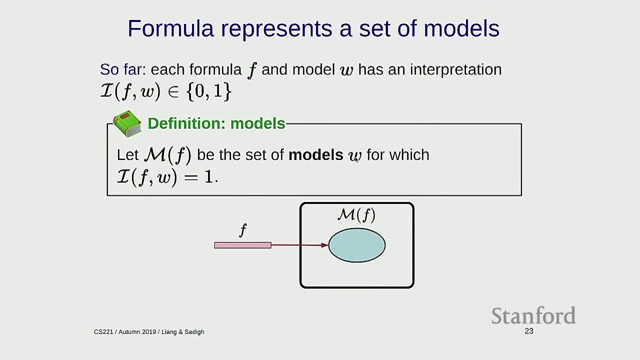 which is this- is the set of models- um, that f is, uh, true on that model. Okay, So, pictorially, this is a f that you say out loud, And what you mean by this is simply this subset of models, which this f is true. 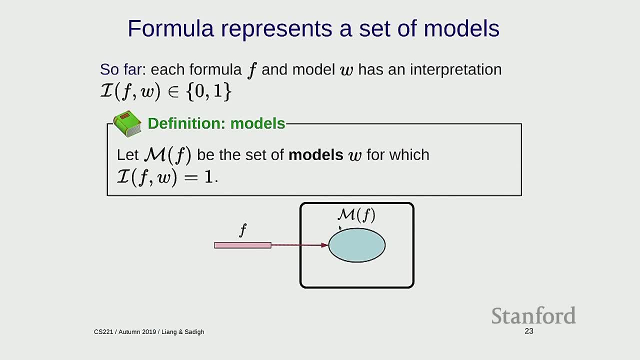 Okay. So if I make a set of models statement here, what I'm really saying is that I think we're in one of these models and not in one of these other models, So that's a kind of an important, I think- intuition to have. 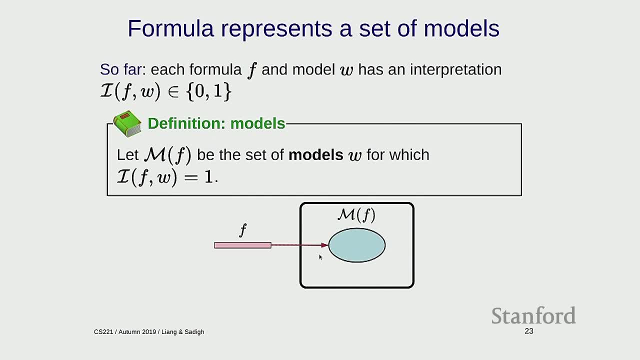 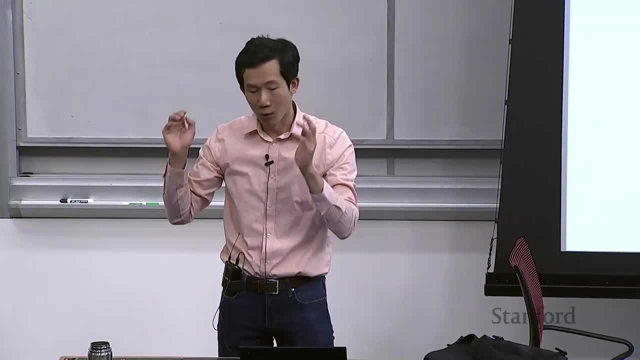 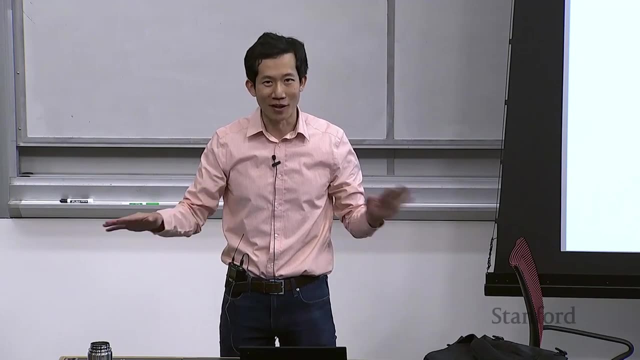 The meaning of a formula is carving out a space of possible situations that you can be. If I say there's a water bottle on the table, what I'm really saying is that I'm ruling out all the possible worlds we could be in where there is no water table- bottle on the table. 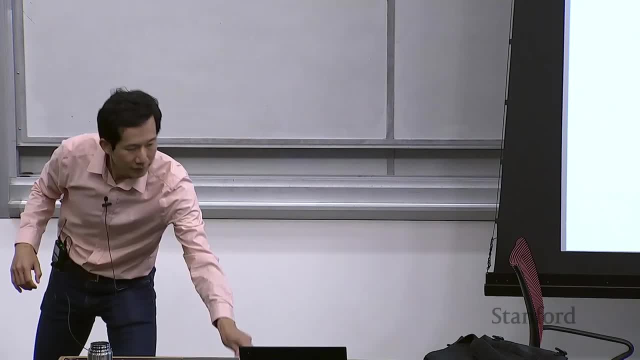 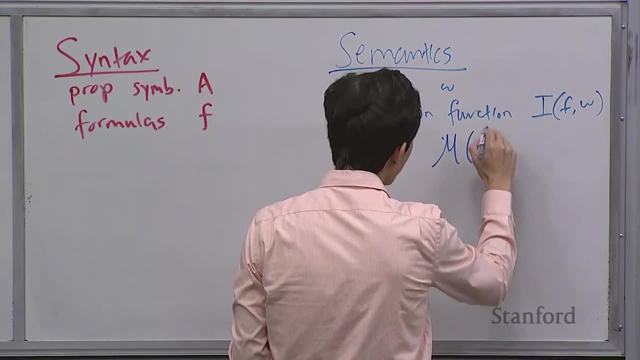 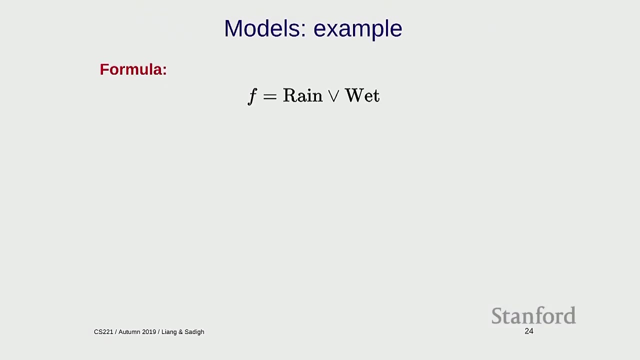 Okay, So models um, M of f is going to be a subset of all the possible models in the world. Okay, So here's an example. So if I say it's either raining or wet, rain or wet, then the set of models can be represented by this subset of this two-by-two. 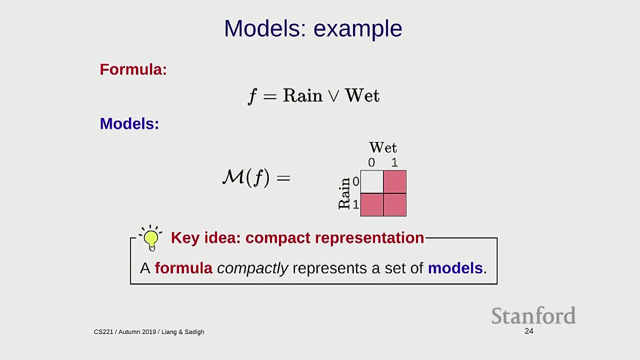 Okay, So over here I have rain, over here I have wet. So this corresponds to no rain, but it's wet outside. This corresponds to it's raining, but it's not wet outside, And the set of models f is this red region. 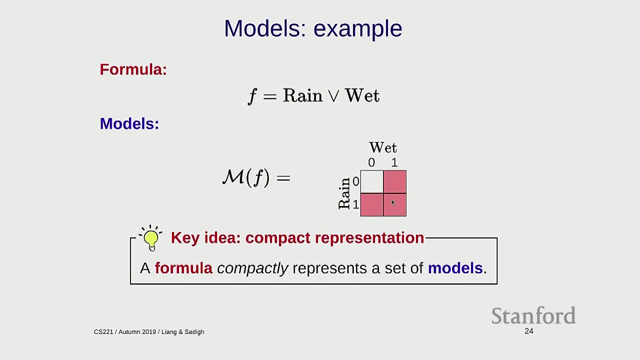 which are these three possible models? Okay, So I'm gonna use this, this kind of pictorial depiction, throughout this lecture, So hopefully this makes sense. So so one key idea here. remember I said that logic allows you to express very complicated and large things by using very small means. 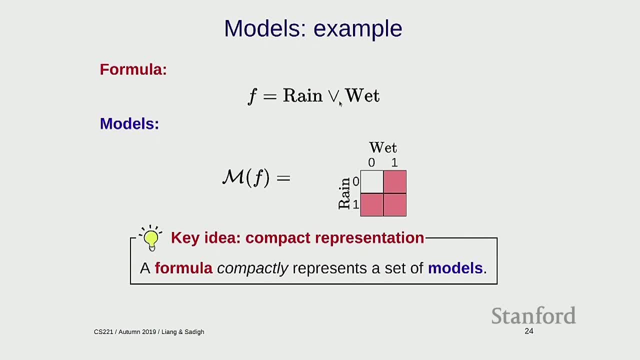 So here I have a very small formula that's um able to represent a set of models, and that set of models could be exponentially large- And much of the power of logic allow- it- comes from the ability to um do stuff like that. 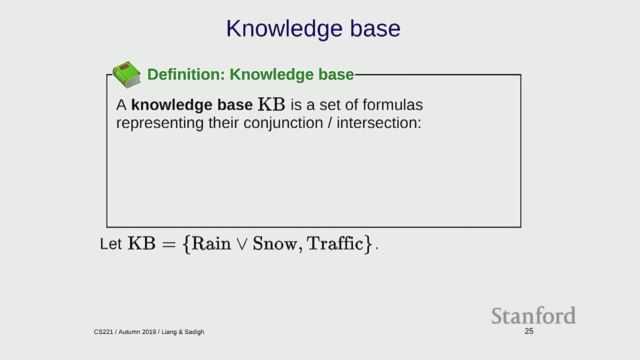 Okay, So, um, here's yet another definition. This one's not somehow um such a new definition, um, oh sorry, a new concept, but it's kind of just trying to give us a little bit more intuition for what these. 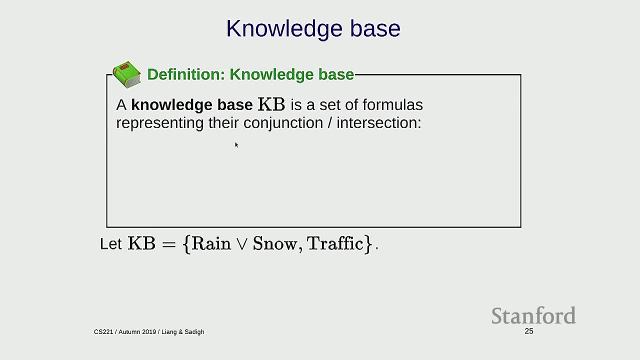 um formulas and um models are doing So. a knowledge base is just a set of formulas. Um, and think about this as the set of facts you know about the world. So this is what you have in your head And, in general, it's going to be a- just a set of formulas. 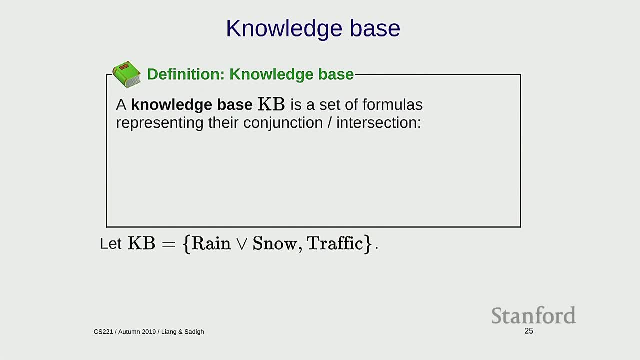 And now the the key thing is, I need to connect this with semantics. So I'm gonna define the set of models denoted by a knowledge base to be the intersection of all of the models denoted by the formulas. So, in this case, if I have rain or snow being this, uh well, 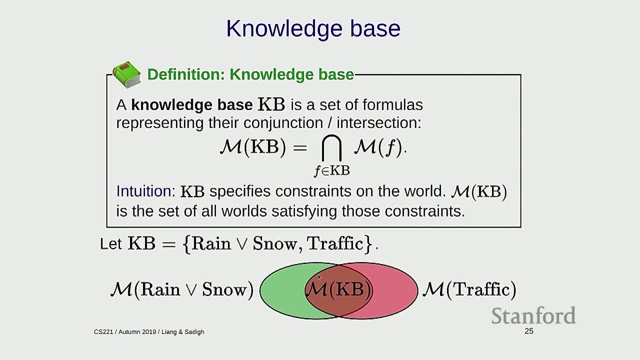 um, green ellipse and traffic being this, uh, red ellipse, then the models denoted by the knowledge base is just the intersection. okay, So you can think about knowledge as how fine-grain. uh, we've kind of zoomed in on where we are in the world, right? 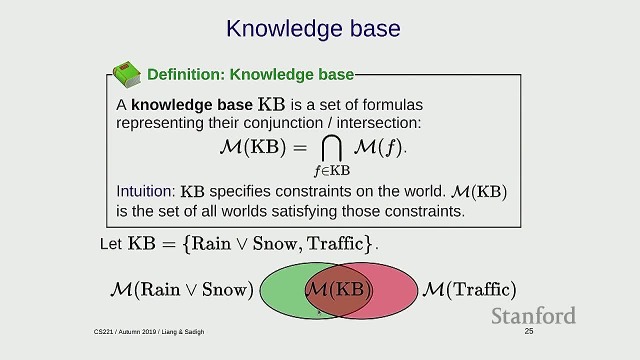 So initially you don't know anything. We say anything is possible, all two to the n. you know models are possible And as you add formulas into your knowledge base, the set of um possible worlds that you think might exi- are possible is going to shrink. 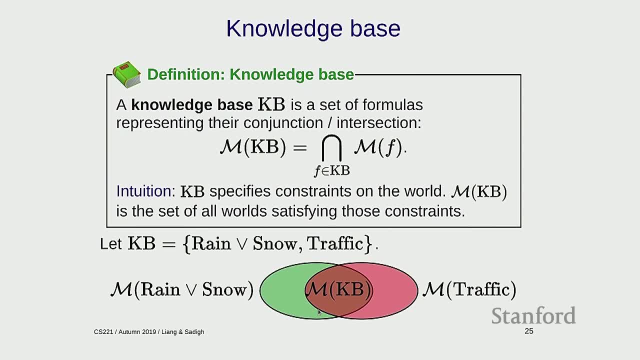 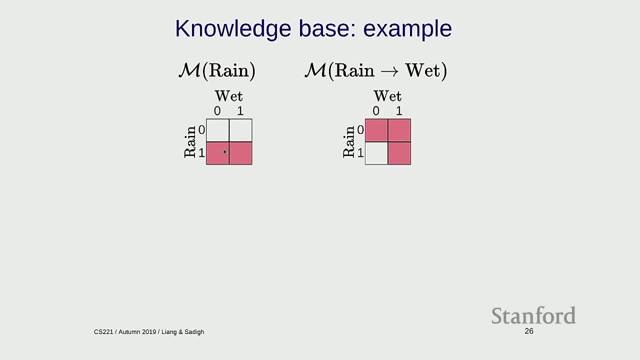 Um, and you know we'll- we'll see that in this- in a second. Okay, So here's an example of a knowledge base. if so, I have rain. that corresponds to this set of models. Rain implies wet, corresponds to this set of models. 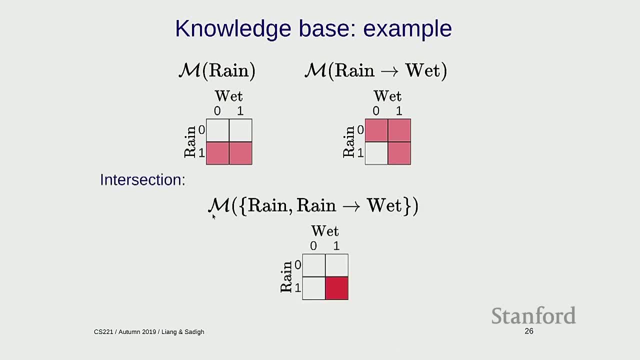 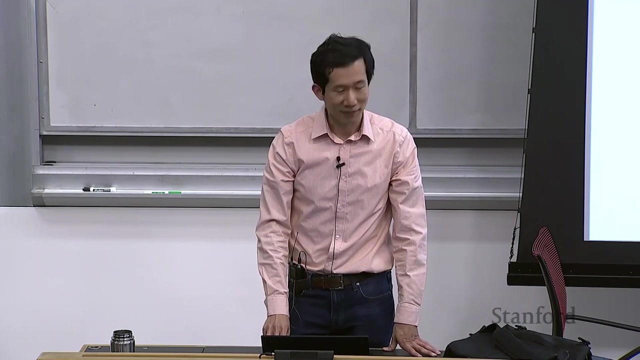 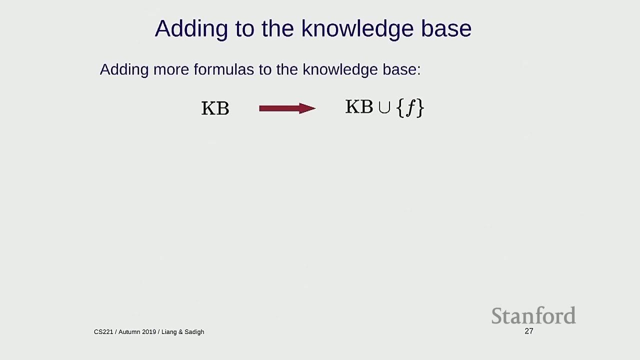 And if I look at the models of this knowledge base, it's just going to be the intersection, which is this: uh, red square down there. Okay, Any questions about knowledge bases, models, interpretation functions. so far All right. So, as I've alluded to earlier, 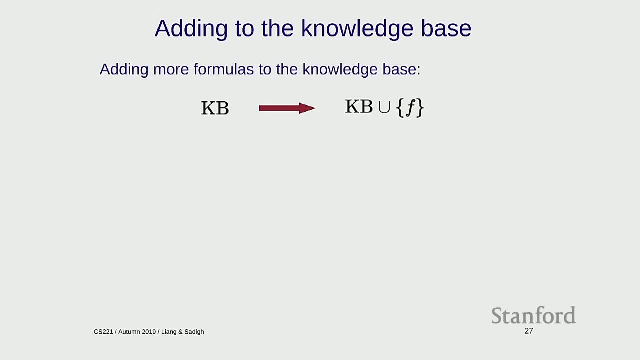 knowledge base is this thing you have in your head, and as you go through life, you're going to add more formulas to your knowledge base. you're gonna learn more things, Um, so your knowledge base just gets uh union with whatever formula you- you have. 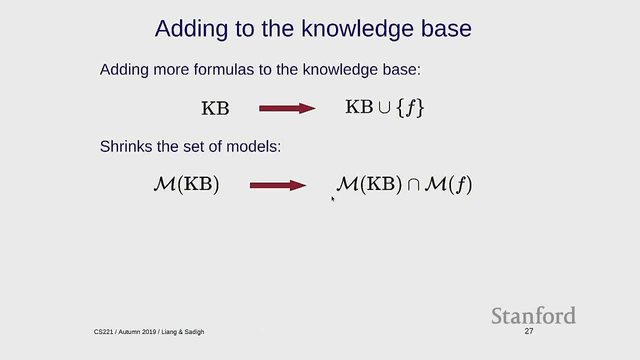 And over time, the set of models is going to shrink, because you're just taking an intersection, Um, and one question is: you know how much is this, uh, shrinking? Okay, So here there is a bunch of different cases. 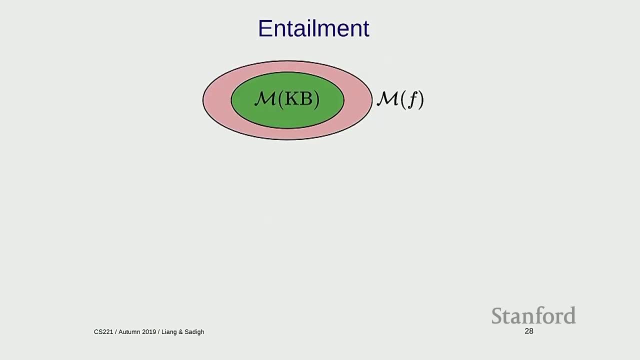 to contemplate Um. the first case is um entailment. So suppose this is your knowledge base so far. and then someone tells you um the formula that corresponds to this uh, set here. okay, So in this case, um. 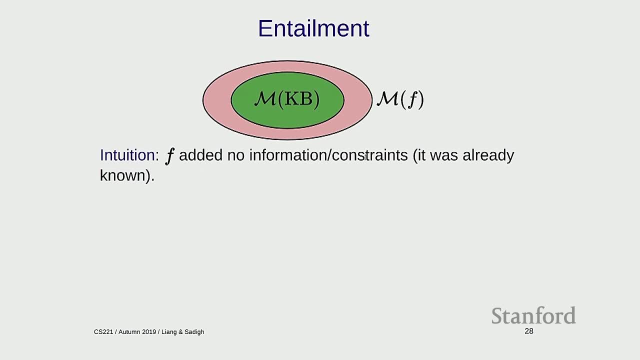 intuitively. f doesn't add any information or new constraints. that was known before And, in particular, if you take the intersection of these two, you end up with exactly the same set of models you had before, So you didn't learn anything. Um, and this is called entailment. 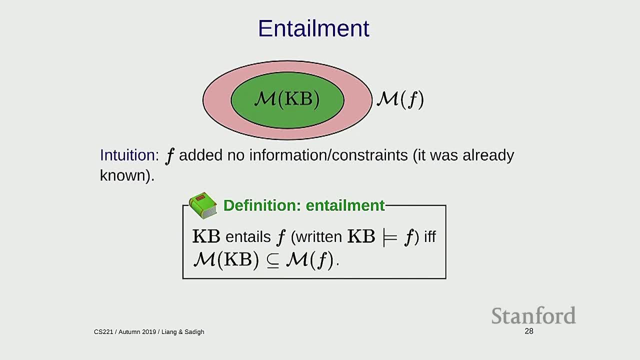 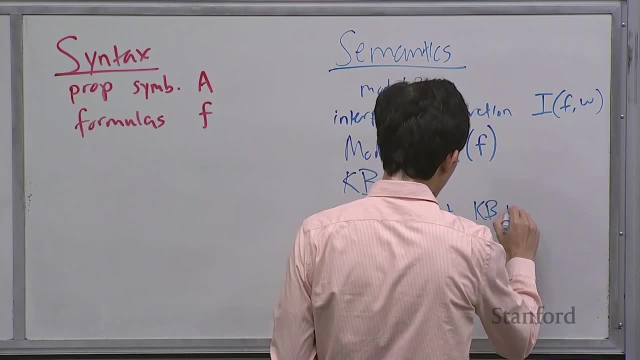 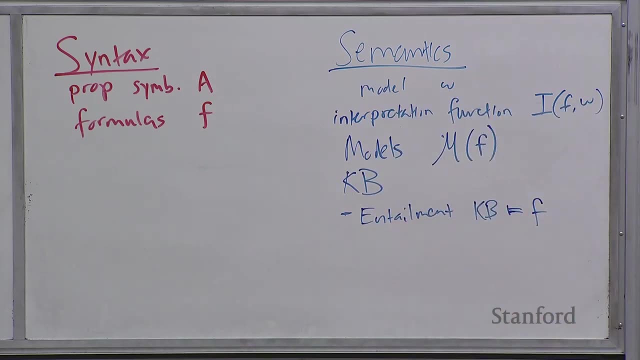 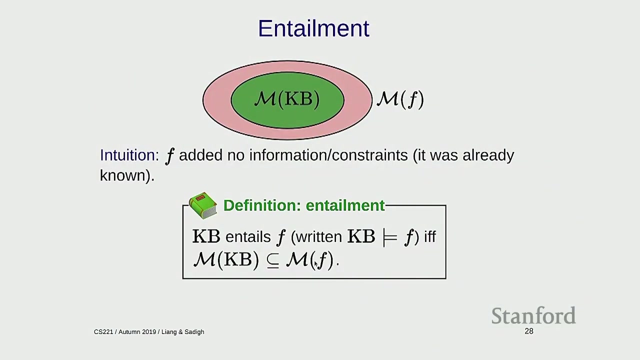 So, um. so there's kind of three notions here. There's entailment which is written this way, with two horizontal uh bars, Um, which means that the set of models um of f is at least as large as the set of models in. 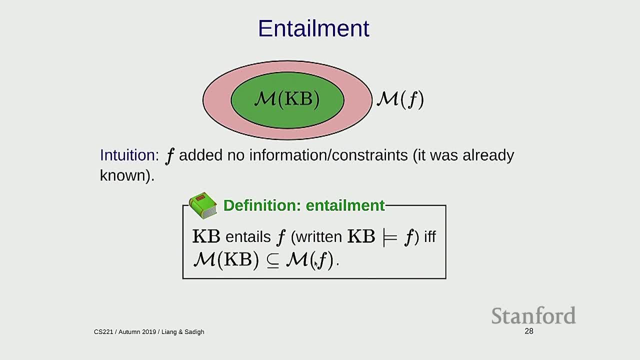 uh, KD, or in other words, it's a superset, okay, Um so, for example, rain and snow. If you already knew it was raining and snowing and someone tells you: ah, it's snowing, then you say: 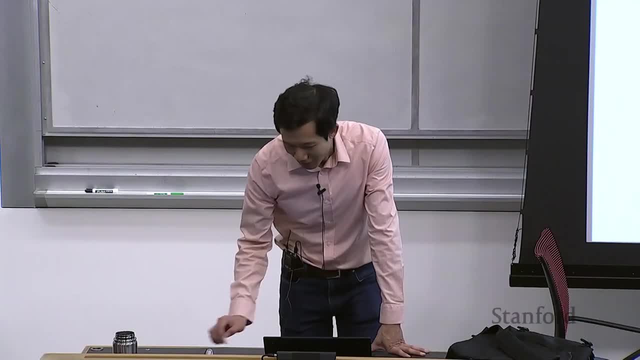 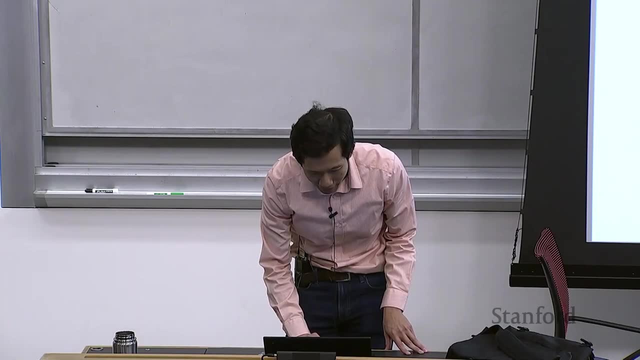 well, um duh, I didn't learn anything. Um, a second case is contradiction. So if you believe the world to be in here somewhere and someone told you it's actually out here, then, um, your brain explodes, right. 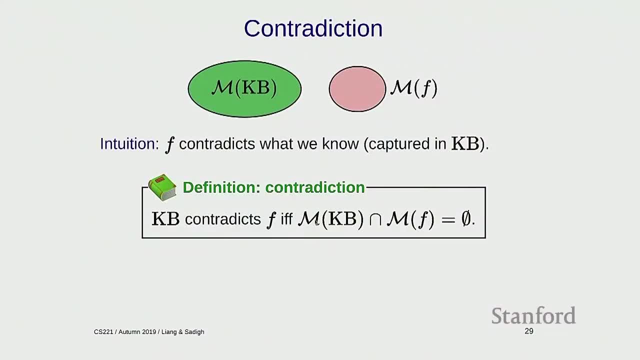 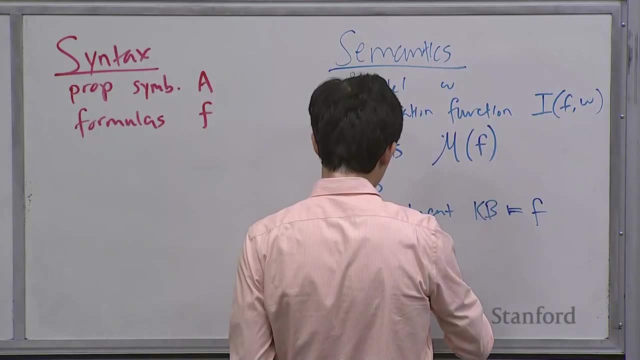 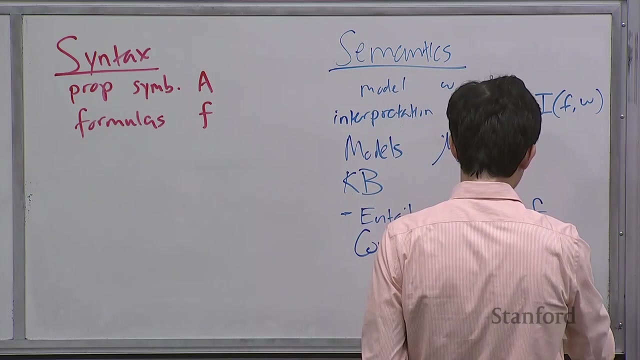 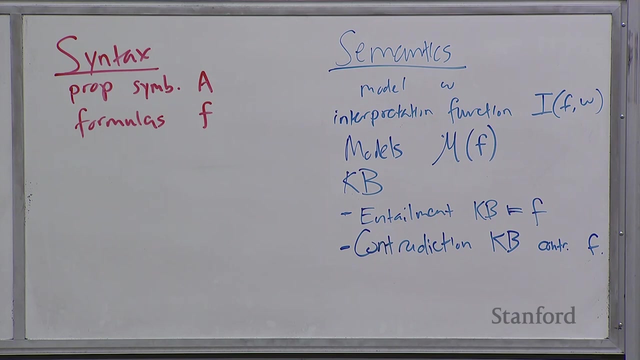 Um, so this is where the set of models of the knowledge base and the set of models denoted by the formula is empty. So this doesn't make sense. Okay, So that's a contradiction. Um, Okay, So if, uh, 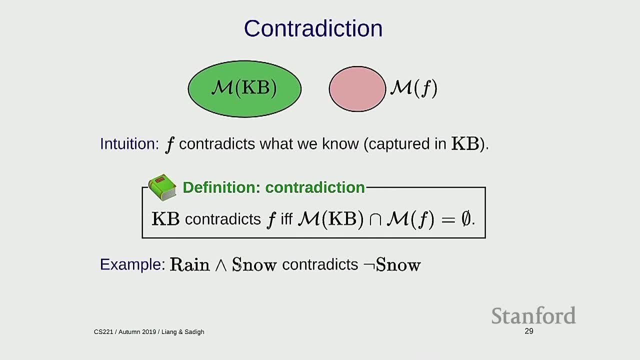 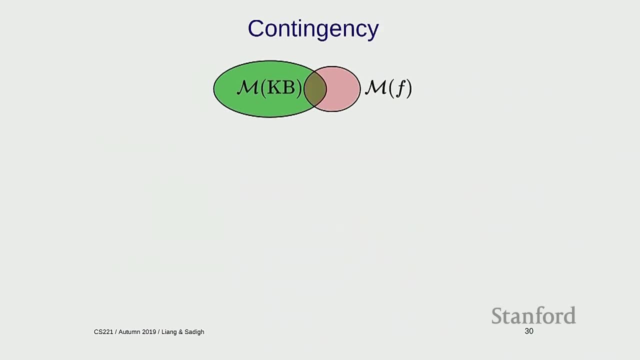 you knew it was raining and snowing and someone says it's actually not snowing, then you would be like, no, that, that can't, that can't be right, Okay. So the third case is: um, basically everything else. 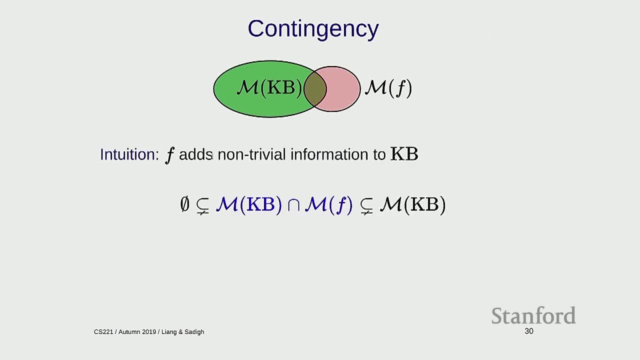 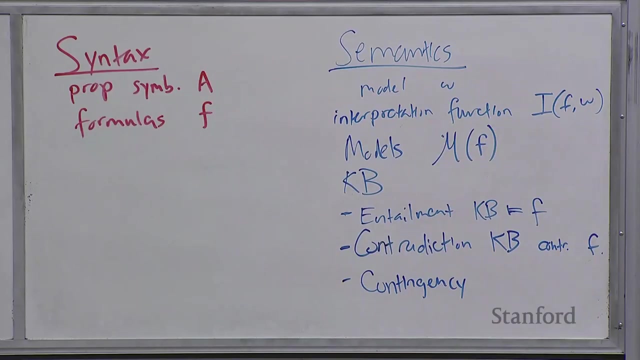 It's contingency where um f adds a non-trivial amount of information to a knowledge base. So the the new set of models, the intersection here is neither empty nor is it the original knowledge base. okay, Um, one thing to kind of. 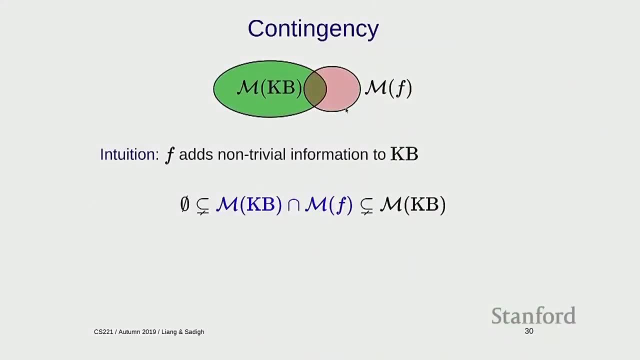 uh, not get confused by is. if the set of models were actually strictly inside the knowledge base, that would also be a contingency right, Because when you intersect it it's neither empty nor the original. Okay, So if you knew it was rainy ants. 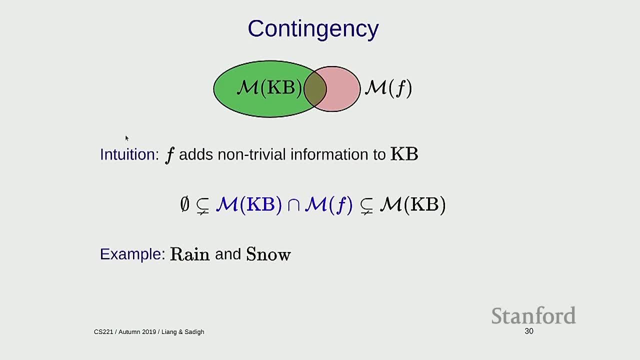 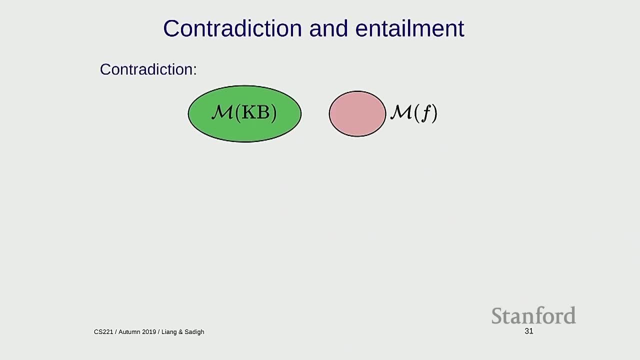 um raining and someone said: oh, it's also snowing too. then you're like: oh cool, I learned something. Okay, So there there's a relationship between contradiction and entailment. So contradiction says that the knowledge base and f 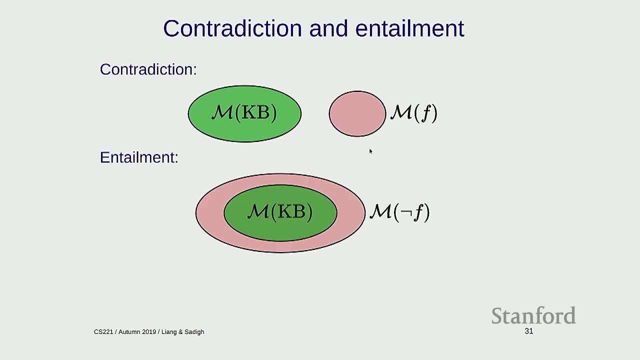 um are have zero intersection And entailment um, this is equivalent to um, the knowledge base, entailing not f. Okay, So just just there's a simple proposition that says um KB contradicts f if KB. 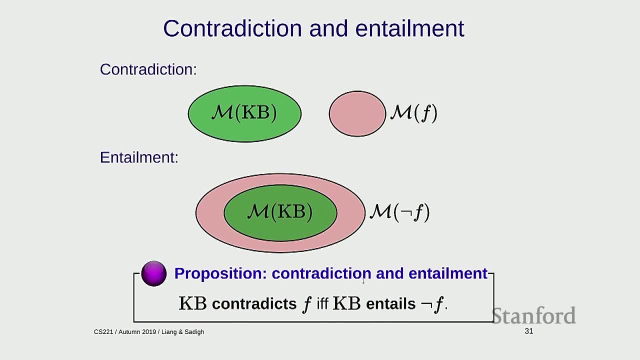 if an f KB entails not f, Okay. So, um, this, the picture you should have in here is like: not f is all the models which are not in this, And if you think about kind of wrapping that around it, you know, looks like this: 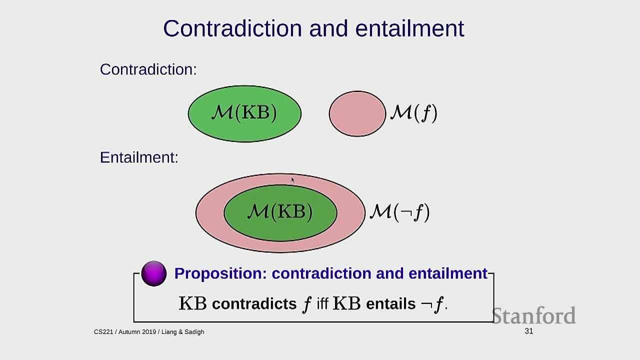 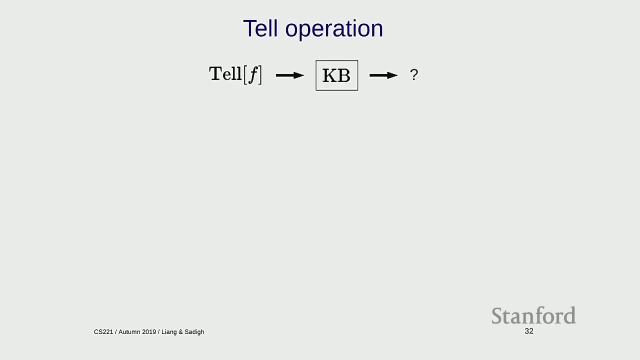 Okay, All right. So with these three um notions- entailment, contradiction and contingency- which are relationships between a knowledge base and- uh, a new formula- we can now go back to our kind of virtual system example and think about how to implement. 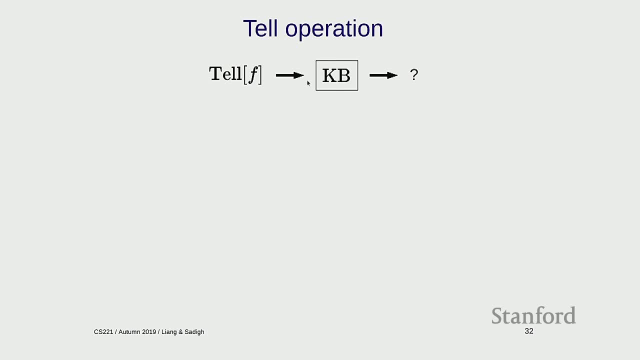 um these operations. So if I have a knowledge base and I tell um the, the virtual system of a particular, um formula f, there are three possible abilities which correspond to different appropriate responses. So if I say it's raining, 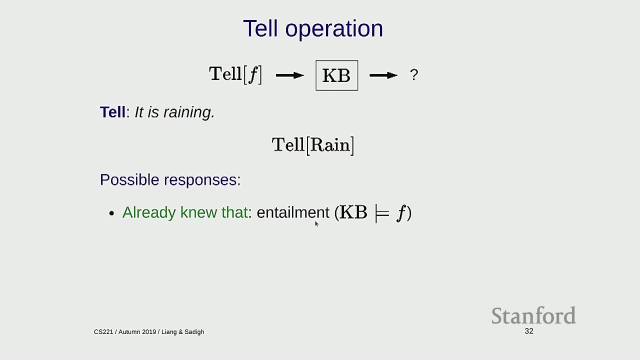 then if it's an entailment, then I say I already knew that, because I didn't learn anything new. If it's a contradiction, then I should say I don't believe that because it's not consistent with my knowledge so far, And otherwise you learn something new. 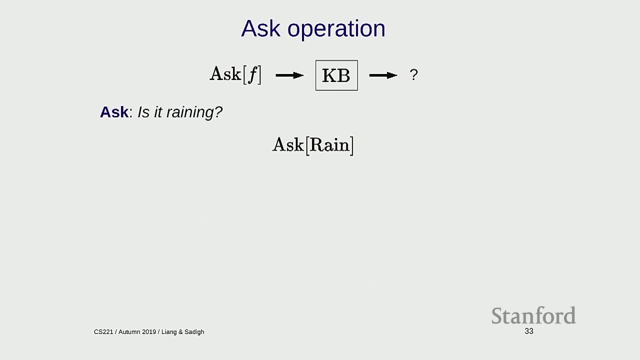 Okay, Um, there's also the ask operation which, if you're asking a question again, the same three uh, entailment, um, entailment, contradiction and contingency can hold, Um, but now the responses are: uh, should be answers to this question. 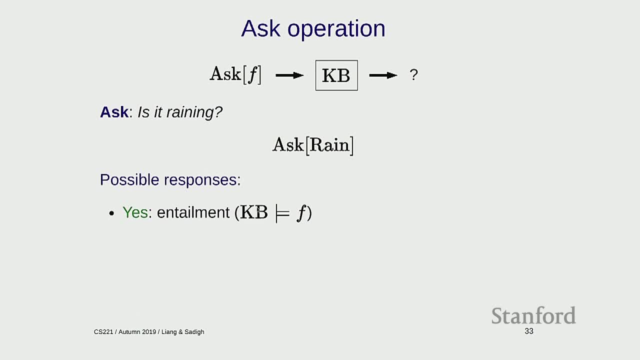 So, um, if it's entailment, then I say yes, And this is a strong yes. This is not like, uh, probably yes, This is a definitely yes. Um, if it's a contradiction, then I say no. 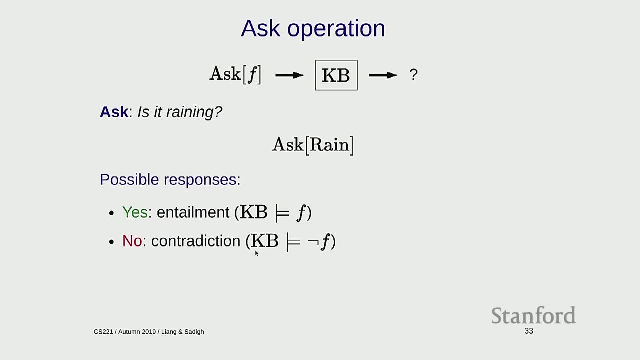 It's again, it's a strong no, It's impossible. And then in the other case it's just contingent, which you say I don't know. Okay, So the answer to a yes or no question, there's three responses, not two. 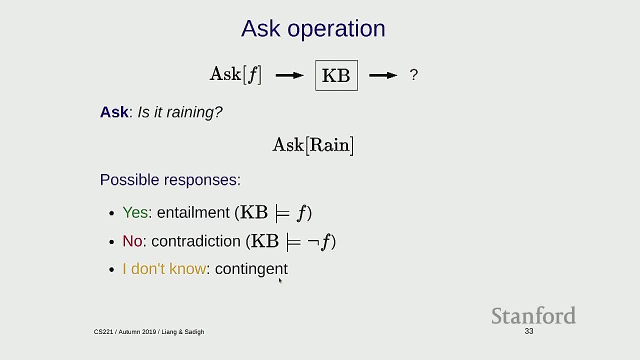 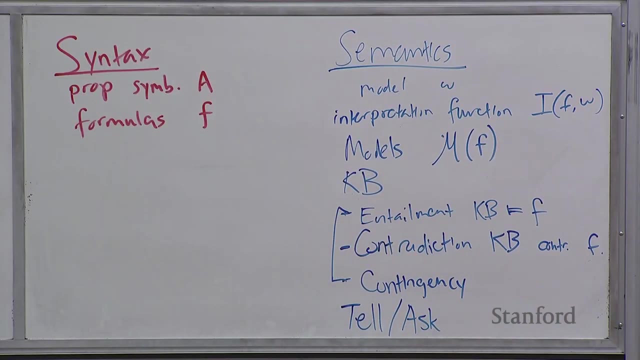 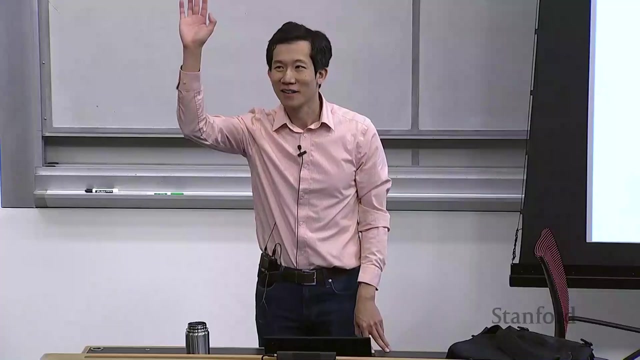 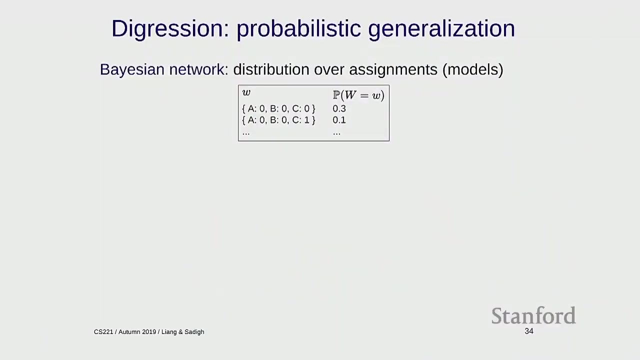 Okay, Okay, Any questions about this? Hmm, How many of you are following along? It's fine, Okay, good, All right. so this is a little bit of a digression And it's going to connect to uh Bayesian networks. 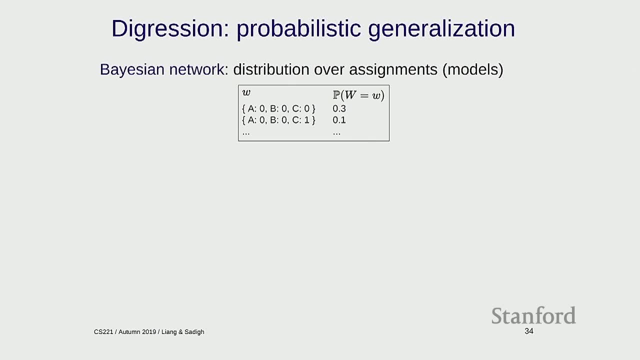 So you might be thinking in your head: well, we kind of did something like this already, right In Bayesian networks. we have these complete assignments and we actually define joint distributions over a complete assignment. That's the principle. now We don't really need to cut theAlgorithms tip. 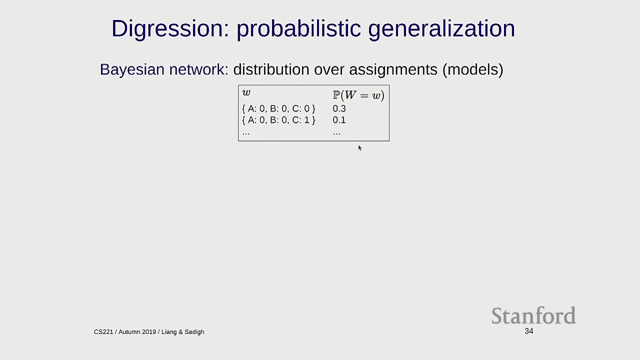 at that 1 or 2 hyphendetager. But even if you do, what do you do? is you just say, no, It's already something, that's all 3ifier for Bayesian networks, And and now, what we're talking about is not distributions. 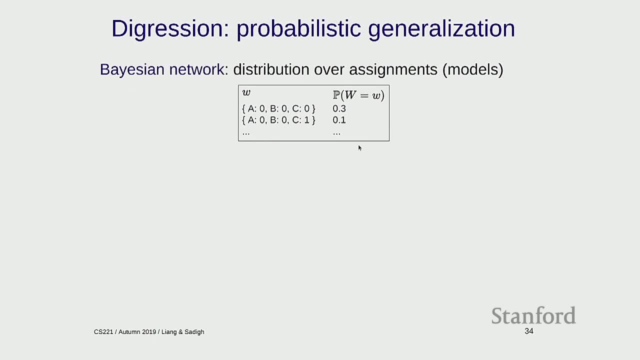 but sets of assignments or models, And so we can actually think about the relation between a knowledge base and an F also having an analog in Bayesian network land given by this formula. So, remember, a knowledge base is a set of models or possible worlds. 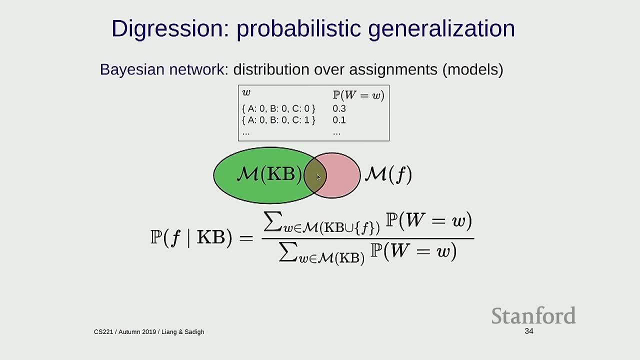 So in the probabilistic terms it is an event And that event has some probability. So that's, that's a denominator here, And when you look at F and KB and you intersect them, you get some other event which is a subset of that. 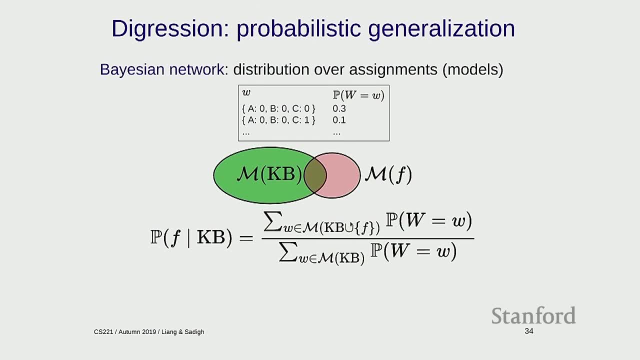 and you can ask for the probability mass of that intersected event. That's a numerator here And if you divide it, if you divide those, that actually just gives you the probability of a formula. uh, given the knowledge base, okay, 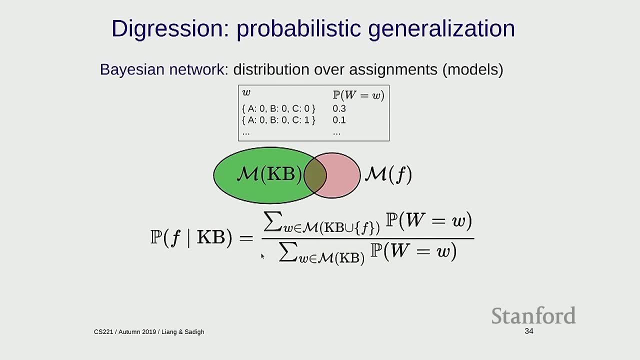 So this is actually a kind of pretty nice and direct um, um probabilistic generalization of, you know, propositional logic. Uh yeah, You have, like all of the all the variables required for that formula already exist in your set of worlds. 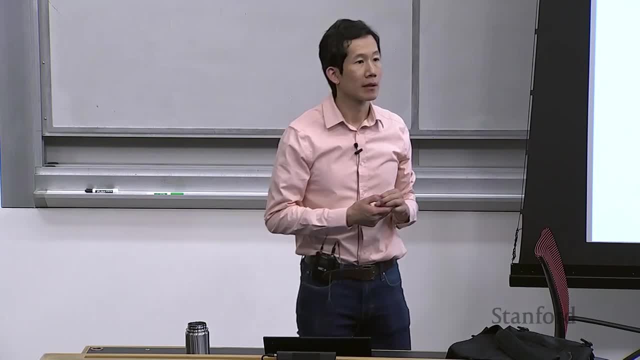 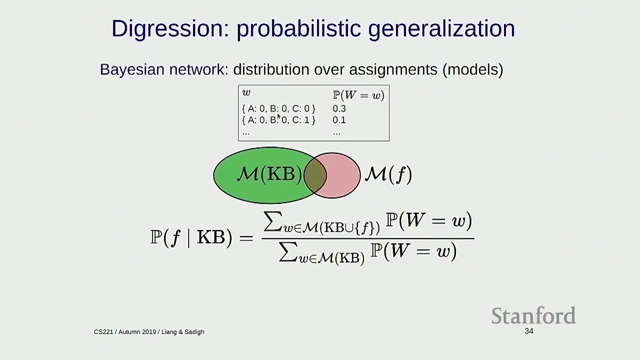 Like in this scenario, there's A, B, C. If we were asking something about D, it would still be an. I don't know because. because we don't have that information. Yeah, So the question is: this only works when restricted to the set of predefined? 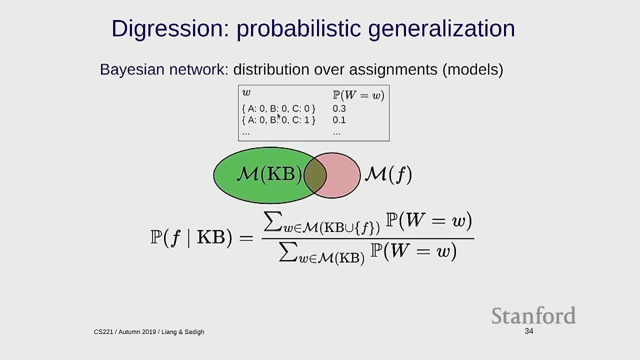 uh, propositional symbols, And you ask about D, then yeah, you would say I don't know, And it's in. in fact, when you define propositional logic, you have to pre-specify the set of symbols that you're dealing with. 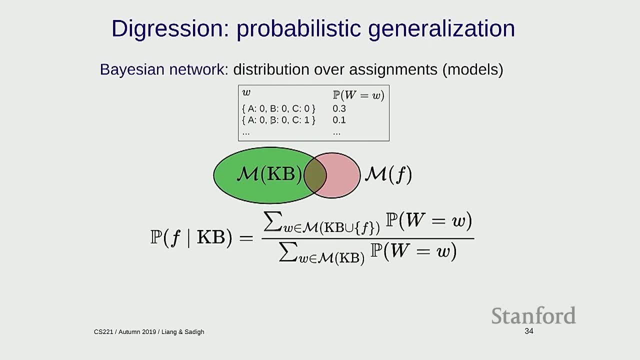 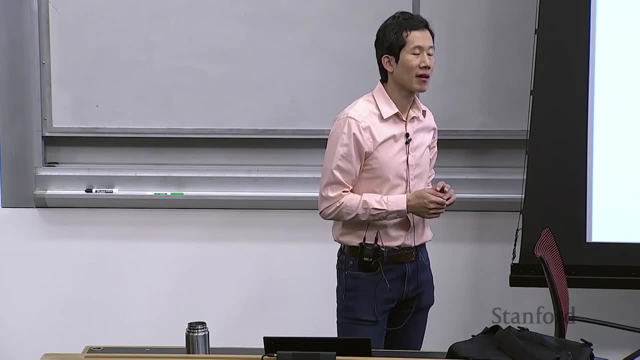 um, in in general, Yeah, In the example that we did earlier, like raining wasn't in the set of examples or things that our agent we knew about before we started, like training it, So is that something we'll get to later? 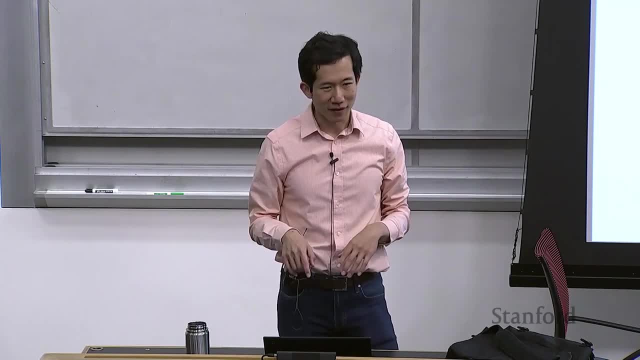 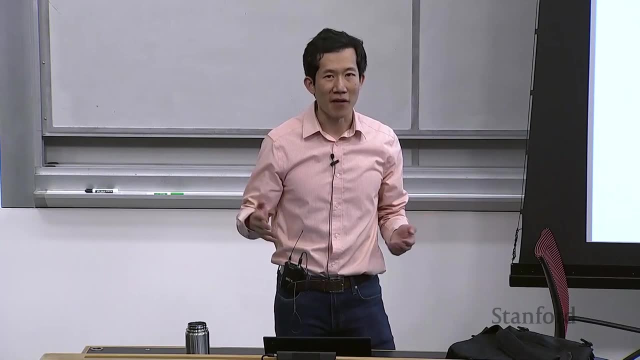 Um, yeah, So the question is in the, in the uh. in practice, you could imagine giving an agent like it is raining or it's snowing or sleeting and having novel concepts. Um, it is true that you can divide. 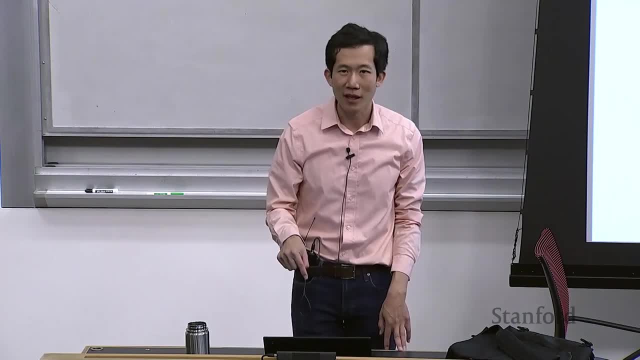 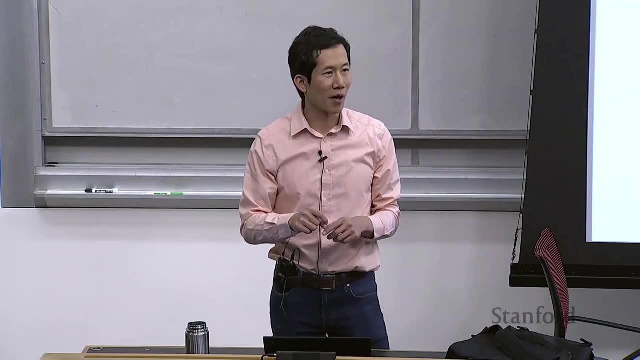 build systems, and the system I'm showing you has that capability. Um, um, and this is uh, it will be uh, it will be uh. it will be clear how we do that when we talk about inference rules, because that allows you to operate directly on the syntax. 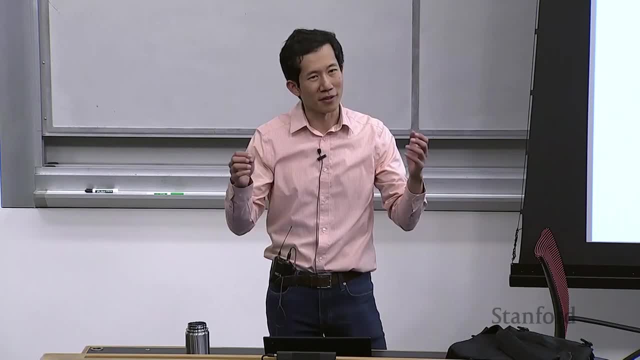 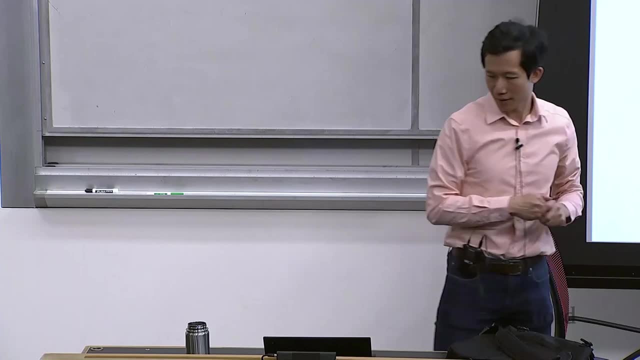 Um, here I'm talking about semantics, where you essentially just just for convenience- I mean you can be smarter- but but we're just defining the the world, Yeah, Yeah. So in this formula, why is this union and not intersection? 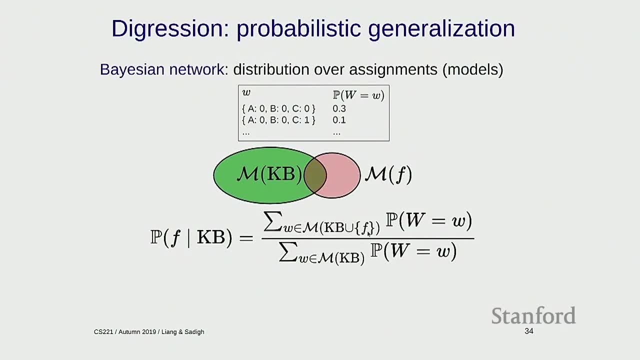 So I'm unioning the KB with a formula which is equivalent to intersecting the models of the KB with a model Because of the formula. Okay, So this is a number between 0 and 1. And this reduces actually to. 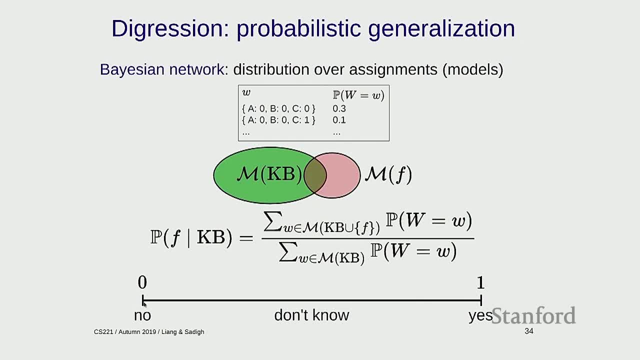 uh, the logical case if, if this probability of 0,, um, that means there's a contradiction, right, Because this intersection is- it's gonna be this prob- probability of 0. And if it's 1,, that means in its entailment. 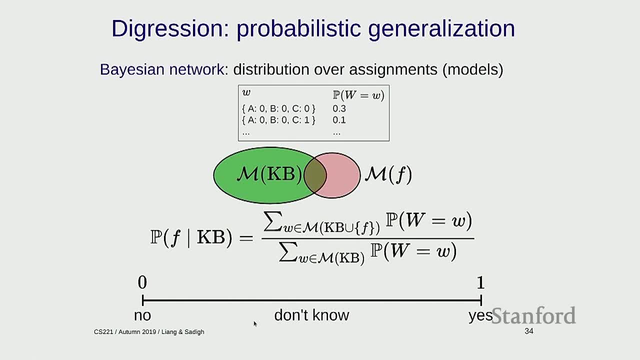 um, and the cool thing is that, instead of just saying I don't know, you can actually give a probabilistic estimate of like well, I don't know, but it's probably like 90%. Um, so you know. 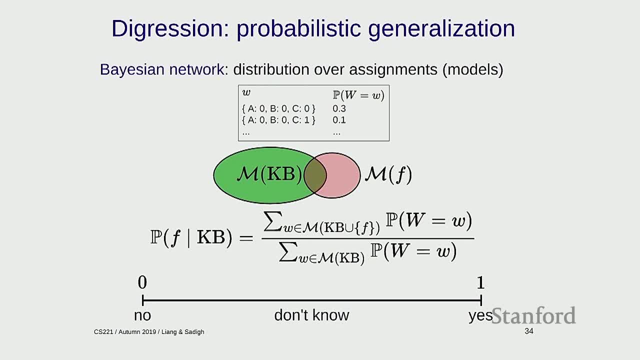 we're not gonna talk. uh, this is all I'm gonna say about probabilistic extensions to logic, but there are a bunch of other things um that you can do, that kind of marry the? um, the expressive power of logic, with some of the more advanced capability. uh, 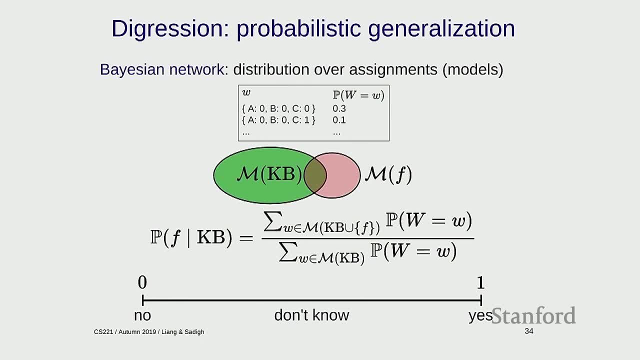 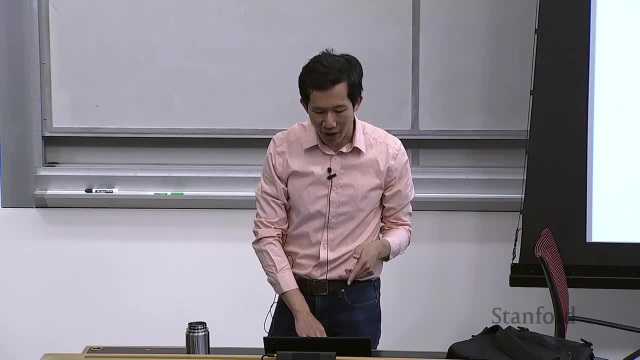 the ability of handling uncertainty of probabilities. Yeah, Are you assuming that we have the probability distribution? Yeah, To do this, you were assuming that we actually have the joint distribution at hand, And a separate problem is, of course, learning this. 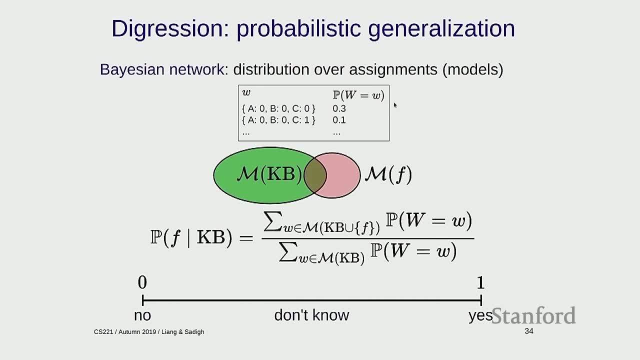 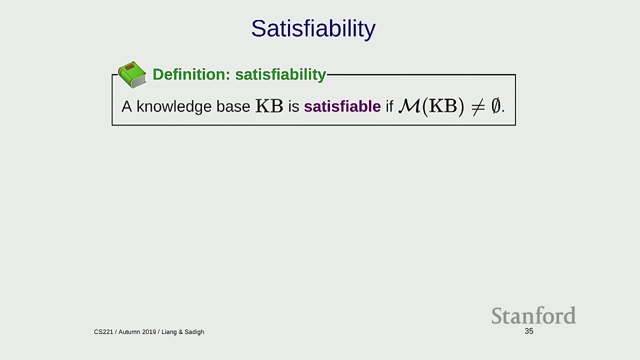 So for logic, I'm only talking about inference. I'm not gonna talk about learning, Although there are ways to actually infer logical expressions too, Okay. So back from the digression now. no probabilities anymore, We're just gonna talk about logic. 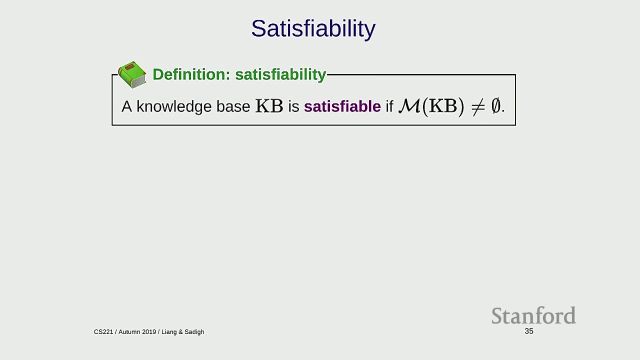 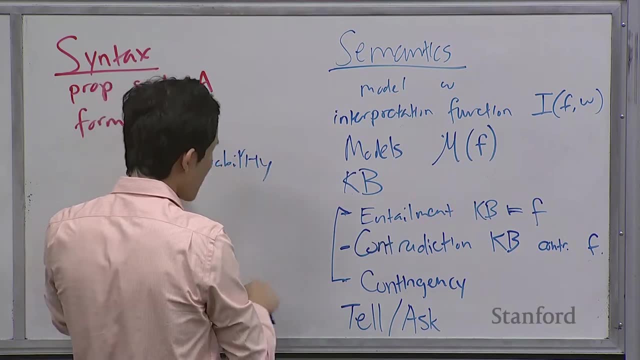 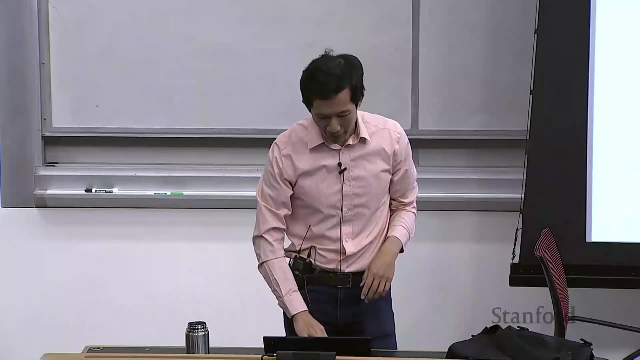 Um. there's another concept which is um really useful, called uh satisfiability, Um, and this is going to allow us to implement um entailment, contradiction, contingency, using kind of one, um primitive, And the definition is a knowledge base is. 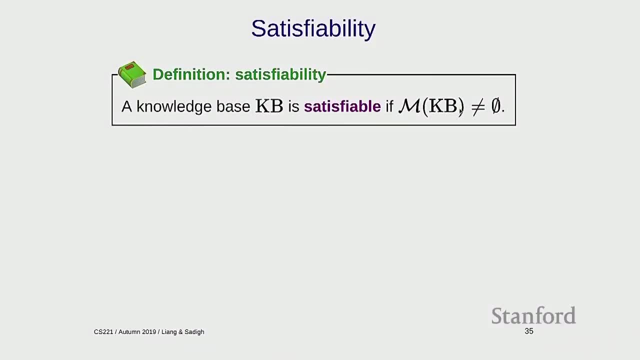 satisfiable if, um, the set of models is not Okay. So it's not self-contradictory, in other words, So now we can reduce ask-and-tell to satisfiability alone. Okay, Um, remember, ask-and-tell have three possible outcomes. 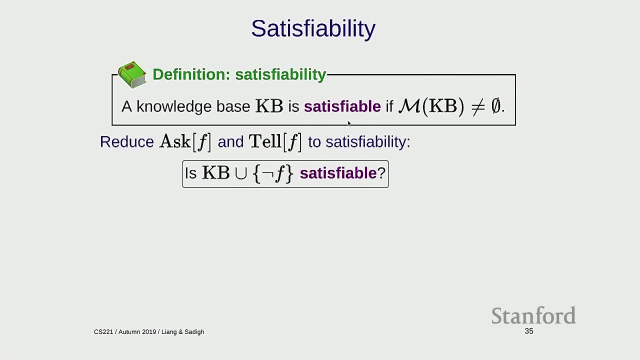 If I ask a satisfiable question, how many possible outcomes are there Two. So how am I gonna make this work? I have to probably call satisfiable twice. Okay, So let's start with asking if knowledge-based union- um, not F, is satisfiable or not. 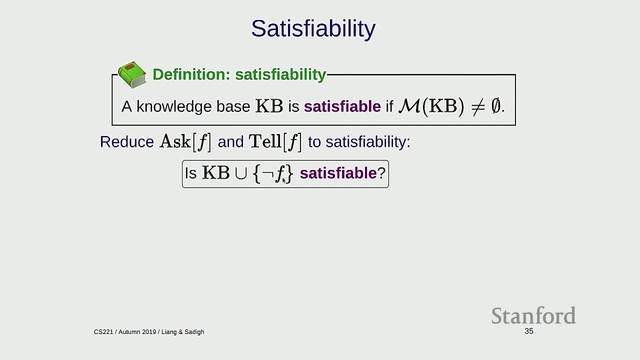 Okay. So if the answer is um, no, what can I conclude? So remember: the answer is no, So it's not satisfiable. Okay, So remember: the answer is no, So it's not satisfiable. Okay, So remember: the answer is no, So it's not satisfiable. Which means that KB contradicts, not F. 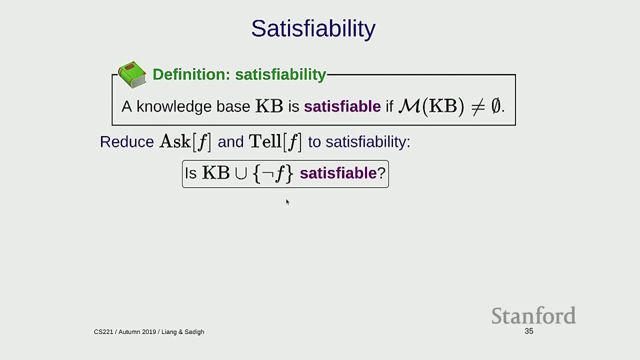 And what is that equivalent to saying Sorry, Like it's not F, like at that point, Um, yeah, So it's not F, So it's. which one of these is? should it be entailment, contradiction or contingency? 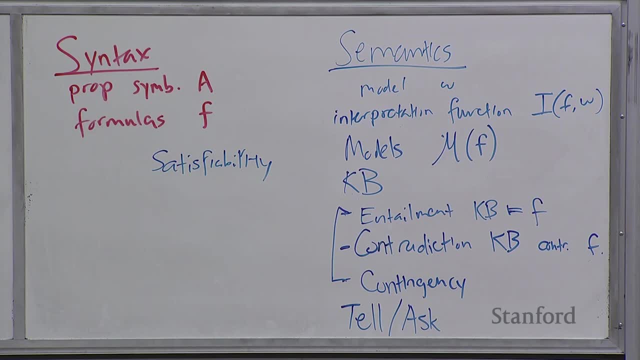 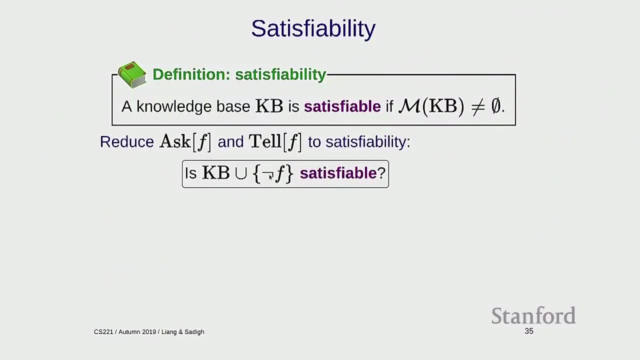 Mm-hmm, Yeah, So, um, I'm interested in the relation between KB and F. I'm asking the question about KB union, not F. Yeah, If F is already in KB. if you try to add not F, it's a contradiction because your at F and not F. 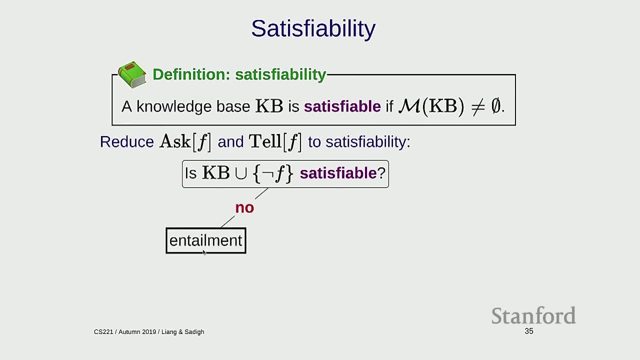 Yeah, Yeah, So exactly Okay. So this should be an entailment relation between KB and F. Remember, if KB entails f is equivalent to KB, contradicting you know F, not F. okay, Um, okay, So what about um? if it's yes? 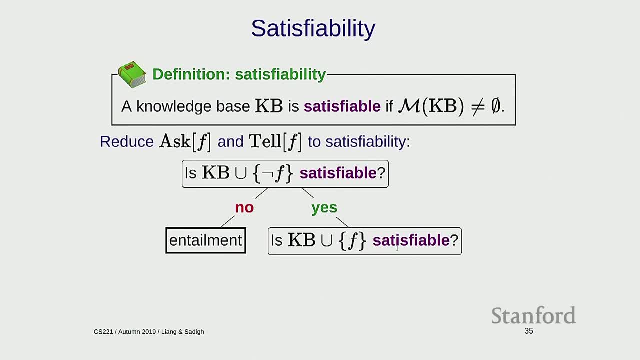 then I can ask another question: is KB union F satisfiable or not? So the answer is no, then what should I say? It should be a contradiction, because I mean this literally says KB contradicts F. And then finally, if it's yes, 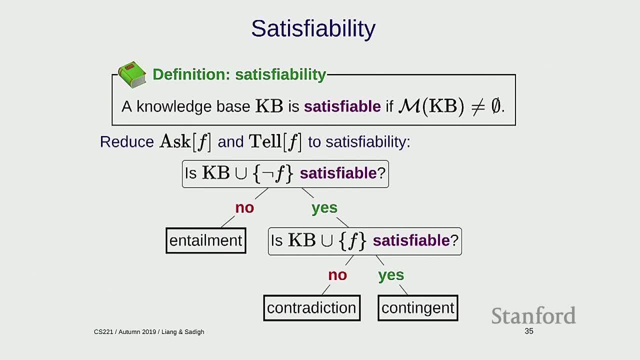 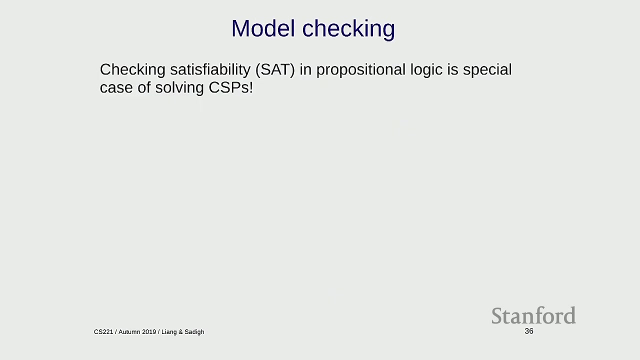 then it's contingency. okay. So this is a way in which you can reduce answering ask and tell, which is basically about assessing entailment, contradiction or contingency, to just two, at most two satisfiability calls. So why are we reducing things to satisfiability? 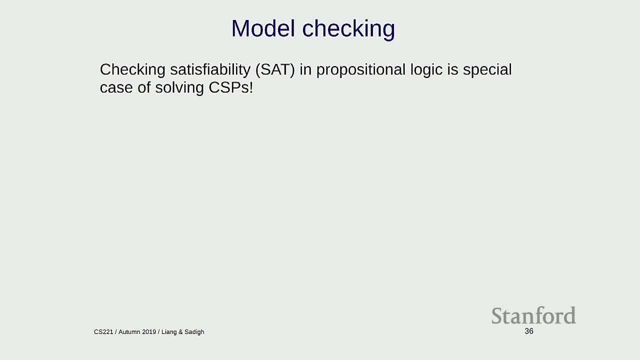 For propositional logics. checking satisfiability is just the classical SAT problem and it's actually a special case of solving constrained satisfaction problems. And the mapping here is: we just call propositional symbols, variables, um formulas, constraints, and we get an assignment here and we call that a model. 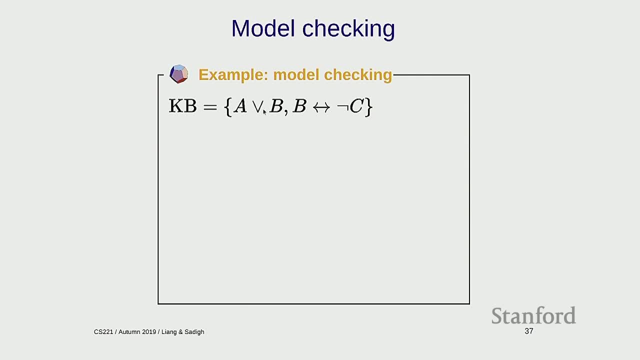 So in this case, if we have a knowledge base, um like this, then there are three variables, a, b and c, and we define this CSP and then we can um. if we find a satisfying assignment, then um, then we return satisfiable. 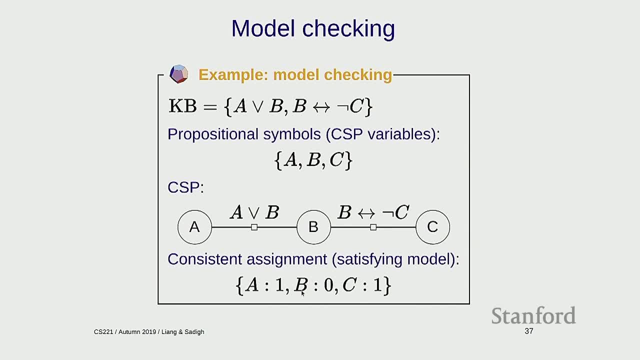 If we can't find one, then we return unsat. Okay, Um, so this is called model checking. Um, it's called um model checking because we're checking whether a model exists or is. uh, um is true. 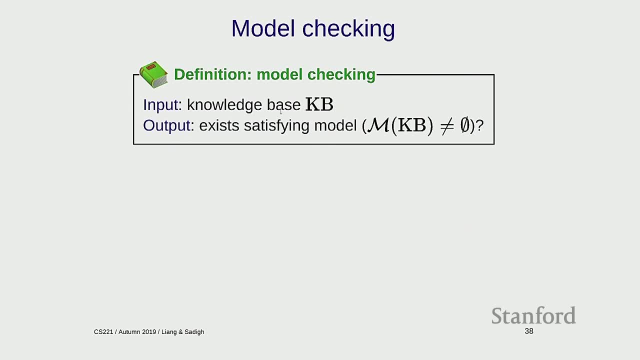 So you model checking takes a knowledge base and outputs whether there's a satisfying model. Um, there are a bunch of algorithms here which are, you know, very popular. There's something called DPL, named after, uh, four, four people. 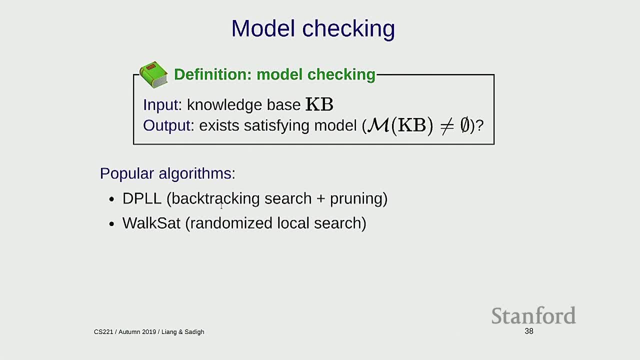 Um, and this is essentially backtracking, search, plus a pruning that takes into account the uh, the structure of your CSPs, um, which are propositional logic formulas. Um and uh, there's something called walk-set, which is: 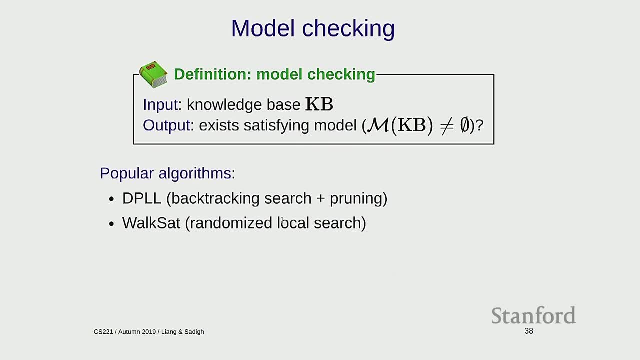 you can think about the closest analog that we've seen as, uh, Gibbs sampling, which is a, a randomized local search. Um, okay, So at this point you really can't have all the ingredients. you, uh, you need to do, um. 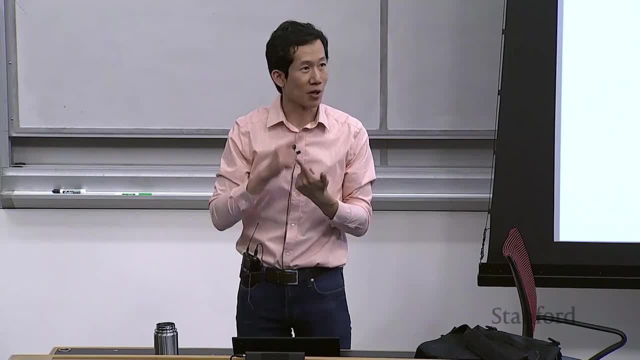 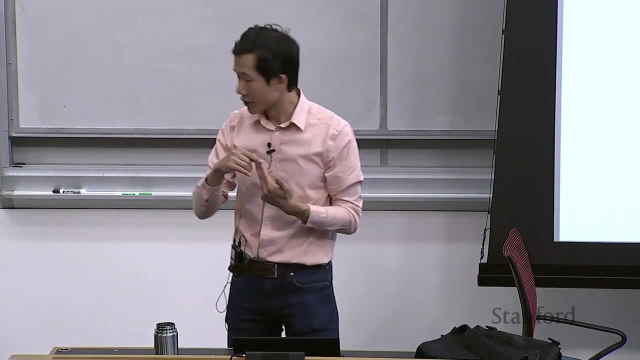 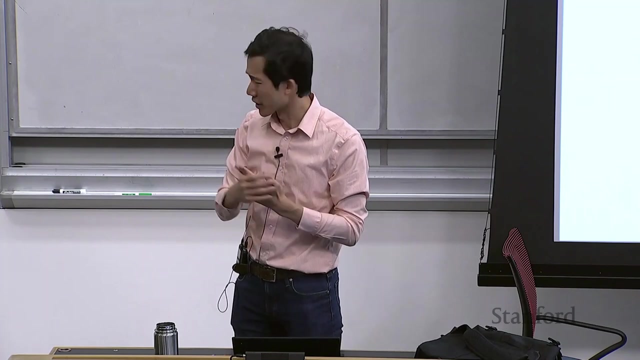 inference and propositional logic. So you define what propositional logic symbols are, Um or or formulas are. I define the semantics um, and I've told you even how to solve uh, entailment and um contradiction and contingency queries by reducing the satisfiability. 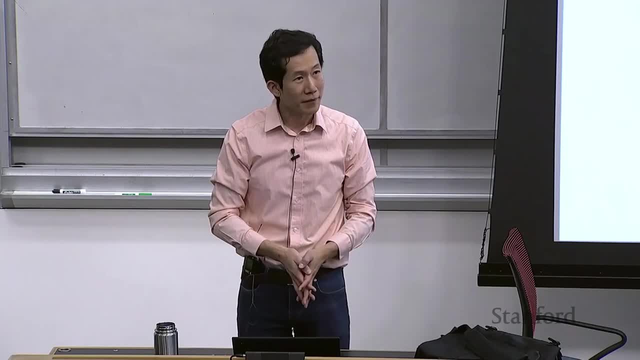 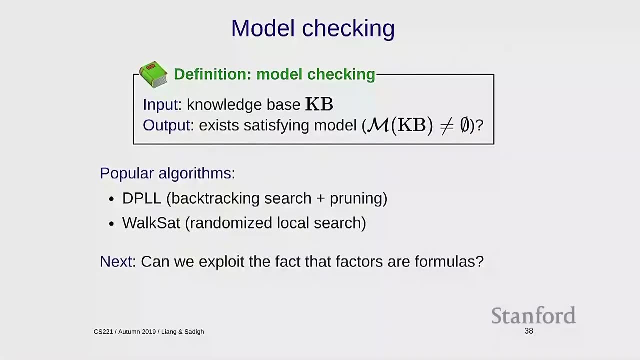 which is actually something we've already, you know, seen, coincidentally, Um. so that should be it, Okay, Um, but now coming back to the- you know, original motivation of x1 plus x2, equals 10, and how we were able to perform that logical query much faster. 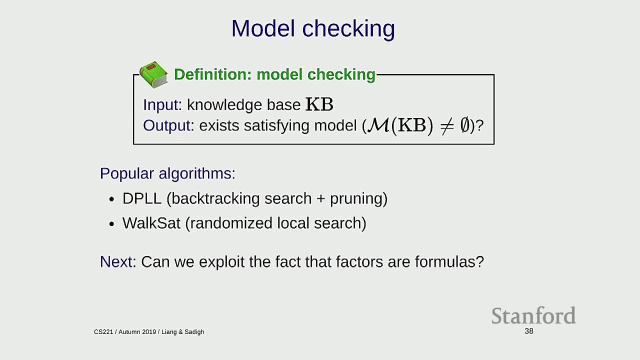 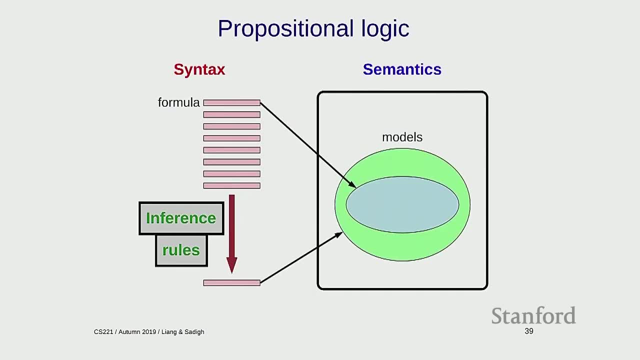 We can ask the question now: can we exploit that the factors are? are formulas rather than arbitrary, you know, functions, And this is where inference rules is gonna come into play, Okay, So, um, so I'll try to explain this. 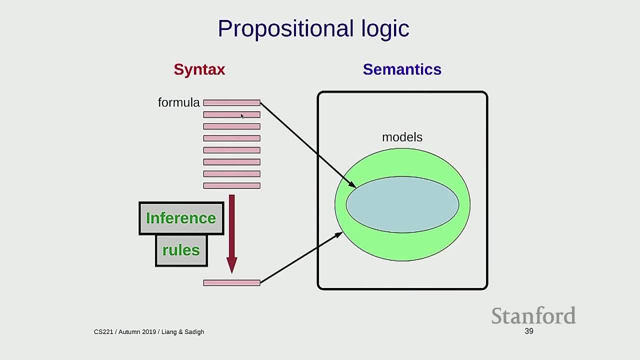 uh, figure a little bit, since it was probably pretty mysterious um from the beginning. So I have a bunch of formulas. This is my knowledge base. Over time I accrue formulas And these formulas carve out um a set of models in semantics land. 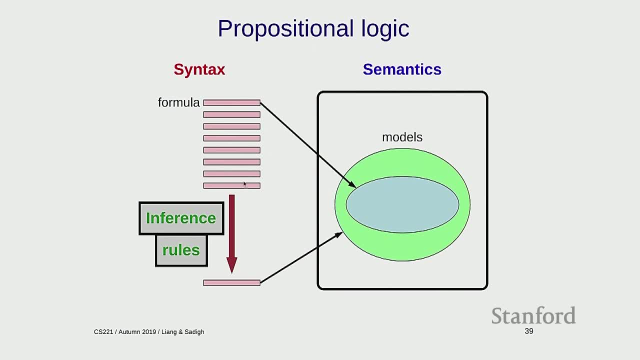 And and this formula here. if it's um a superset, that means it's entailed by these formulas, right? So I know that this is true, given my knowledge, which means that this is kind of a logical consequence of. 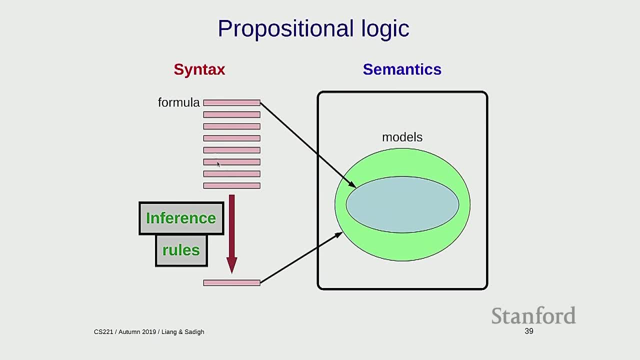 of what I know. okay, So so far, what we've talked about is taking formulas and doing everything over in semantics land. What I'm gonna talk about now is inference rules that are gonna allow us to directly operate on the syntax and hopefully get. 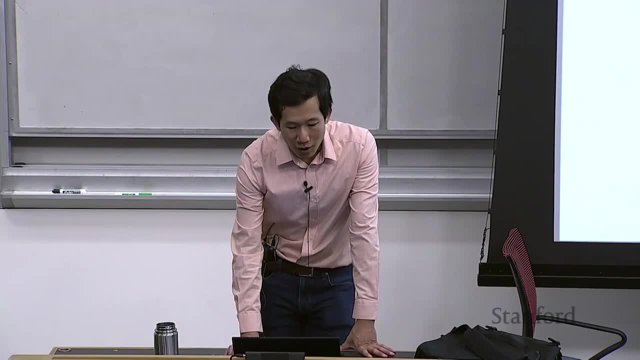 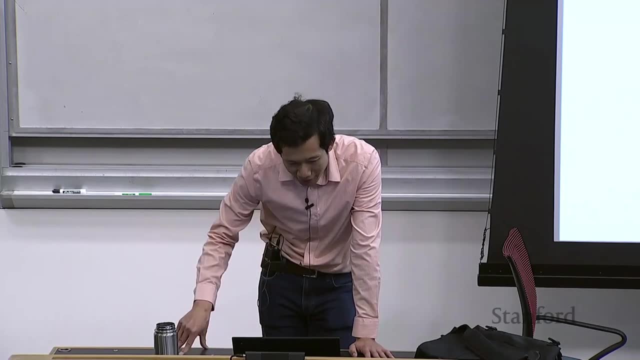 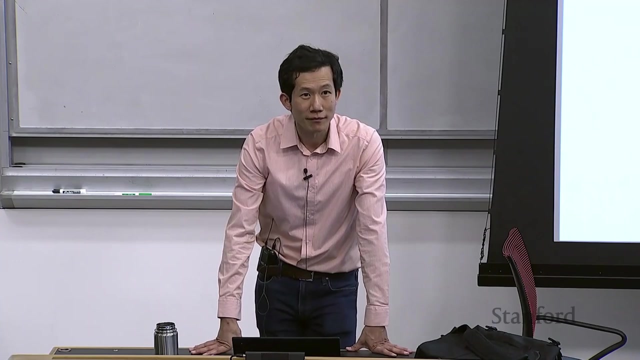 um, some results that way. Okay. So here is an example of making an inference. Um, so if I say it is raining and I tell you, if it's raining, it's wet- Um, rain implies wet- then what should you be able to conclude? 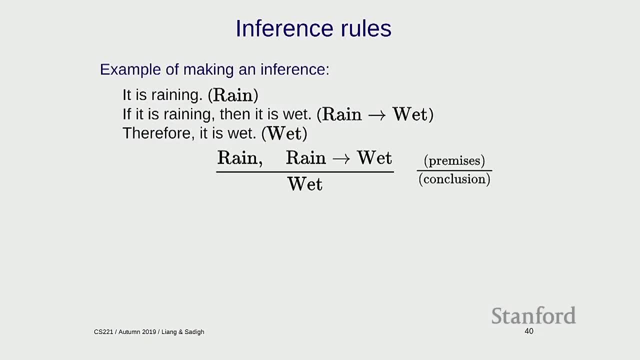 It's wet, right? So I'm gonna write this inference rule this way, with this um kind of fraction looking like thing, where there's a set of premises, which is a set of formulas which I know to be true, And if those things are true, 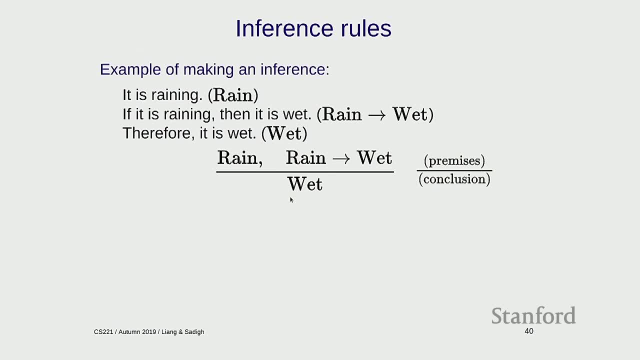 then I can derive a conclusion, which is another formula. This is um um, an instance of a general rule called modus ponens Um. this says for any propositional symbols p and q. if I have p and p implies q in my knowledge base. 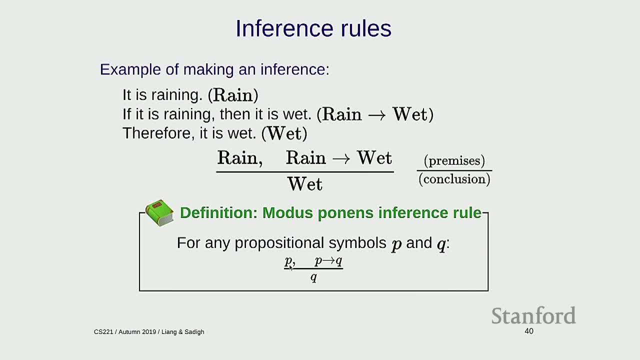 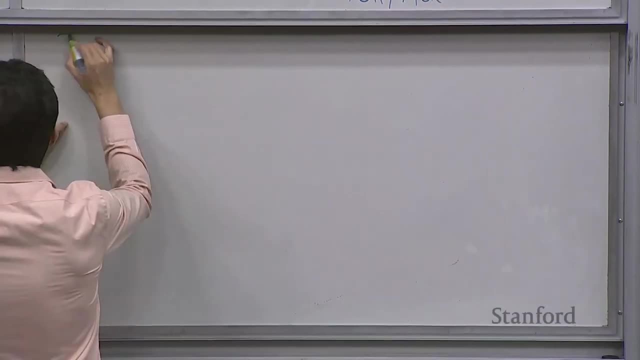 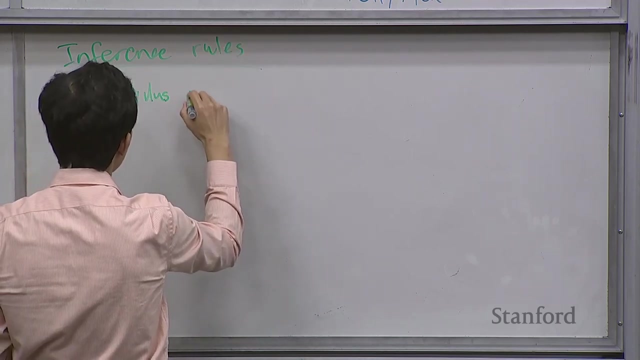 then I can- that entails uh, q. Okay, So let's talk about inference rules. Um, inference- Actually, let me do it over here, since I'm gonna run out of space otherwise. Okay, So modus ponens is the first thing I'm gonna talk about. 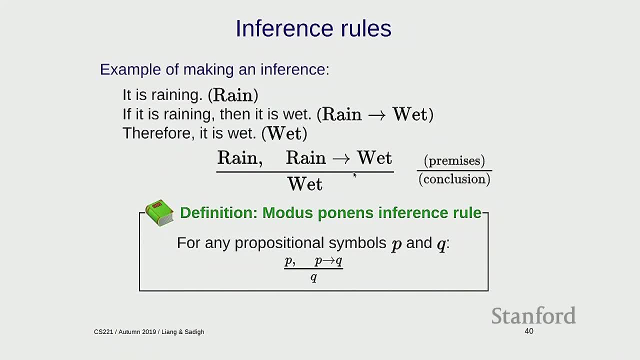 Um, so notice here that if I could do these type of inferences, it's much less work, right, Because I- it's very localized. All I have to do is look at these three formulas. I don't have to care about all the other ones. 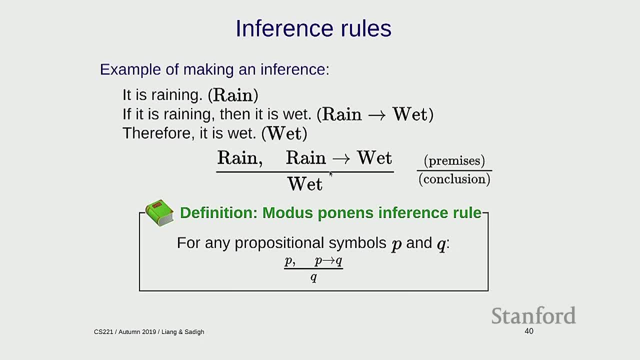 formulas or propositional symbols that exist. And going back to this question over here about oh how do I? what happens if I have new concepts that occur? Well, you can just treat everything as just a new symbol. There's not necessarily a fixed set of symbols that you're working with at any given time. 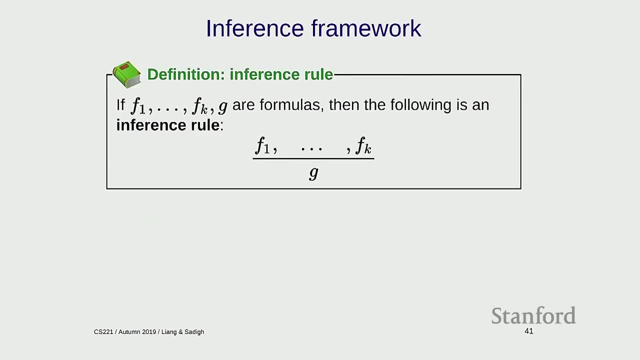 Okay, So this is the example of the inference rule In general. the idea of the inference rule is that you have rules that say, if I see F1 through Fk, which are formulas, then I can add G, Um, and the key idea, as I mentioned before, is that these inference rules operate. 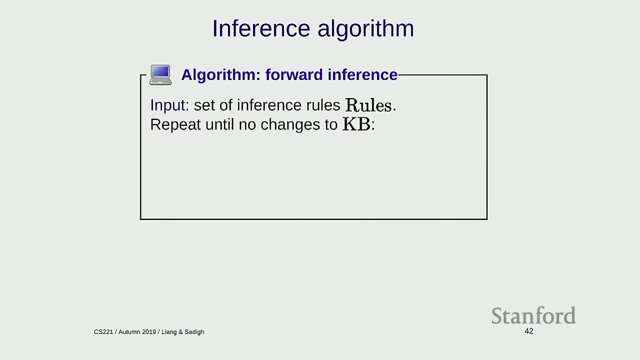 directly on the syntax and not on the semantics. So, given a bunch of inference rules, I have this um kind of meta-algorithm that can do a logical inference as follows. So I have a set of inference rules and I'm just going to repeat. 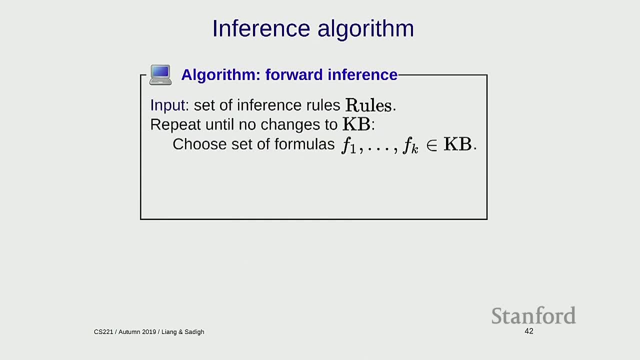 until there's no changes to a knowledge base, I choose a set of formulas from the knowledge base: Um. if I find a matching rule inside rules that exists, then I simply add G to the knowledge base. Okay, Um, so what the other definition? 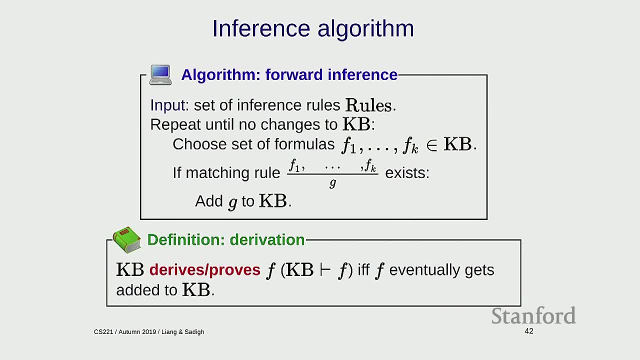 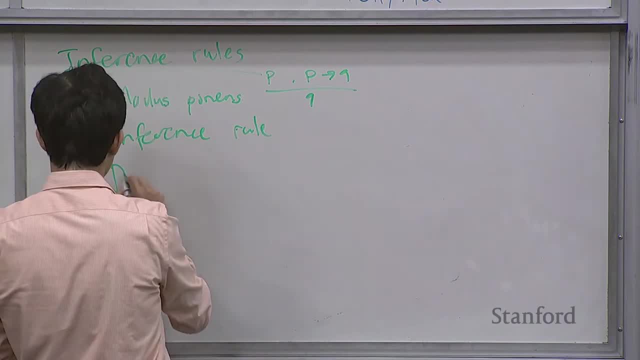 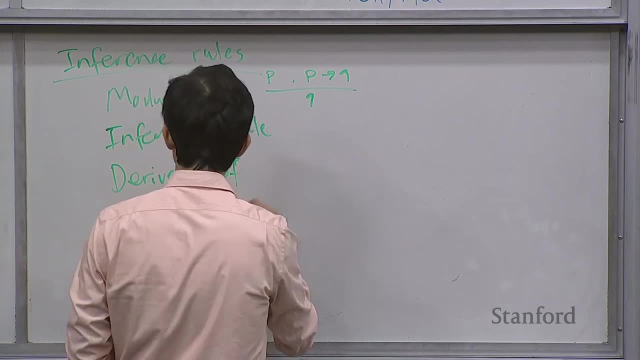 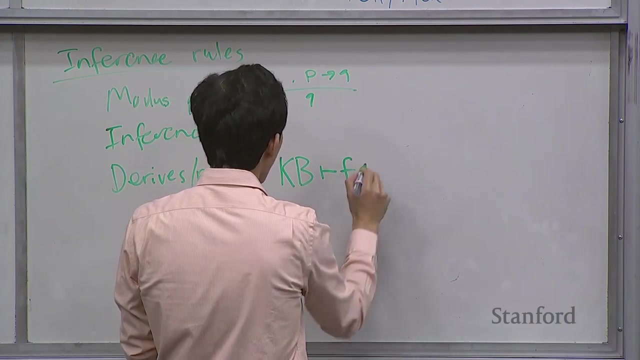 I'm gonna make is this idea of derives and proves. So um inference Rule: um, derives, proves, Um. so I'm gonna write Kb and now with a single horizontal line, um to mean that from this knowledge base, 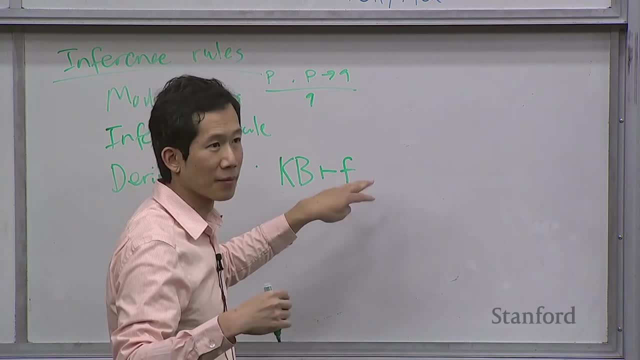 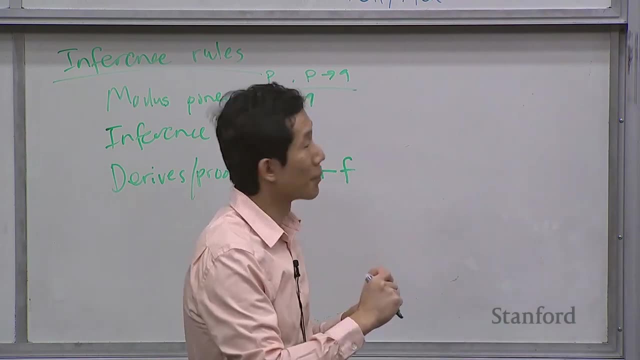 given a set of inference rules, I can produce F via the rules. Okay, This is in contrast to entailment, which is defined by the relationship between the models of Kb and the models of F. Now, this is just a function of mechanically applying a set of rules. 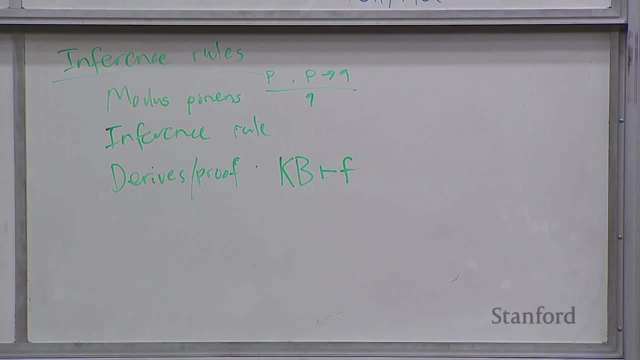 Okay. So that's a very, very important distinction. And if you think about it, why is it called proof? So, whenever you do a mathematical proof or some sort of logical argument, you're in sense- in some sense- just doing logical inference. 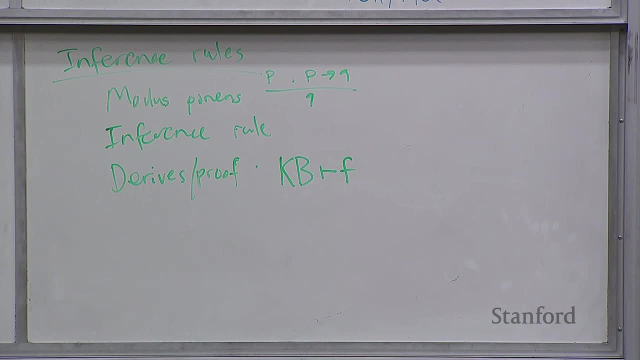 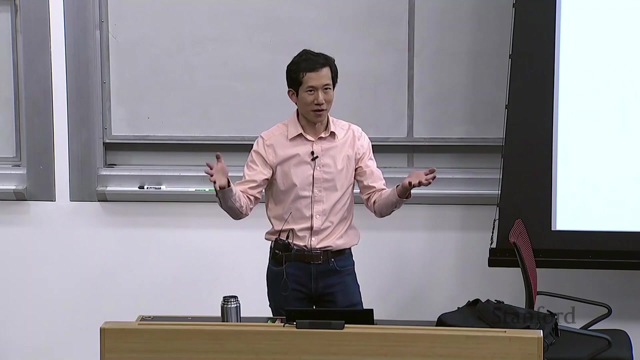 where you have some premises, and then you can apply some rule. uh, for example, you can add um, you know, multiply both sides of the equation by 2. That's a rule. You can apply it, um, and you get some other equation which you can. 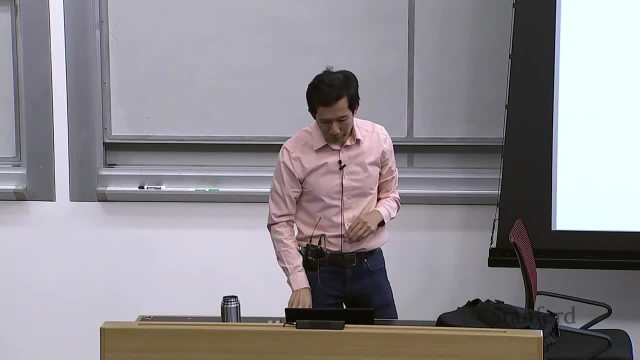 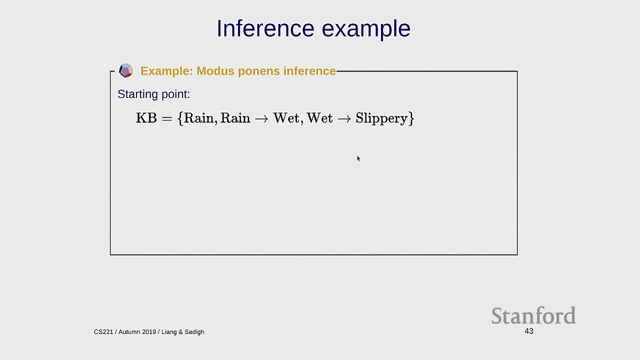 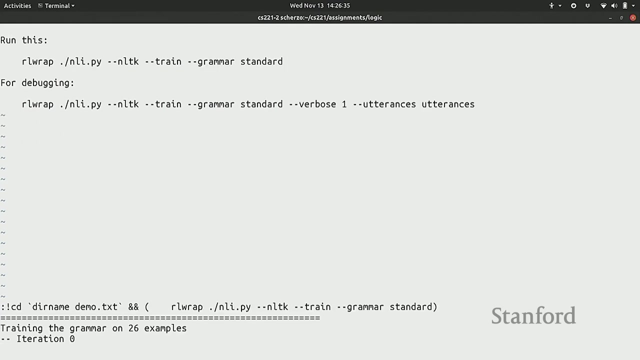 um, which you hope is true as well. Okay, So here's an example: Um, maybe I'll, just for fun, I'll do it over here. Um, oops, So I can say it is raining, And if I dump that? 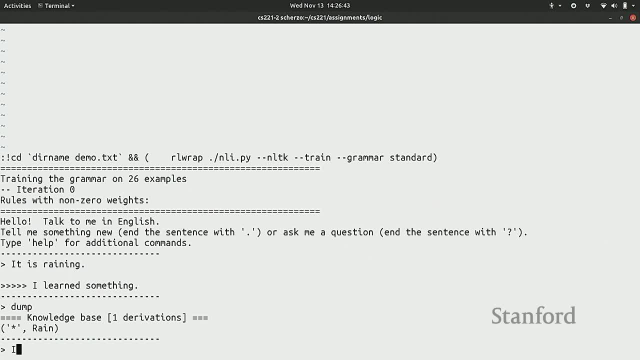 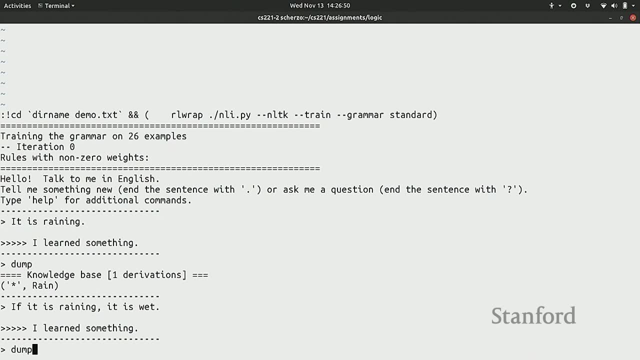 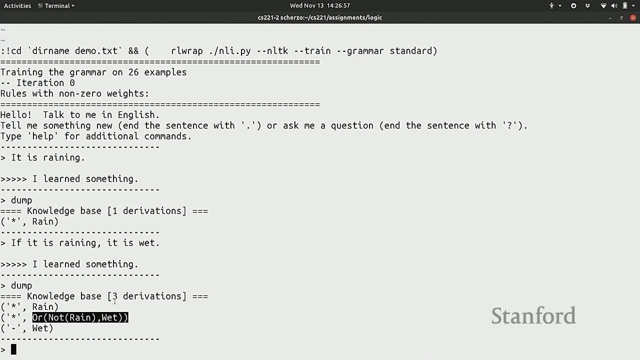 it gives me, uh, my knowledge base. it has rain, Um. if it is raining, it is wet, Um. so if I dump, then I have. this is the same as um. rain implies wet. Okay, Just-, just-, just to- in case you're rusty on your propositional logic. 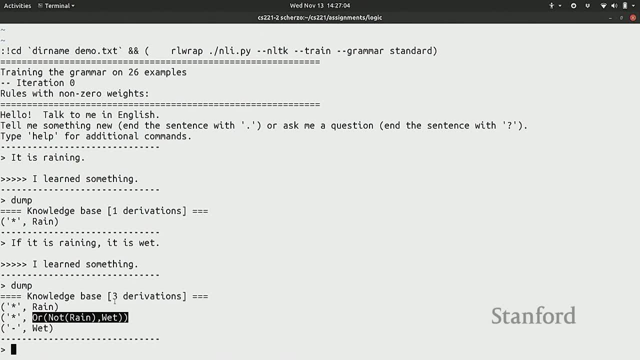 if I have P implies Q. that's the same as not P or Q. Okay, And notice that I have also wet appearing in my knowledge base, because this uh in the background, it's basically running forward inference to um. try to derive as many conclusions as it can. 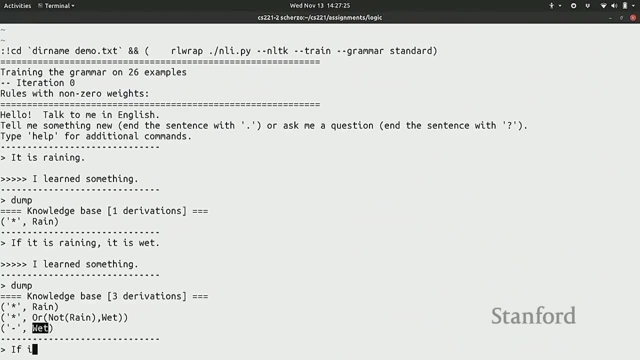 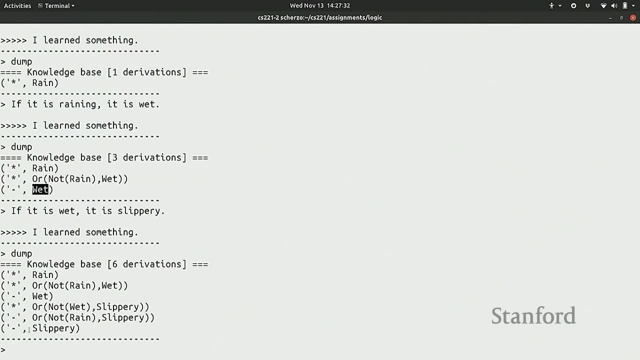 Okay, Um. and if I say if it is wet, it is uh slippery Um, again, now I have um, I have uh. wet implies slippery um, and now I also derive slippery Um, I also derive rain um. 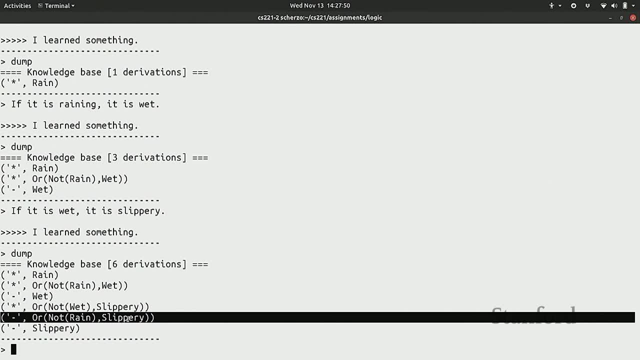 implies slippery, which is actually, as you'll see, not derivable from modus ponens. So behind the scenes is actually a much more- uh, fancy inference algorithm. But um, but-. but the idea here is that you have your knowledge base um, you can pick. 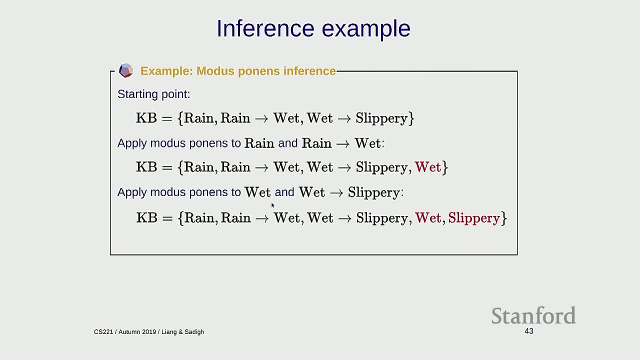 pick up rain, and rain implies wet, and then you can add wet, and then you pick up ra- wet, wet implies slippery, and then you can add slippery here, And with modus ponens, um, you can't actually derive some things. 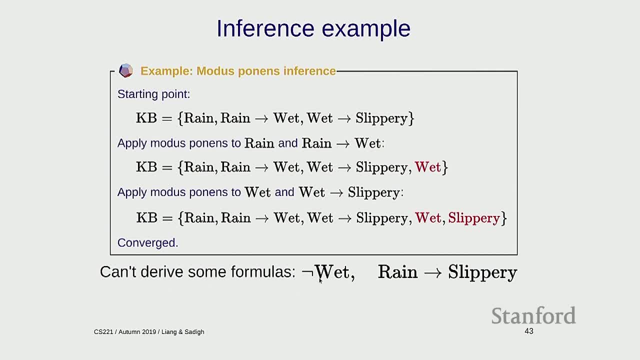 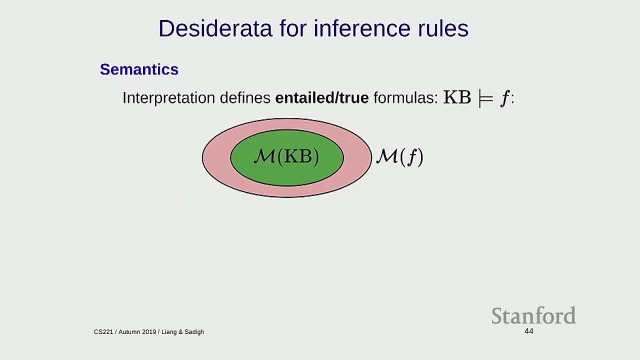 You can't derive- not wet, um, which is probably good, because that's not true- And you also can't derive. rain implies slippery, which actually is true, but a modus ponens is not powerful enough to derive it. Okay, So- so the burning question you should have in your head is: 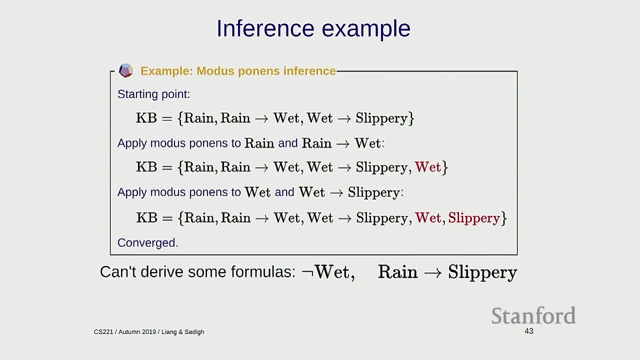 okay, I talked about there's two relations between a knowledge base, KB- and a formula F. There is entailment relation, And this is really what you want, because this is semantics- You- you care about meaning, Um, and you also have this, uh. 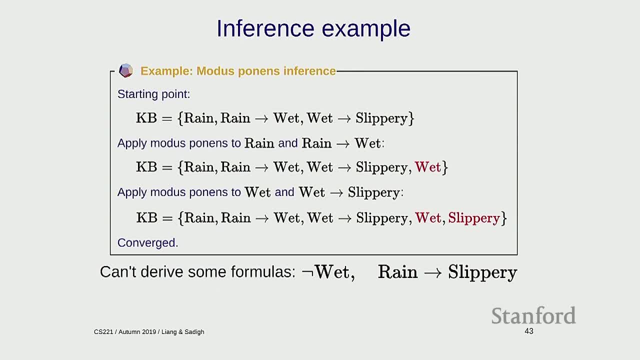 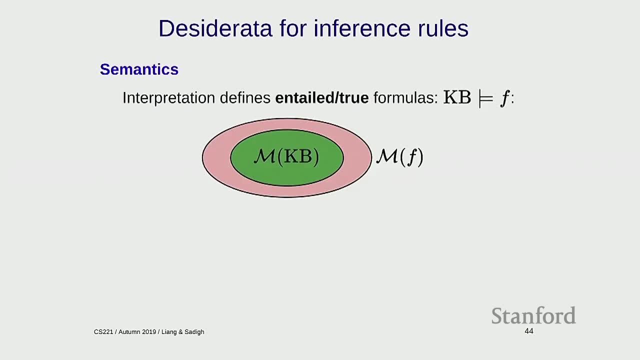 KB derives F, which is a syntactic um relationship. So what's the connection here? In general, there's no connection um, but there's a kind of uh, these concepts that will help us think about the connection. So the semantics, these are things which are um. 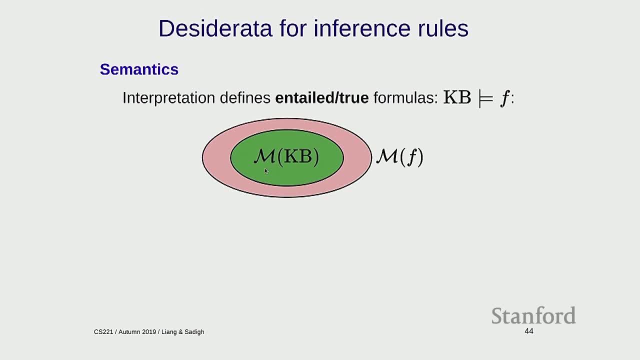 when you look at semantics, you should think about the models implied by the um, the formulas And syntax is just some set of rules that someone made up, Okay, So how do these relate? Okay, So to um. understand this. 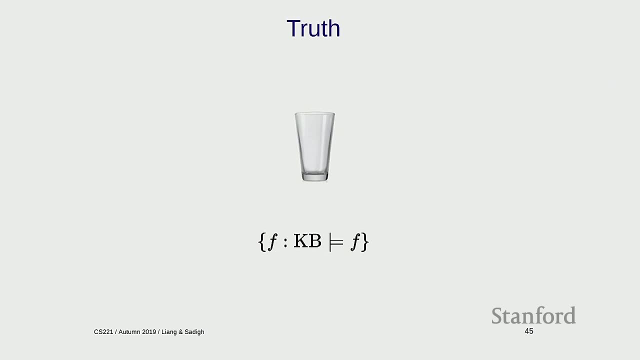 imagine you have a glass and this glass is um, um. what's inside the glass is a formulas And, in particular, it's the formulas which are true. Okay, So this glass is all formulas, such that the- this formula is entailed by the knowledge base. 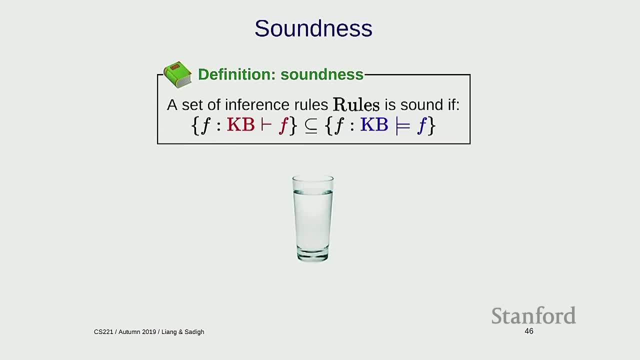 So, um, soundness is a property of a set of rules And it says: if I apply these rules until the end of time, do I stay within the glass? Am I always going to generate formulas which are inside the glass, which are semantically you know? 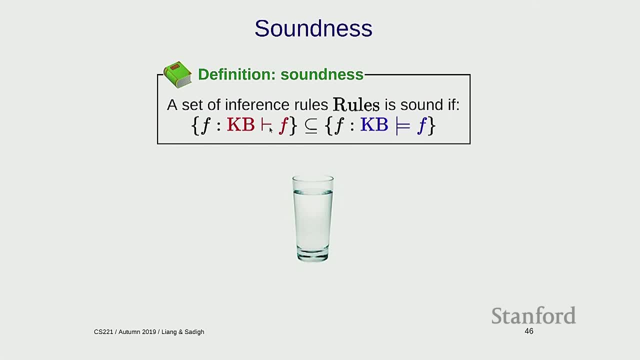 valid or entailed. Okay, So soundness is good, Um, completeness says the- the kind of uh, um. the other direction, which says that I am going to generate all the formulas which are true or entailed, I might generate extra stuff. 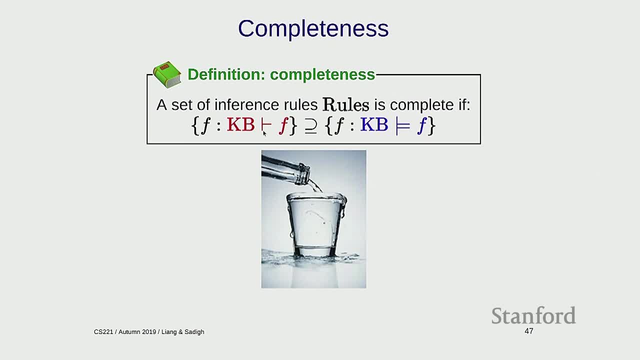 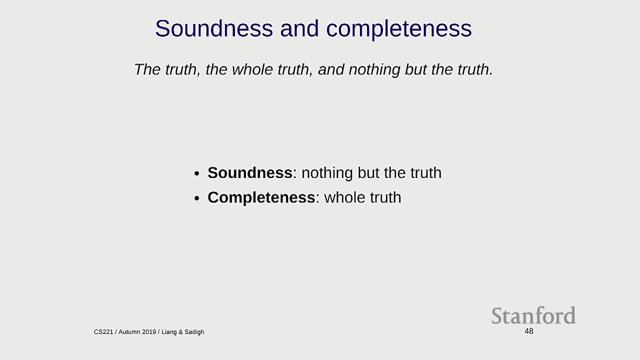 but at least I'll cover everything. That's what it means to be complete. Okay, So the model you should have in your head is: you want the truth, the whole truth and nothing but the truth. Soundness is really about nothing but the truth. 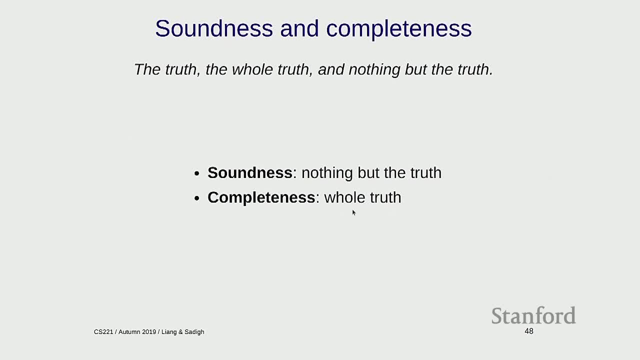 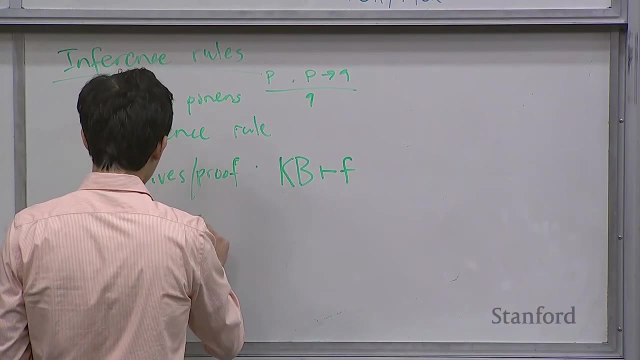 and completeness is about the whole truth. Ideally, you would want both. Sometimes you can't have both, so you're gonna have to pick your battles, Um, but generally you want soundness. Um, you can maybe live without completeness. 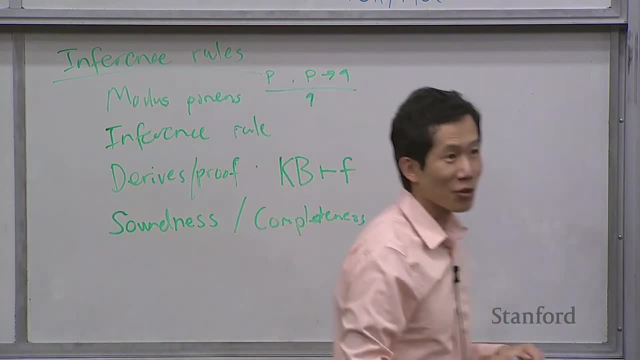 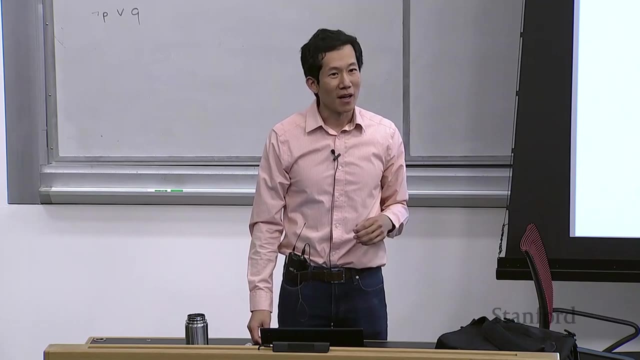 Um, but if you're unsound, that means you're just going to generate erroneous conclusions, which is uh bad, Whereas if you're incomplete, then maybe you just can't uh infer certain notions, but at least you- the things that you do infer- 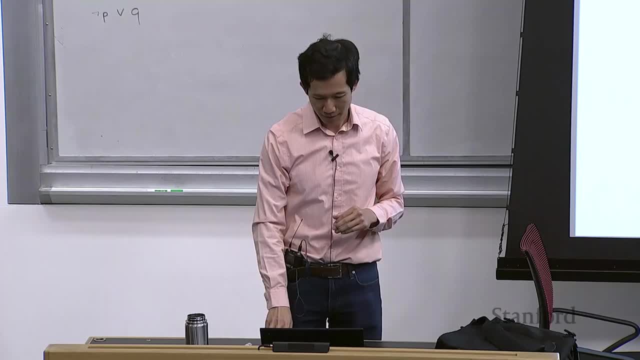 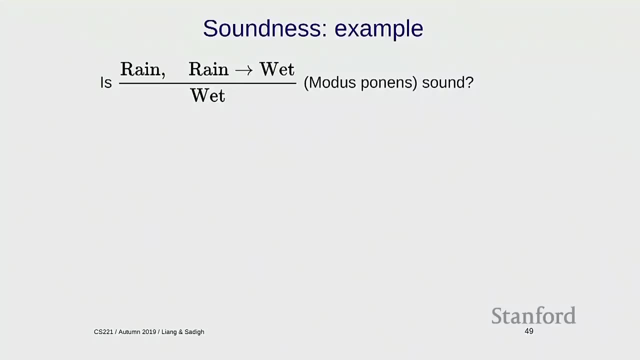 you know are actually true. Okay, So how do we check um soundness? So is modus ponens sound, Um, so remember, uh, there- there's kind of a rigorous way to do this, And the rigorous way is to look at two formulas. 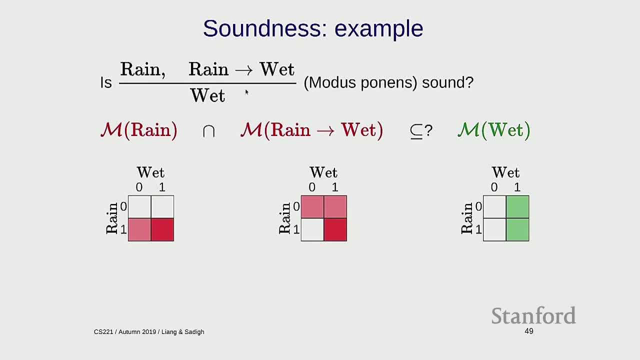 Rain, rain, uh implies what Um? and then look at their models. Okay, So rain corresponds to these set of models, here, Um, rain implies what Corresponds to this set, Um, and when I intersect them, that's the- the set of models which are conveyed by the knowledge base. 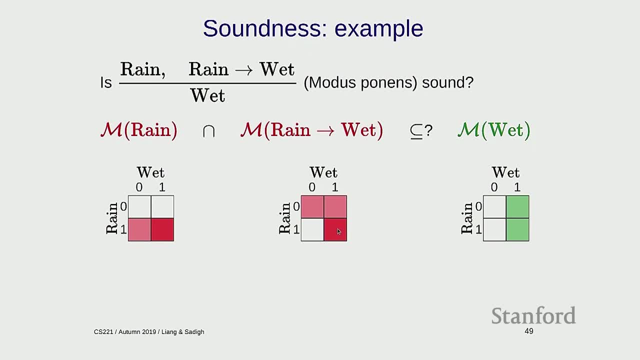 which is this corner here. Um- and I have to check whether that is a s- a subset of the models of wet And wet is over here. So this 1, 1 corner is a subset of 1, 1, and 0, 1.. 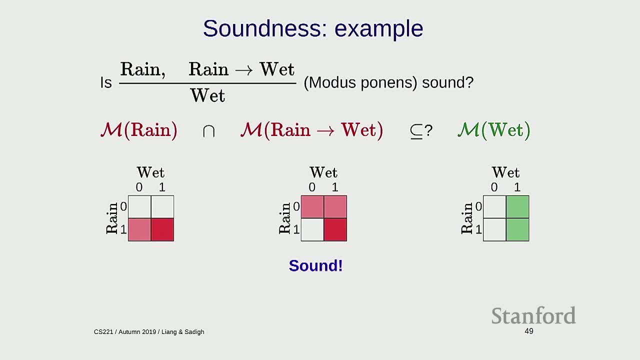 So this um rule is sound. Remember this. why is this subset the thing I want to check? Because that's the- just the definition of entailment, Right, Okay? So let's do another example. So if someone said it was wet and you know that rain implies wet, 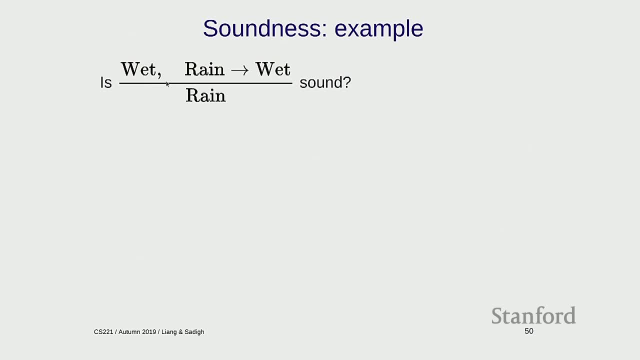 can you infer rain? Well, let's- let's, uh, let's just double-check this, Okay. So again, what are the models of wet? They're here. What is the models of rain implies wet? They're here. 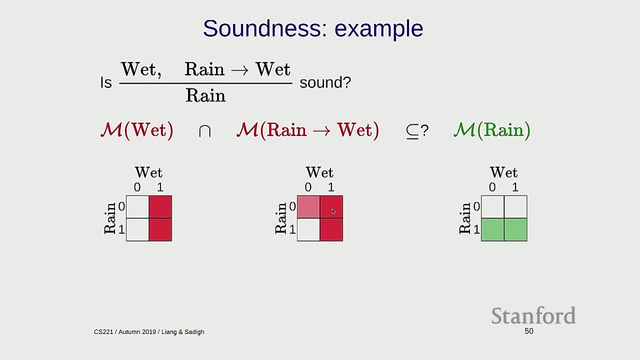 And I intersect them. I get this, um, this- these two over here in dark red, And then is that a subset of models of rain. Nope, So this is unsound. Okay, So in general, soundness is actually a fairly 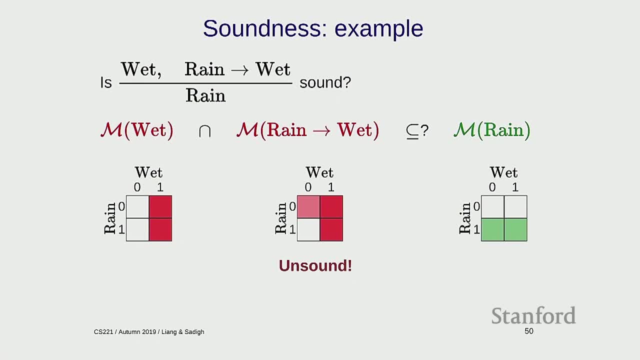 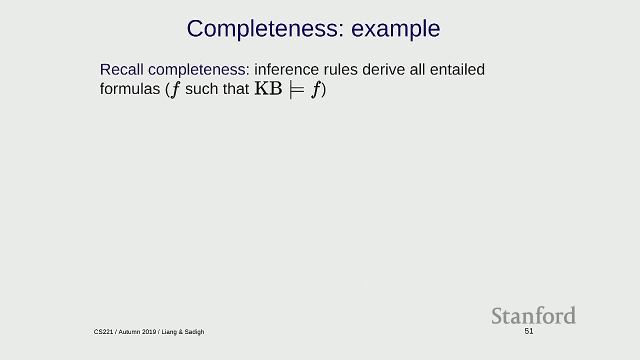 uh, easy condition to check, especially in propositional logic, but in higher order logics it's, you know, not as bad. So now completeness is a kind of a different story which I'm not gonna have time to um. 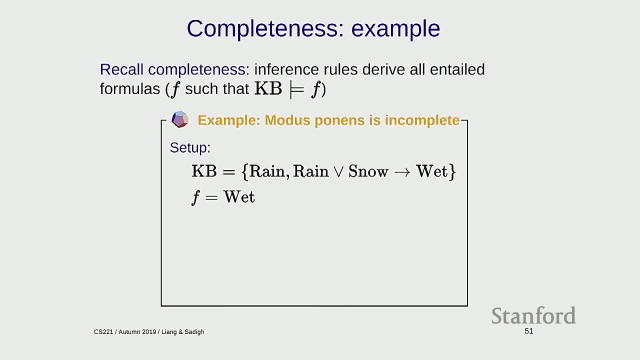 to really do full justice in this class. But, um, but here's a kind of a uh example showing modus ponens is um incomplete, So um, uh, for propositional logic, Um. so here we have the knowledge base: rain. 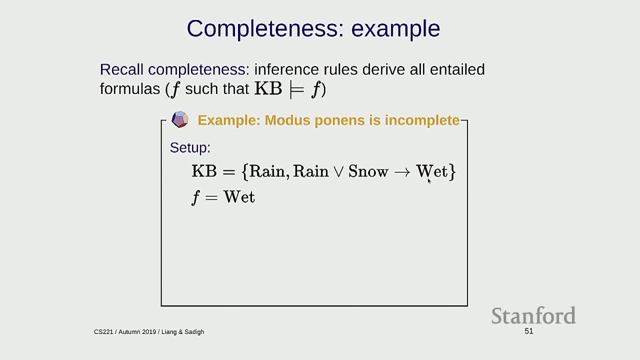 rain or snow implies wet, um and um. is this entailed wet? So it's raining, and if I know it's raining or snowing, then it should be wet. How many of you say yes, Yeah, it should be entailed, right. 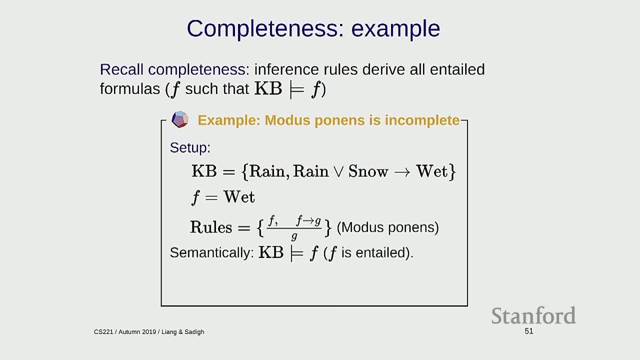 Okay, But what does modus ponens do? Well, all the rules look like this: Um So um. clearly, you can't actually arrive at this with modus ponens, because modus ponens can't reason about ore or disjunction. Yeah, 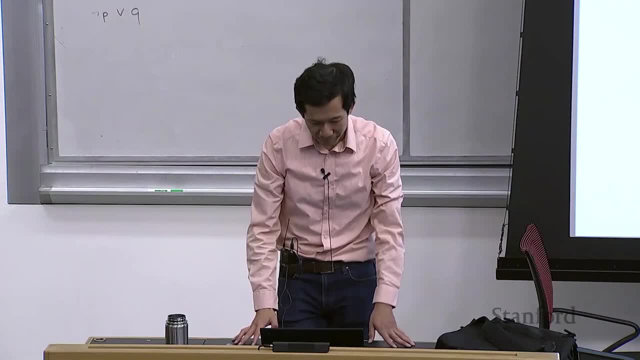 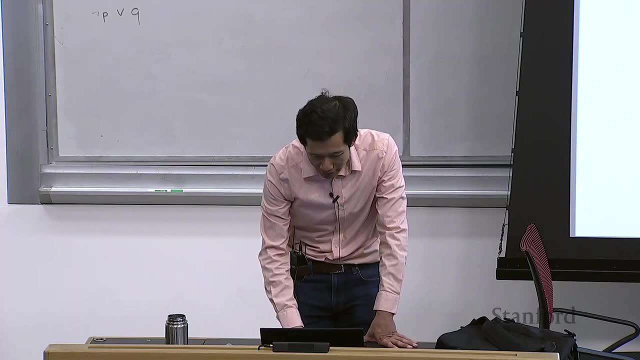 Is that the rain or snow? I guess it's saying that it's not possible for it to be not wet, given rain. Um, is it not? Yeah, because you're- you already know that it's raining, So you should say that that's why. 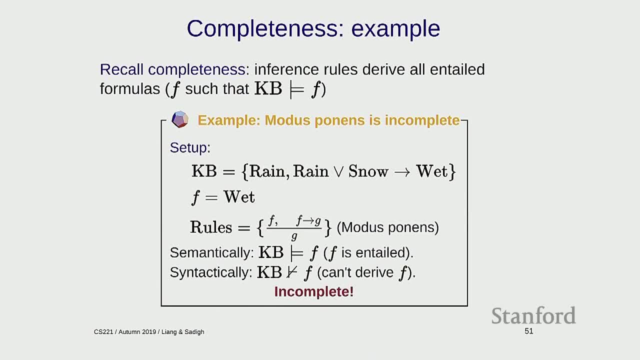 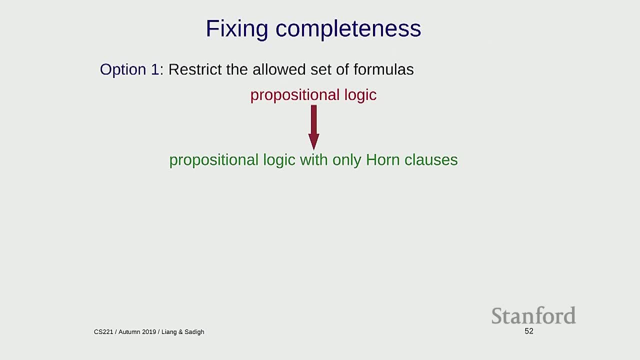 Yeah, Okay, So this is incomplete. Um, so we can be, um you know, sad about this. Um, there are two ways you can go to fix this. The first way is, um we say okay, okay, propositional logic was um too fancy. 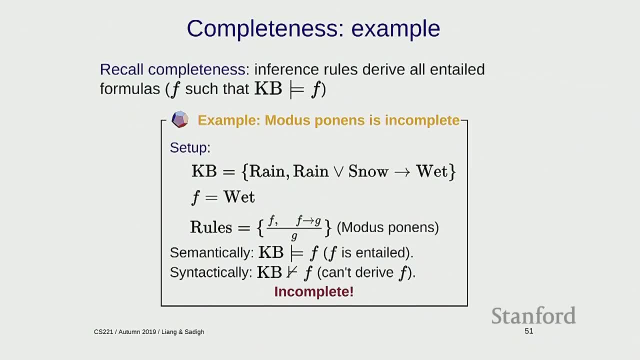 Um question. Yeah For the notation. when it says kv equals rain, then comma rain or snow yields what Is it implying? any type of assignment to rain there, Like is it saying that it is raining or is it just saying that we have variable rain? 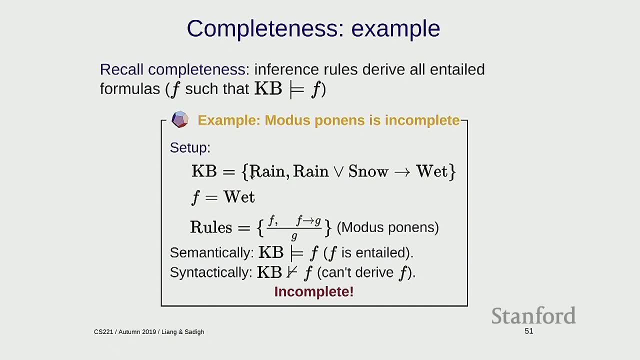 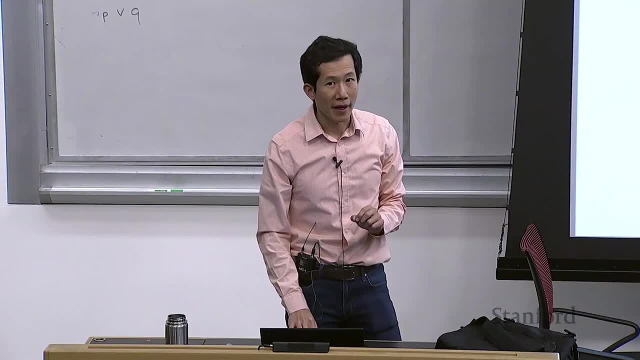 Yeah. So the question is: what does this mean? Um, this- so the knowledge base is a set of uh formulas, So in this particular formula is rain, And remember the models of a knowledge base is where the formulas are true. 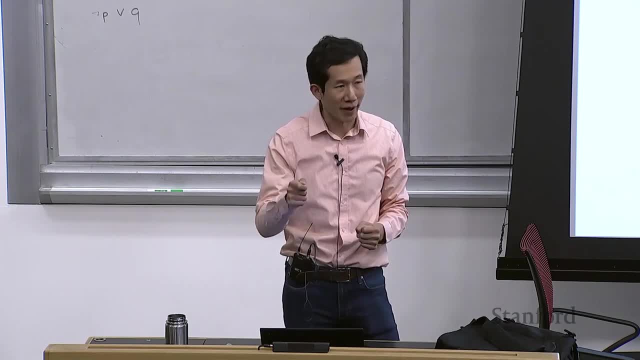 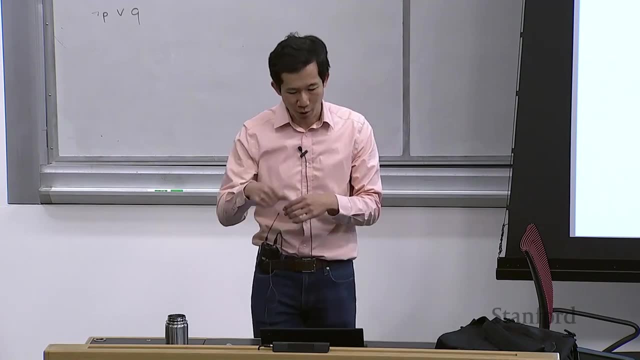 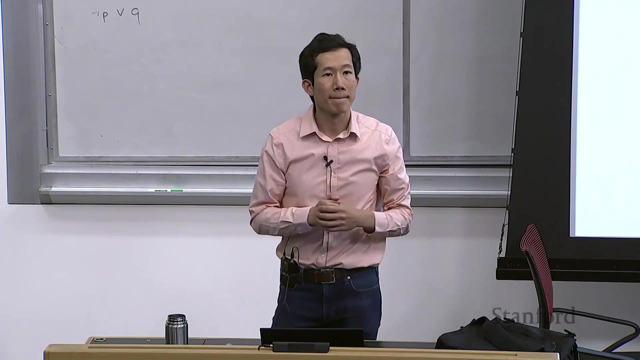 So yes, in this case it does commit to rain being one. It- the models of kv are only include the um- the models where rain is one. Otherwise this formula would be false. Yeah, Probability of a model um. 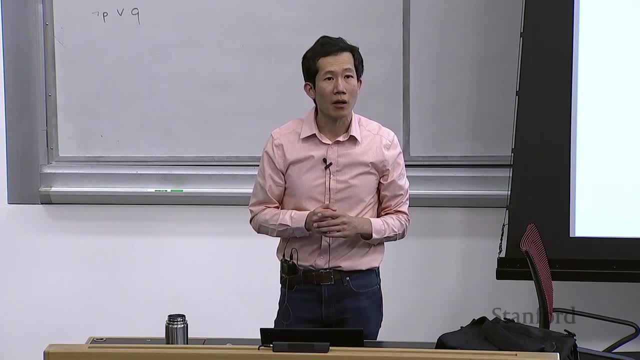 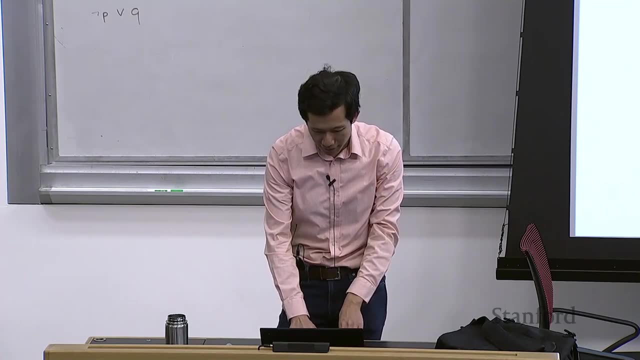 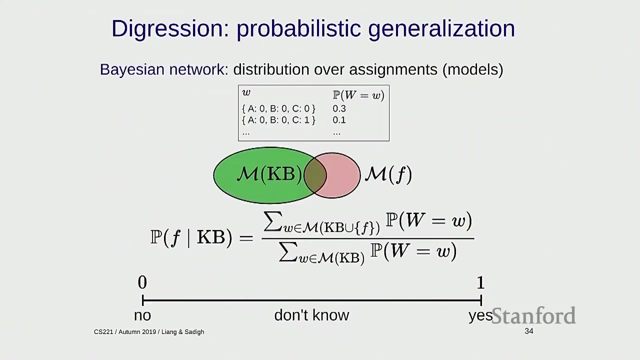 as in way back before the- Oh it was. how can we have a probability over a model? Um, so remember that a model is um. where did it go? Okay, So remember a model. here is just an assignment to a set of. 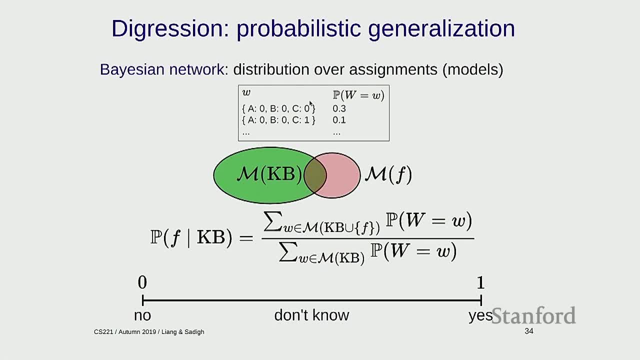 uh, propositional symbols or variables, right? So when we talk about Bayesian networks, um, we're defining a distribution over assignments to all the variables. So here what I'm saying is that assume there is some distribution over um complete assignments to random variables and I could use that to compute. 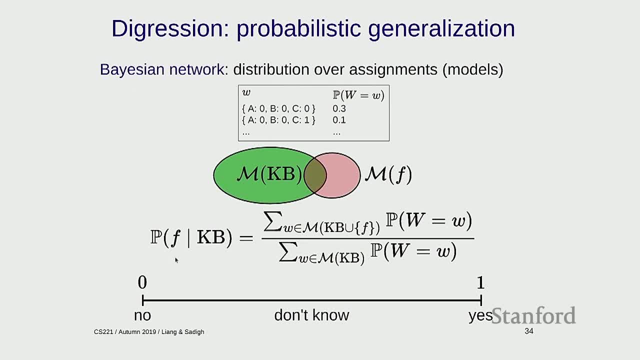 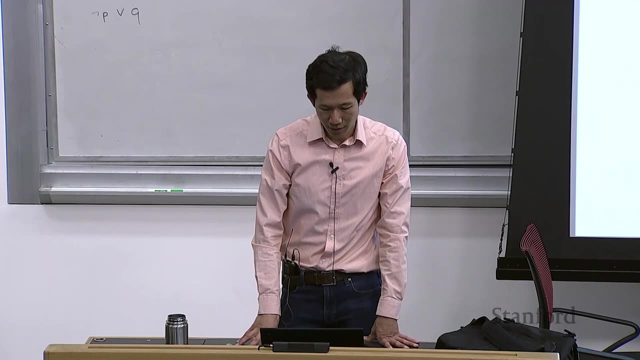 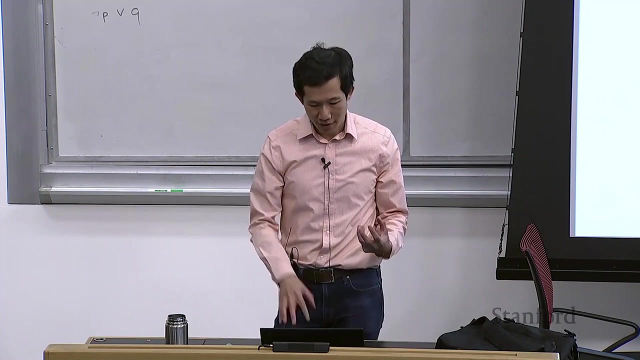 um problem: probabilistic queries of the form of formula given knowledge base. Am I answering your question? They can't be in the same knowledge base. Um, if you have two models that uh, or formulas that contradict, then this intersection is going to be uh zero. 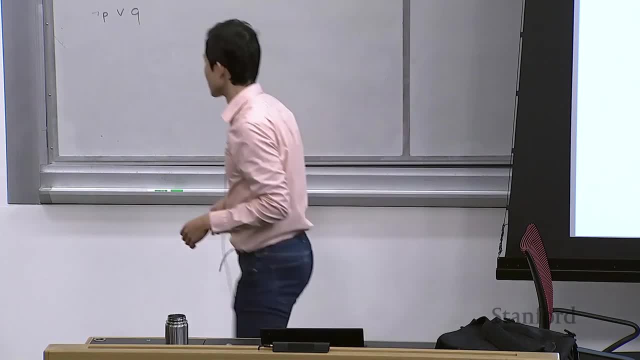 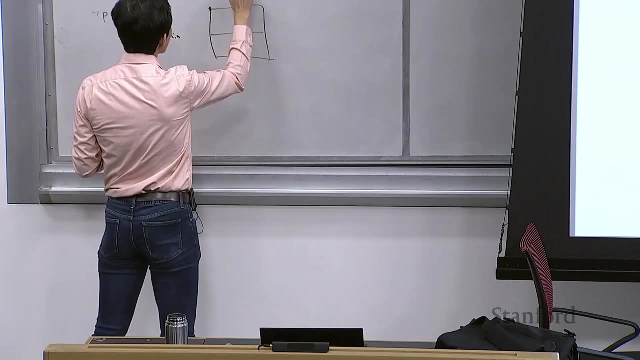 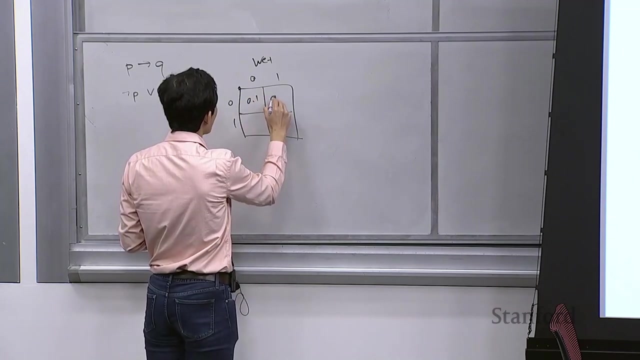 So there is, exists a set of models, So let me do it. um you know this way. So imagine you have these two variables, rain and wet. Um a Bayesian network might assign a probability 0.1, 0.. um I should make these sum to 1,. 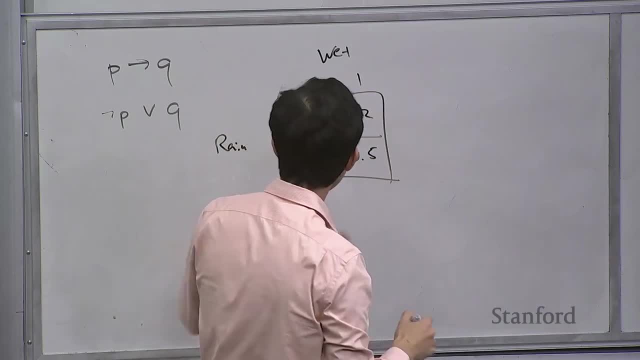 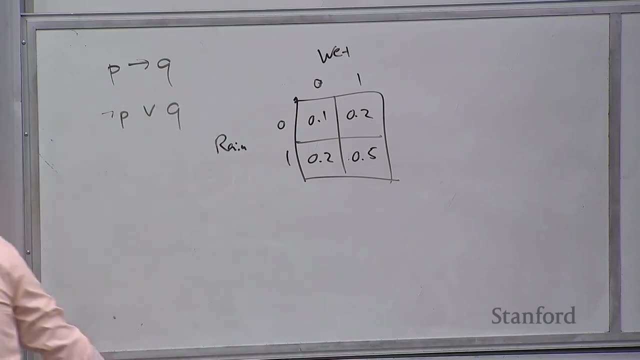 um 0.. what is this? 5. Um, so some distribution over these states, right And um? and if I have rain that corresponds to these models, so I can write: the probability of rain is 0.2 plus 0.5 to 0.7, okay. 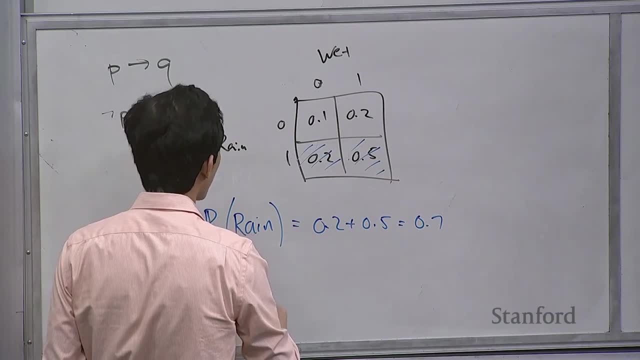 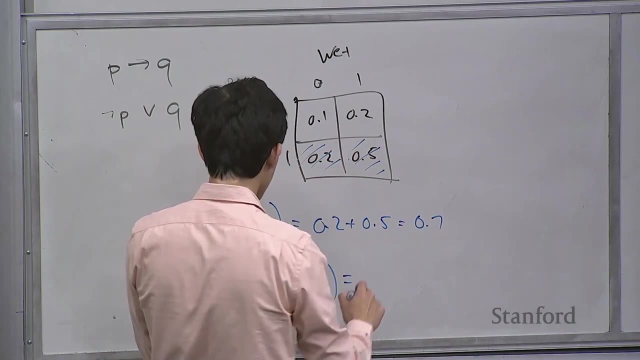 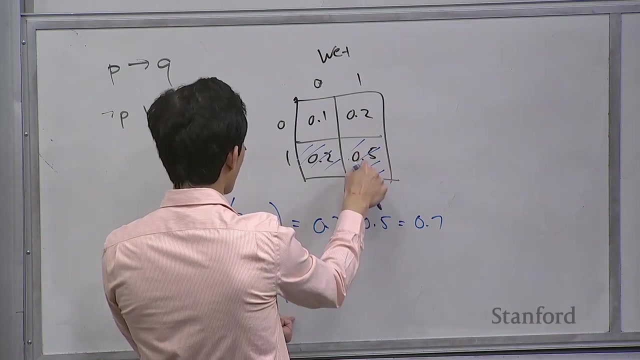 And if I have the probability of wet, um given rain, um, this is going to be the probability of the conjunction of these, which is going to be wet and rain, which is here, which is going to be 0.5 divided by the probability of rain. 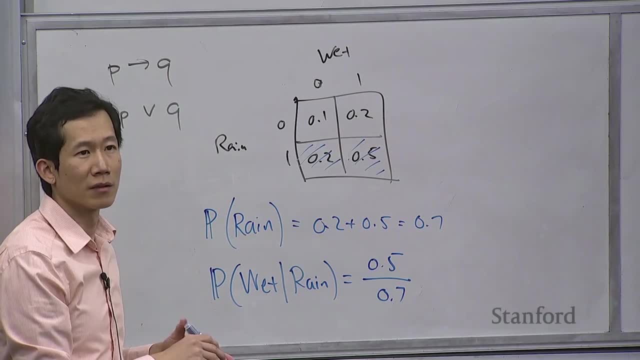 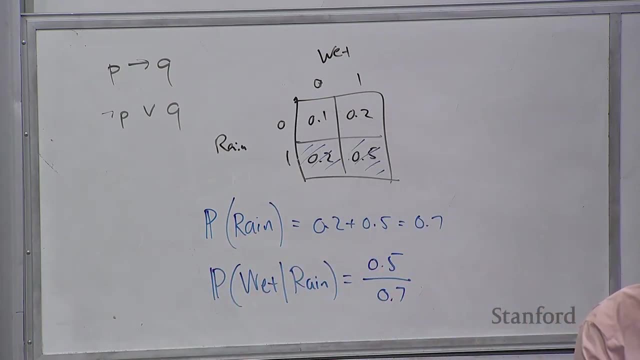 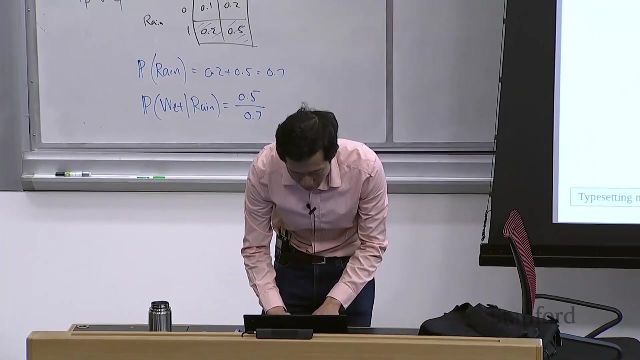 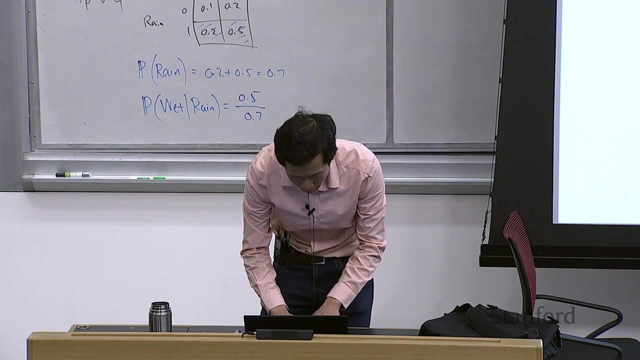 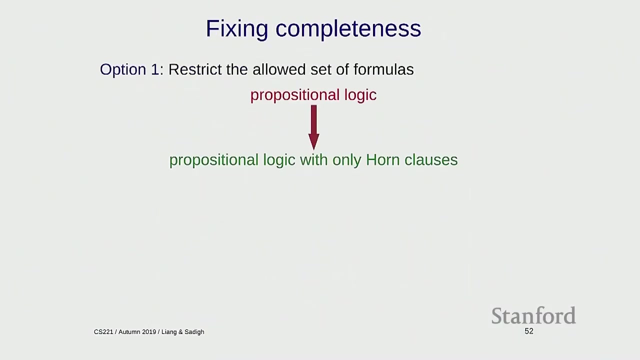 which is 0.7.. Does that help? Okay, Oops, Um, okay, So, okay. so modus ponens is sound, but it's not complete. So there's two things we can do about this. We can either say: propositional logic is too fancy. 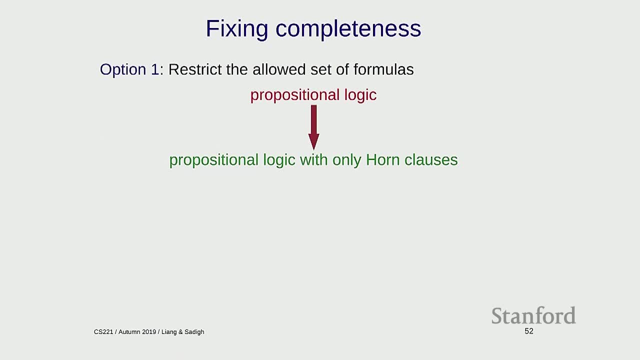 let's just restrict it so that modus ponens becomes complete with with respect to a restricted set of formulas, or we can use more powerful inference rules. So today we're going to restrict propositional logic, Um, to make it complete. 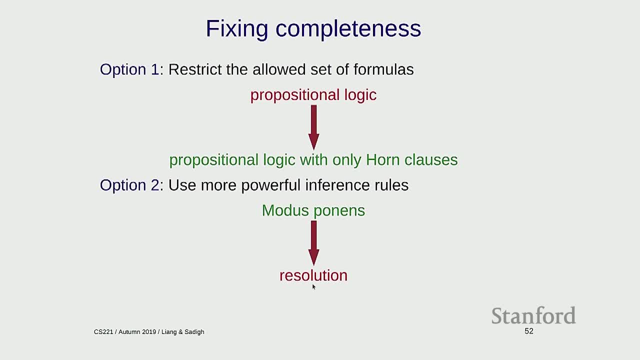 Um, and then next time, we're going to show how a resolution, which is, uh, even more powerful inference rule, can be used to make, um, any arbitrary inferences. And this is what's uh powering the- the system that I showed you. 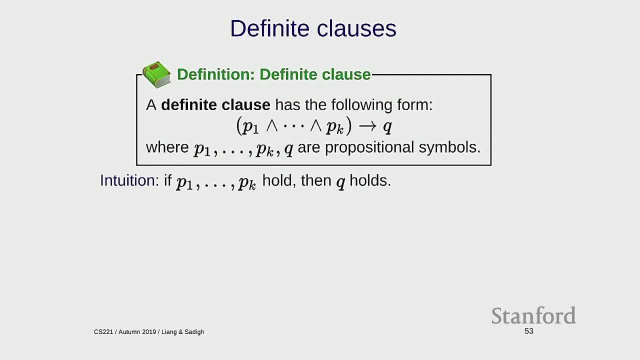 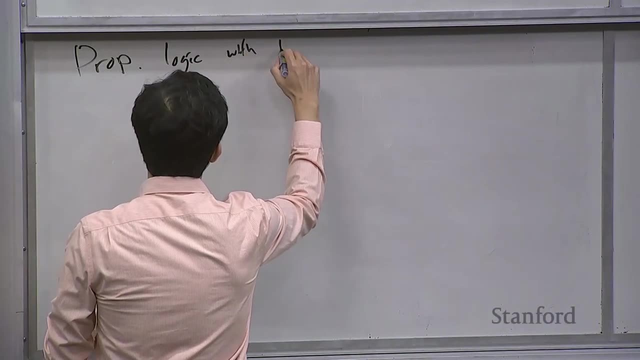 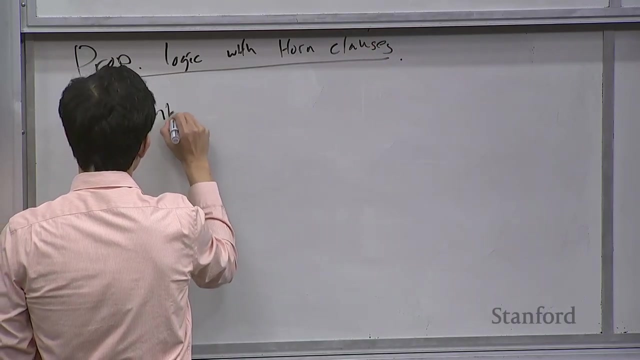 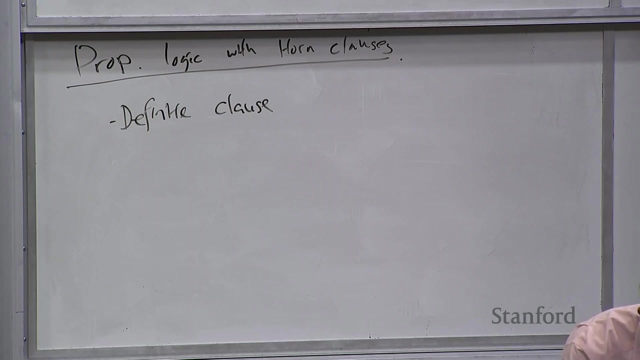 Okay So, um a few more definitions. So we're going to, uh, we're going to- define um propositional logic with with horn clauses, Okay So. so a definite clause is um a propositional formula of the following form: 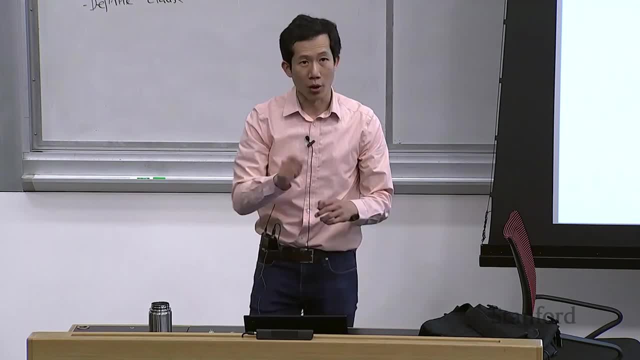 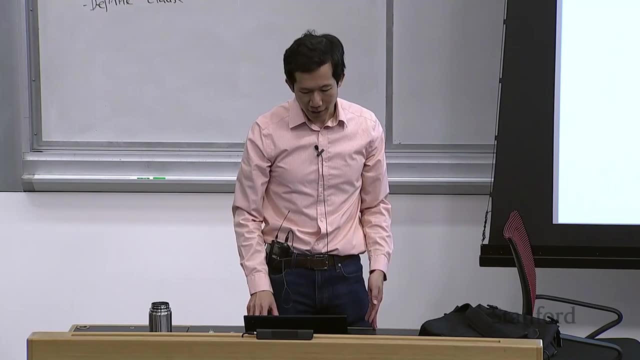 So you have some propositional symbols all conjoined together. Conjoined just means it's added. um implies some other propositional symbol, q, And the intuition of this uh formula says: if P one through p call, k hold. 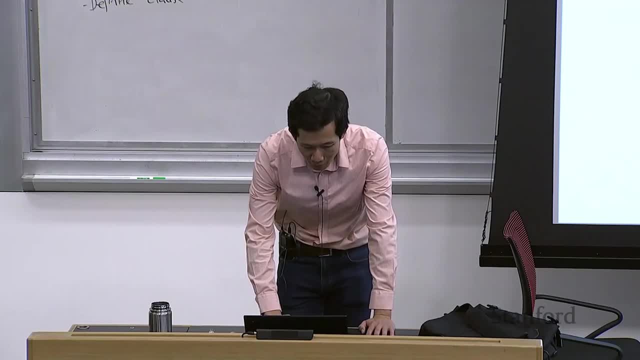 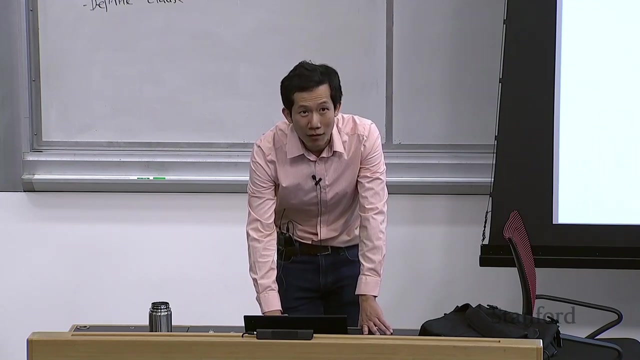 then q cut also holds. So here's some examples: Rain and snow implies traffic. Um, traffic is- can be- is possible. Um, this is a, not an example. um, this is a valid propositional uh logic formula. 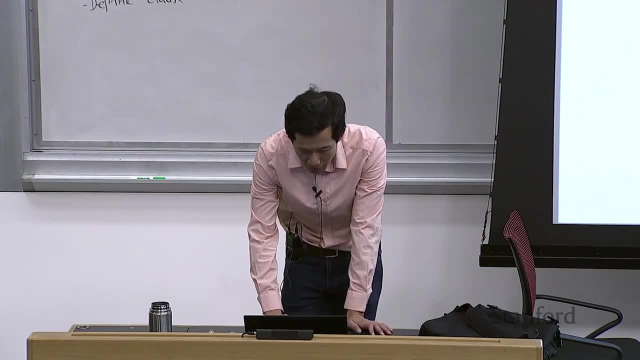 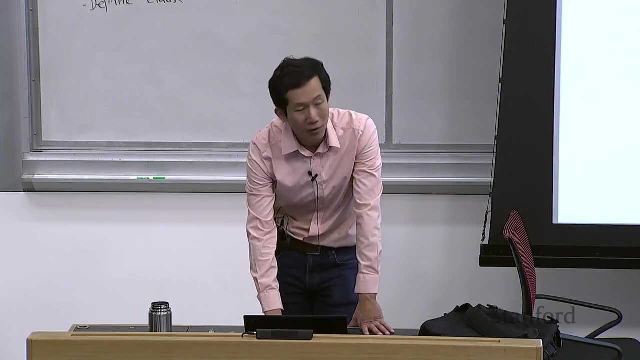 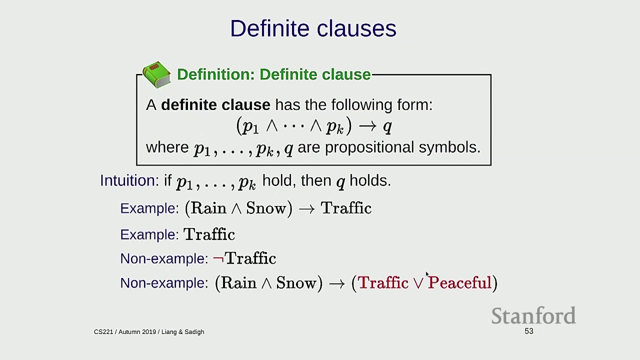 but it's not a valid definite clause. Um, here's, uh. Here's also another example: um, rain and snow implies peace. uh, traffic or peaceful, Okay. So this is not allowed. because only thing allowed on the right hand- hand side. 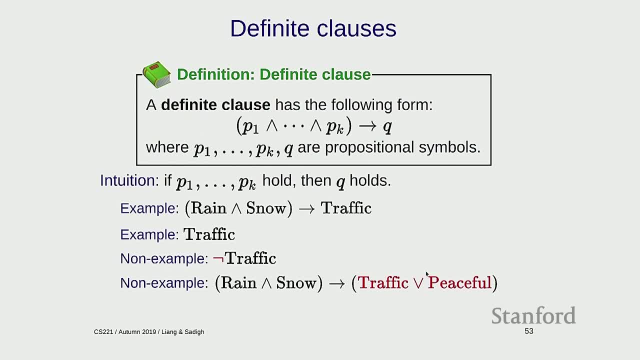 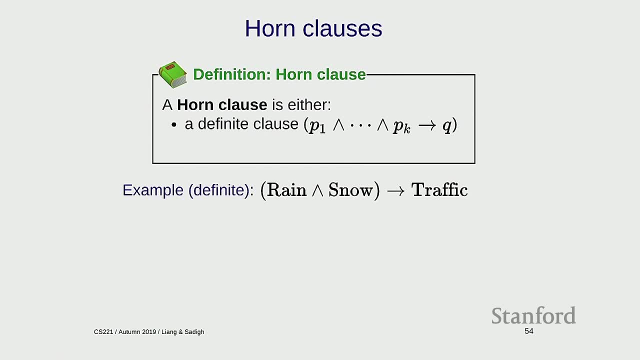 of um. the implication is a single propositional symbol and there's two things over here. Okay, So a Horn Clause is um a definite clause or a goal clause, um, which might seem a little bit mysterious, but um, it's defined as a. 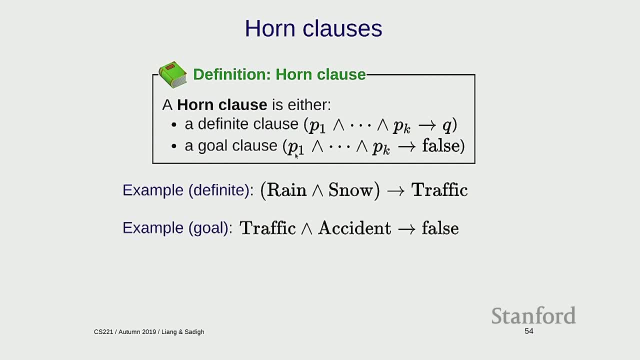 um something that um P1 through Pk implies false, And the way to think about this is the negation of a conjunction of things. right, Because, remember, um P implies Q is not P or Q, So this would be not P or true. 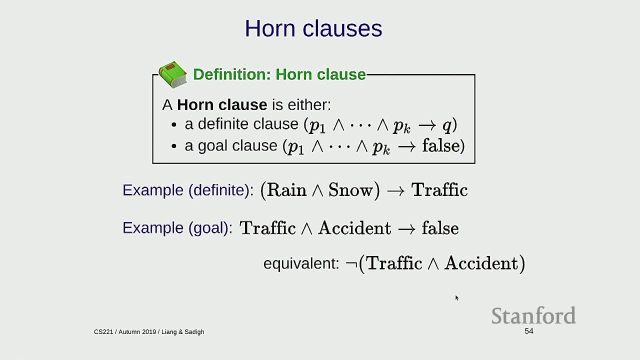 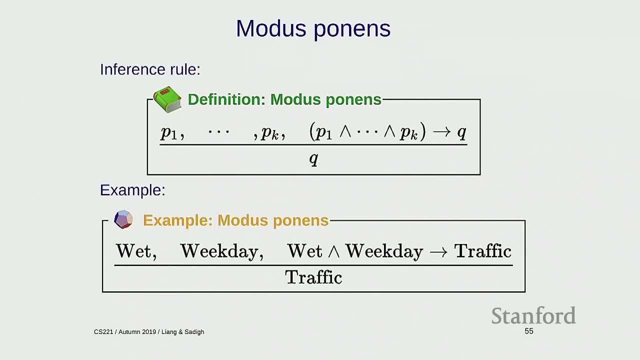 which is not P in this case. Okay, So. so now we have these Horn Clauses, Um. now remember the inference rule: modus ponens, Um. we are gonna slightly generalize this to include um, not just P implies. 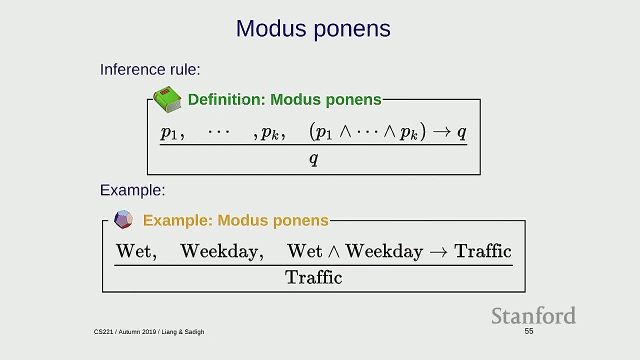 Q, but P1 through Pk implies Q, So you get to match on um premises which include formulas which are atomic propositional symbols and a rule that um looks like this and you can uh derive or prove uh Q from that. 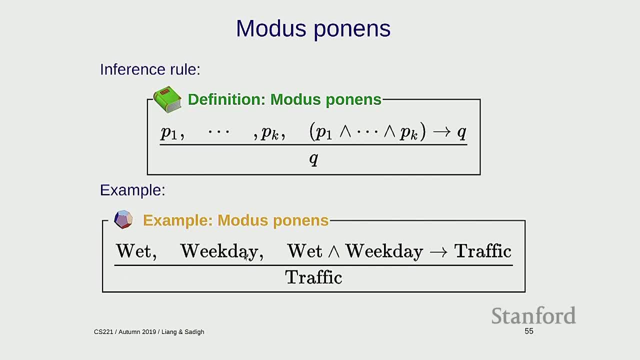 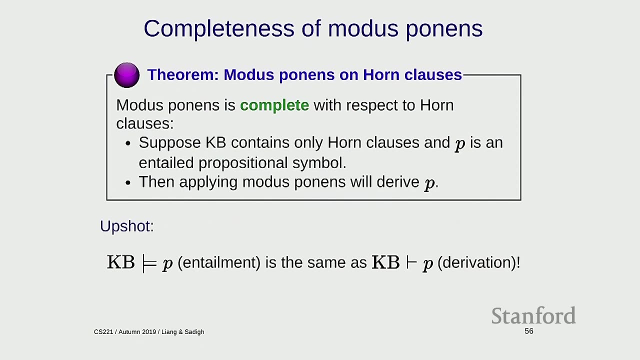 Okay. So, as an example, wet and weekday- if you see wet weekday, wet and weekday implies traffic, those three formulas, then you can- you're able- to add traffic, Okay So, um. so here's the claim. 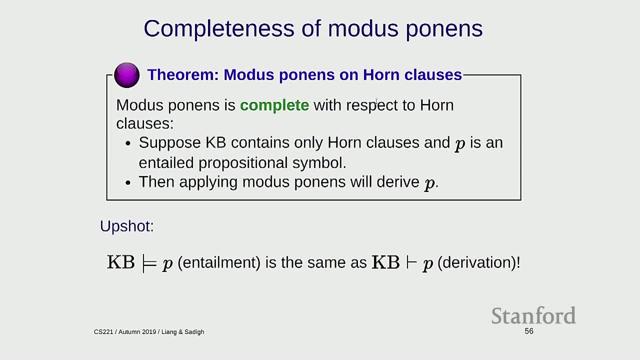 So modus ponens is complete with respect to Horn Clauses for propositional logic. So, in other words, what this means is that suppose that the knowledge base contains only Horn Clauses and that um P is some entailed uh propositional, uh symbol. 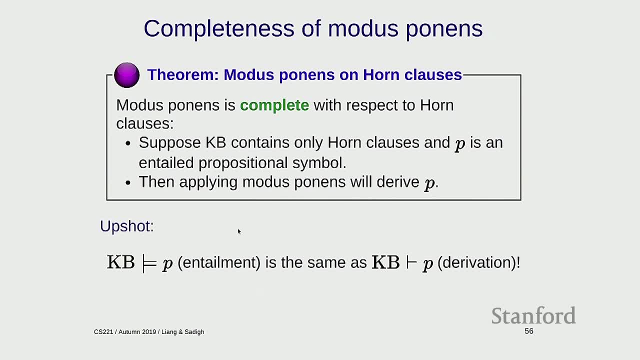 By the entailed propositional symbol. I mean like kB actually entails P. snatically, Then applying modus ponens will derive: P means that the two relations are equivalent and you can celebrate it because you have both soundness and, uh, completeness. 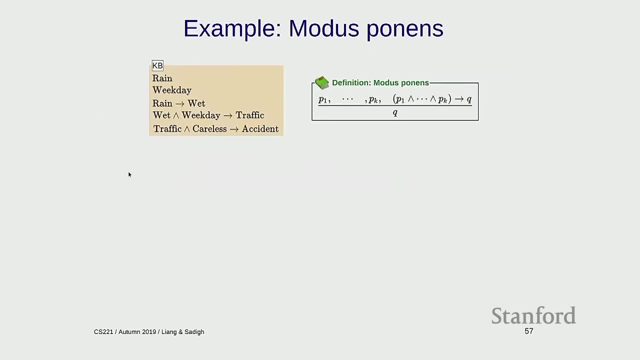 Okay, So just a quick example of this: Um. so here, imagine, is your knowledge base, um and uh, so the base is so many different things. So, versus exponential randomization, you know this equation that I just did, and if I do this, 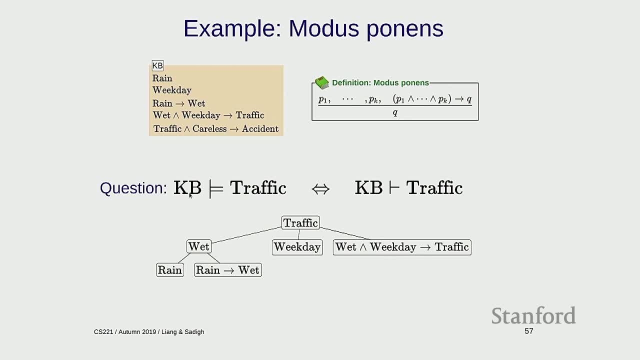 okay, so I can multiply it for, and that's the result, And that's the Commonwealth. I wrote the convolutional operation of Liszt. you're asking the question: uh, is there traffic? And remember, because, um, this is a set of only horn clauses. 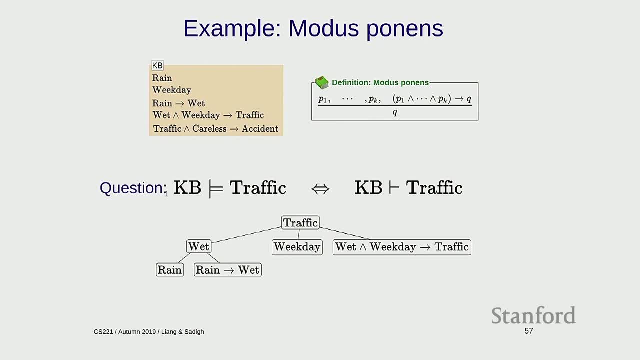 and we're using modus ponens, which is complete. That means um entailment is the same as being able to derive it using these rules, this particular rule, um, and you would do it in the following way: So rain, rain implies wet. 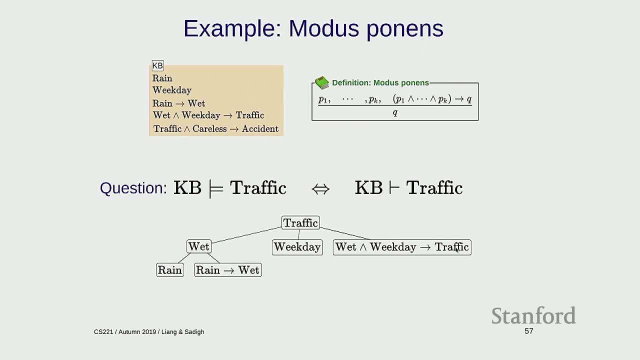 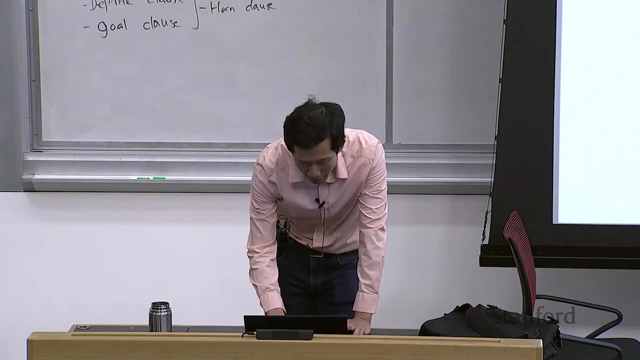 gives you wet, wet, weekday, wet and weekday implies traffic, gives you traffic and then you're done. Yeah to um like rain and weekday. why are those horn clauses? Uh, the question is, why are rain and weekday horn clauses? 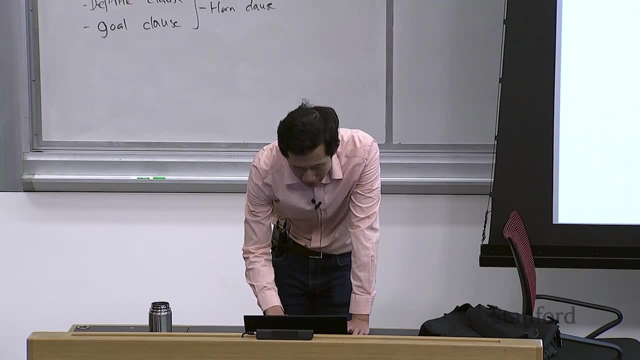 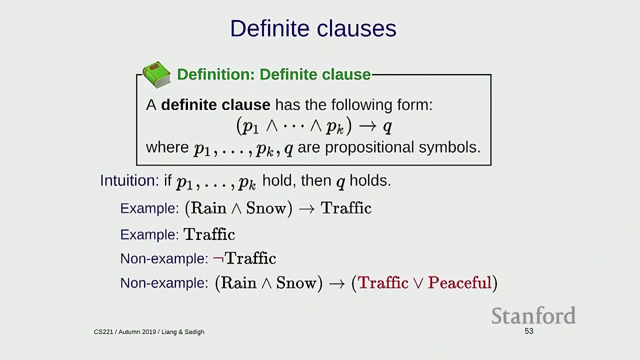 So if you look at the definition of horn clauses, they're definite clauses. If you look at the definite, they should have definite clauses. they look like this: and um k can be 0 here, Which means that um. 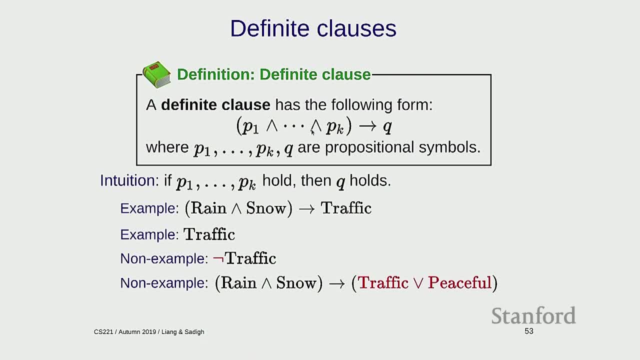 there's um, there's kind of like nothing there. Does that make sense? It's a little bit of a- I'm using this notation, kind of um, to exploit this corner case that if you have the and of 0 things. 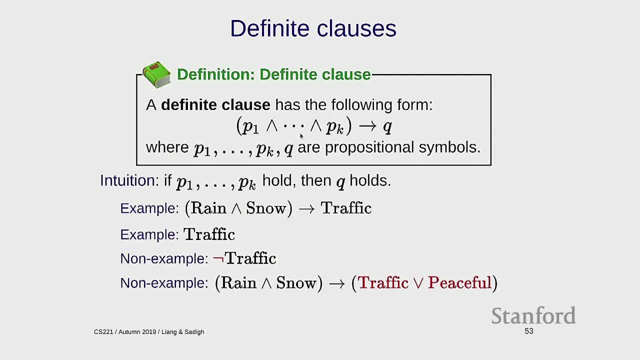 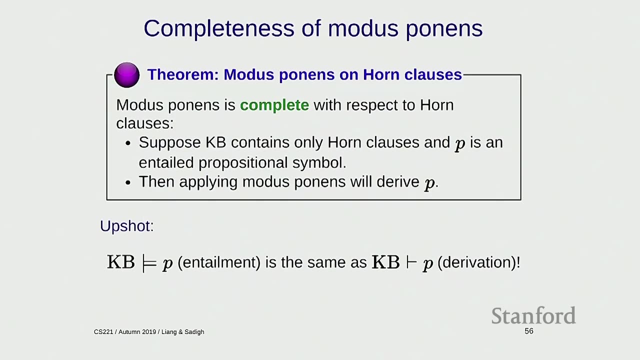 then that's just um, you know true. Or you can just say: by definition, definite clauses contain propositional symbols. um, that will do too, Okay. So let me try to give you some intuition. why modus ponens and horn clauses? 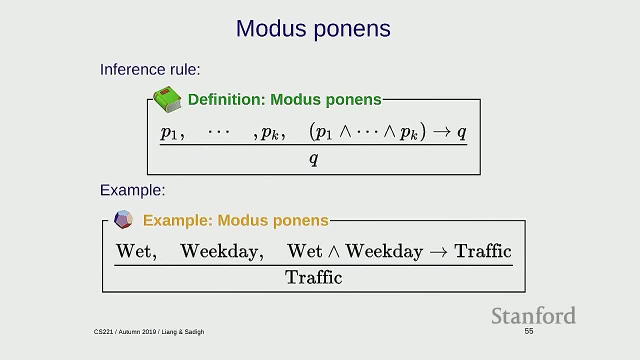 So the way you can think about um modus ponens is that it only works with positive- uh- information. in some sense, There's no branching either, or It's like every time you see this, you just definitively declare q to be true. 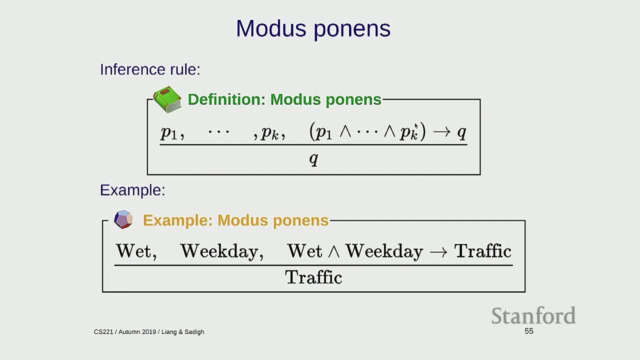 So in your knowledge base, you're just gonna build up all these propositional symbols that you know are going to be true, And the only way you can add a new propositional symbol ever is by, uh, matching a set of other things which you definitely know to be true. 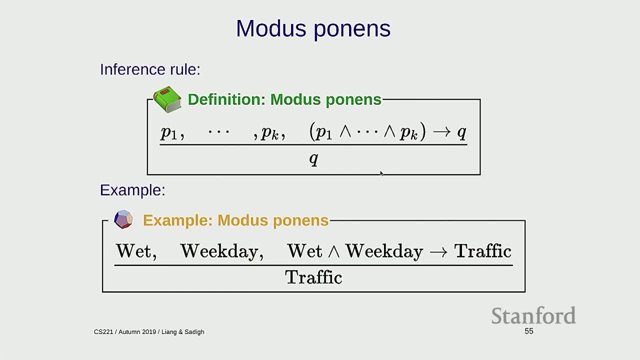 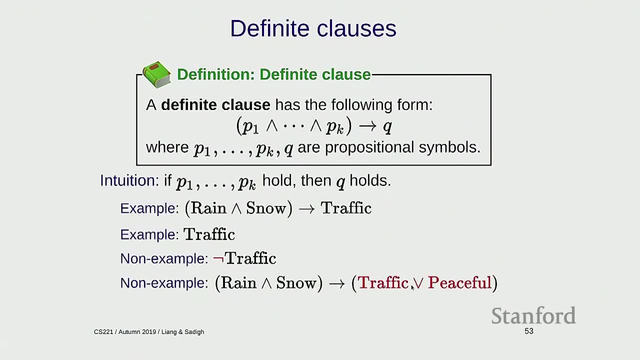 and some rule that tells you q should be true and then you make q true. um, add q to your knowledge base as well. The problem with propositional symbols, uh, more general clauses, is: if you look at this, rain and snow implies traffic or peaceful. 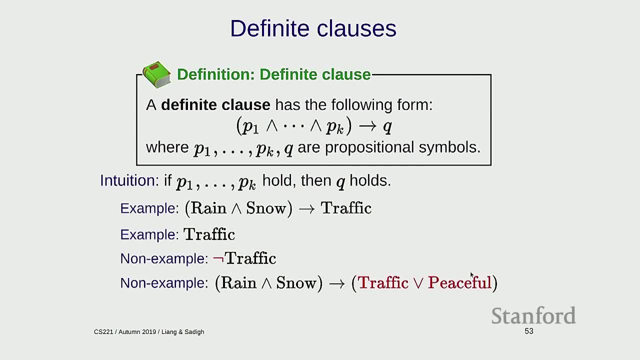 you can't just write down traffic, or or peaceful, or both of them You have to reason about. well, it could be either one, and that um is outside the scope of what modus you know ponens can do. Yeah. 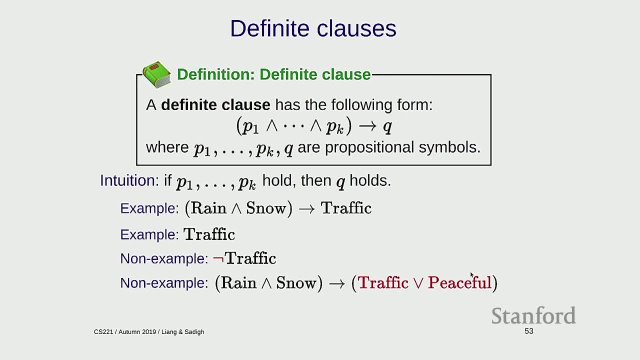 And peaceful, not what you can say like, okay, those two are true, so those both have to be true. Yeah, yeah, Good, good question. So what if it happens? if it were traffic and peaceful? Um, so this is an interesting case where technically it's not a definite clause. 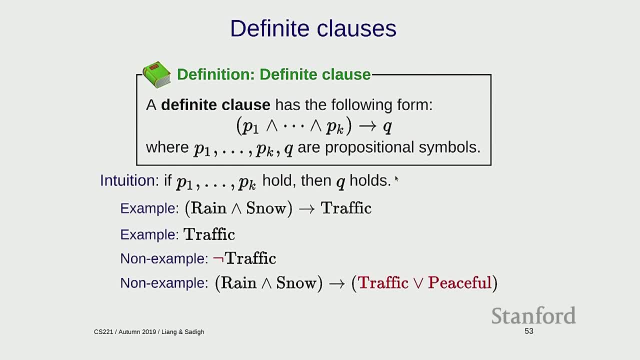 but it essentially is: Um, so I'm- there's a few subtleties here. So if you have A implies B and C, you can rewrite that This is exactly the same as having two formulas: A implies B and A implies C. 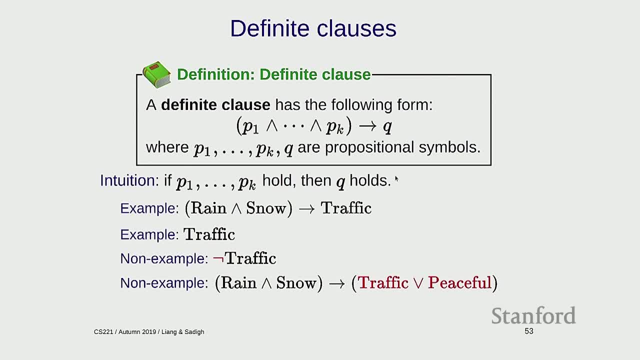 and these are definite clauses. Um, just like you know, technically, if I gave you, hey, what about A? not A or B? It's not a definite clause by the definition, but you can rewrite that as um. A implies B, So there is.